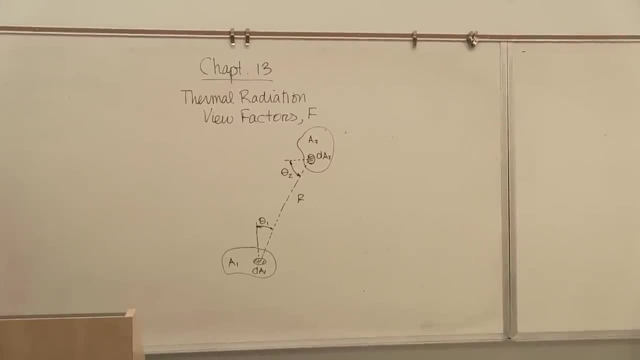 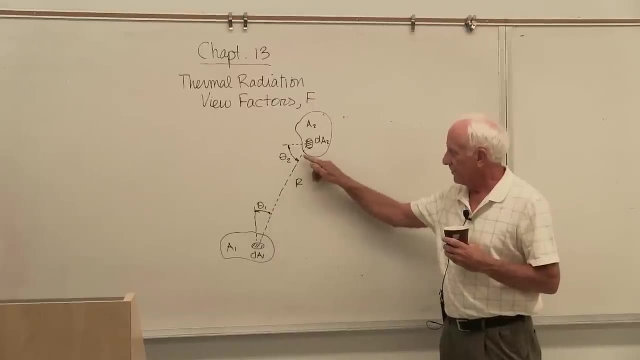 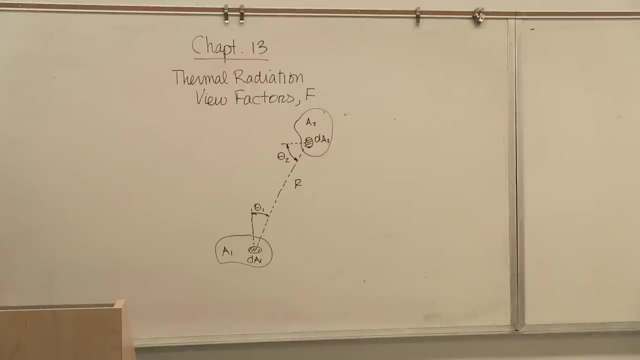 And the angles of A1 and DA1 and DA2 with respect to their normals, going to the distance R, theta 1, this angle, theta 2, this angle from the normal to the line labeled R. Now, to do that, to find that energy between A1 and A2,. 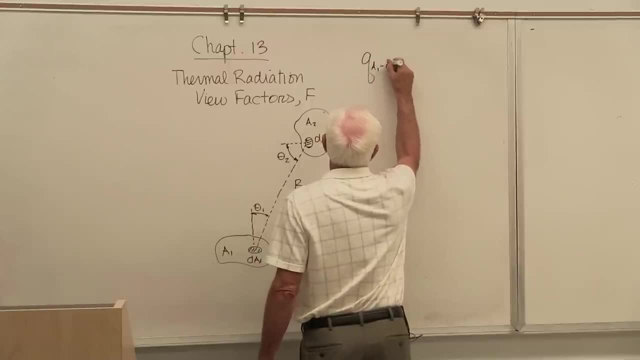 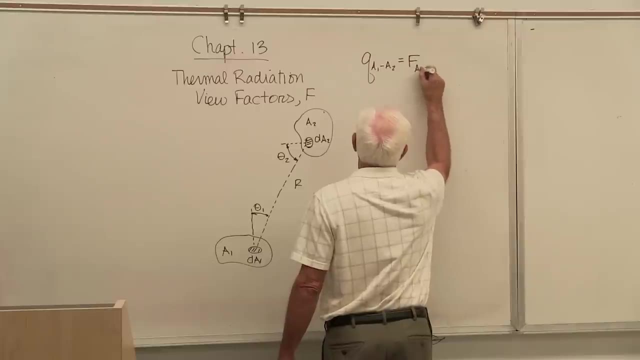 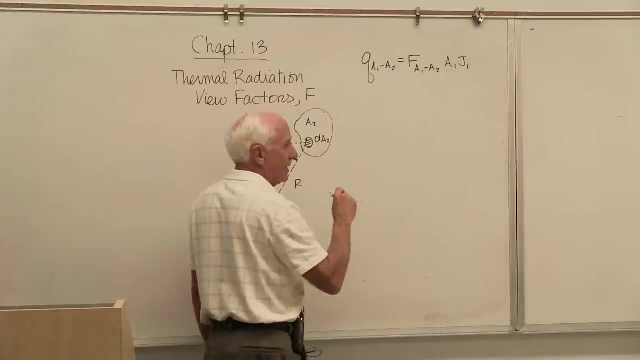 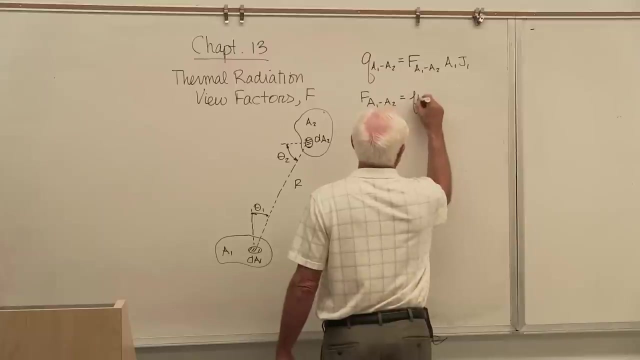 we can say that Q from A1 going to A2 is equal to the view factor from A1 to A2, which is equal to the clean energy from the A1 and the J1.. Now I'm going to define F. A1 to A2 is a fraction of energy. 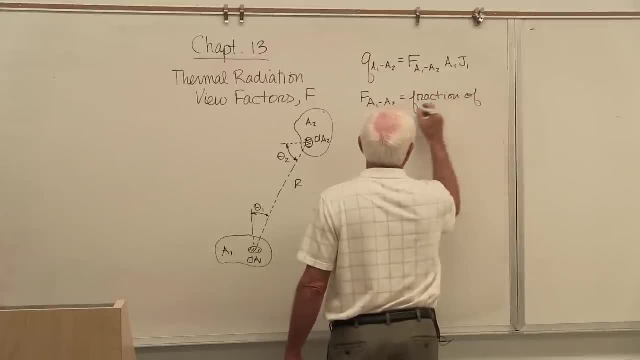 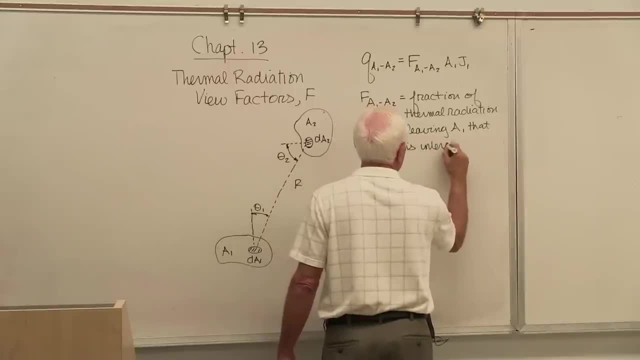 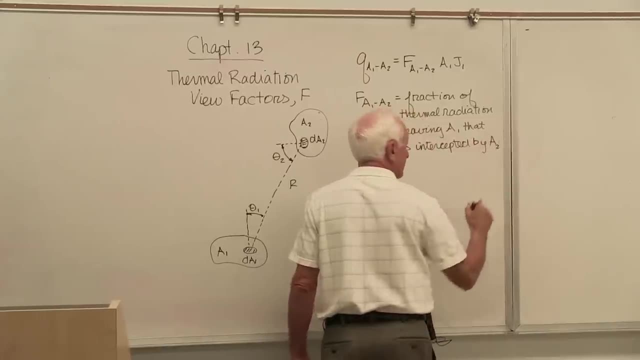 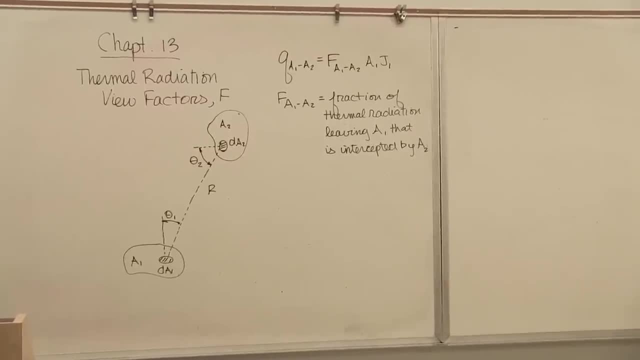 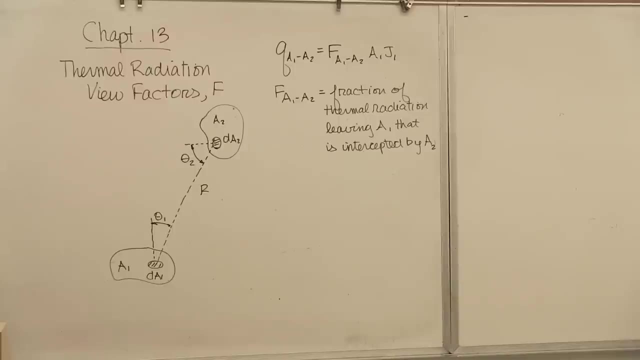 But that's the fraction of the total energy leaving A1, the thermal radiation energy that ends up getting to surface, A2.. You can say it's intercepted by, received by strikes by. They all mean the same thing, Maybe if F, if F, A1 to A2 is 0.10,. 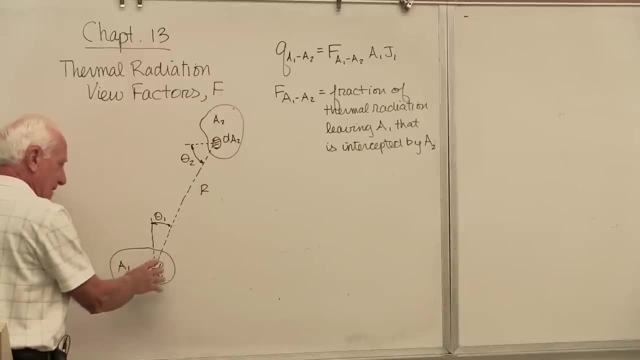 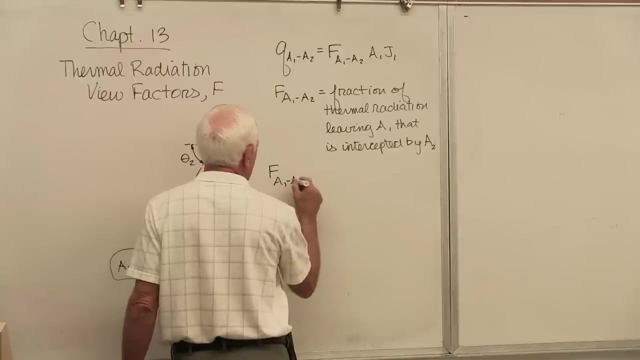 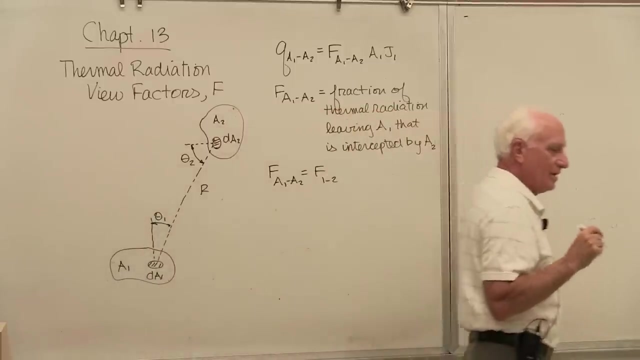 that means 10% of the thermal radiation leaving surface A1 ends up at surface A2, 10%, 0.10.. We take shorthand notation here rather than F A1, A2.. So F? A1, A2, we call that another shorthand notation, F1-2.. We know that to mean. 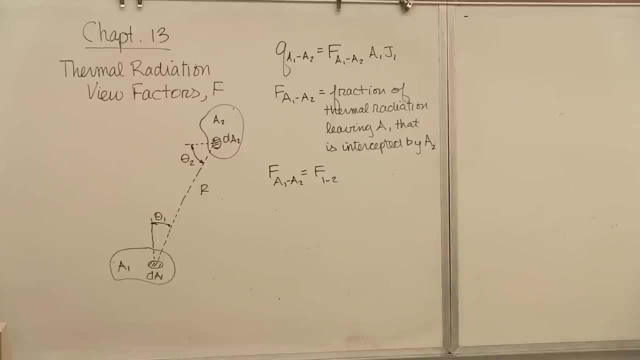 that's the fraction going from surface A1 to surface A2.. We even simplify that further. We don't like the dash, so we just say F12.. That's not F12.. Don't say F12.. That's F12.. It means the fraction going from A1 to A2.. So we can rewrite this expression for. 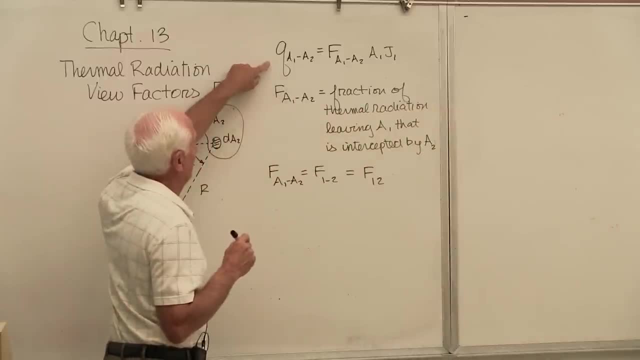 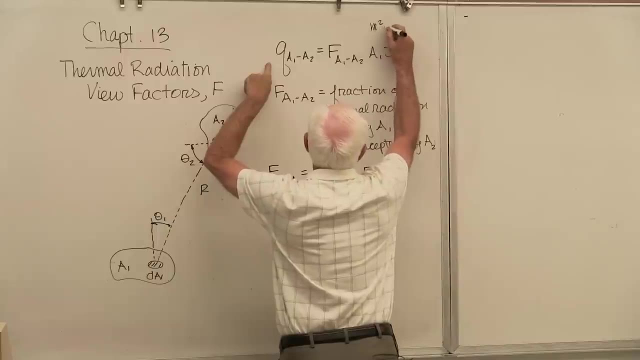 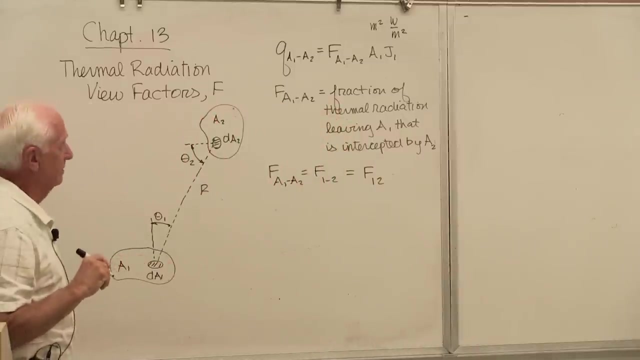 what's Q? Q is the amount of radiation in watts. in watts, Just so you know, A1 is meters square, J1 is watts per square meter and F is a fraction and fractions are dimensionless. So Q's in watts, That's the number of watts leaving. 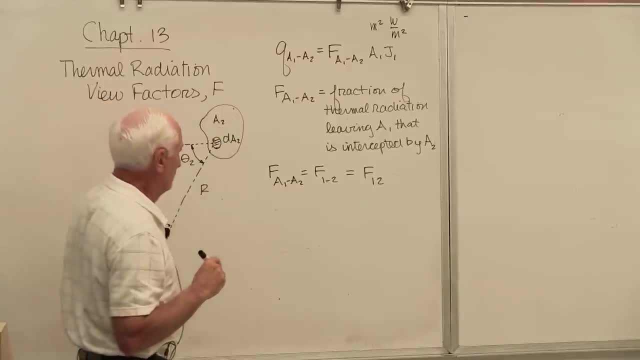 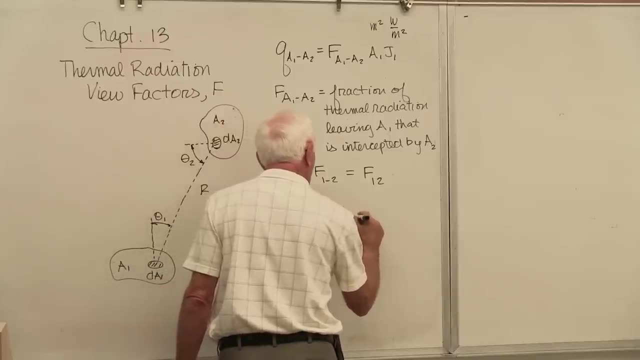 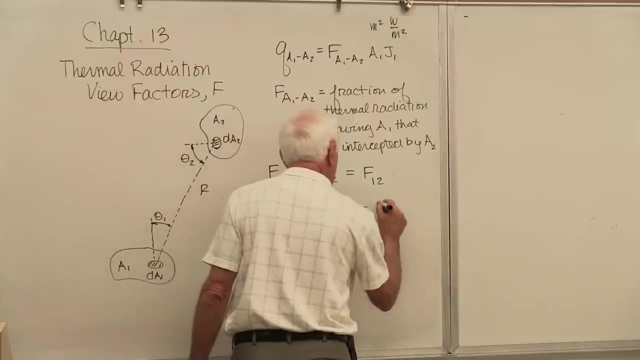 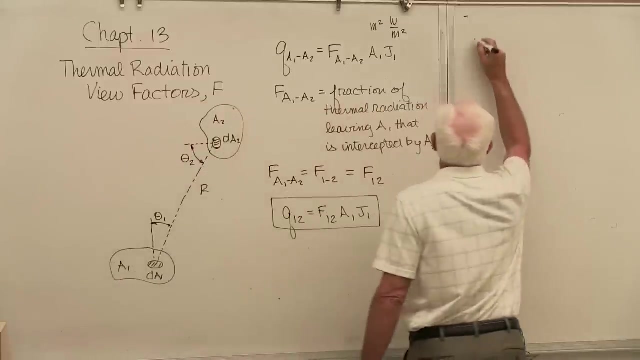 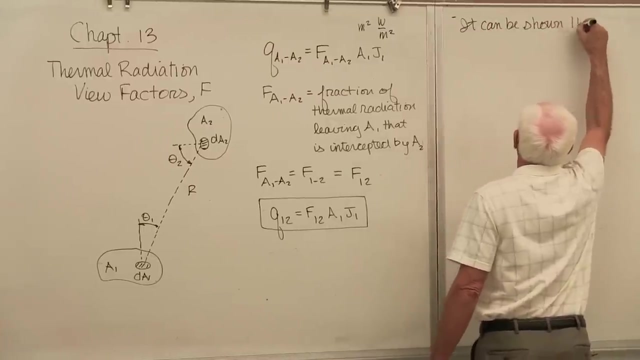 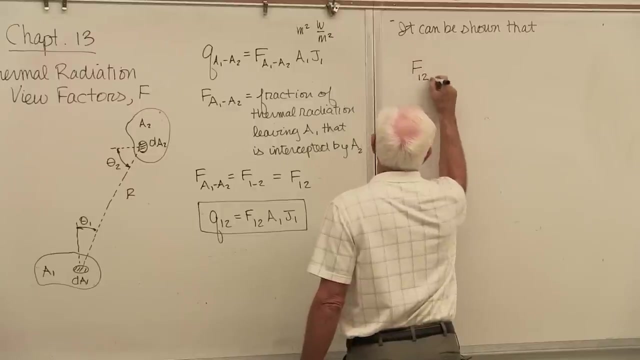 going from surface A1, going to surface A2.. So now the new equation is: Q12 equal F12, A1, F12, J1.. All right, So that's our equation there. Now, officially, the definition of F12 is this mathematical definition: 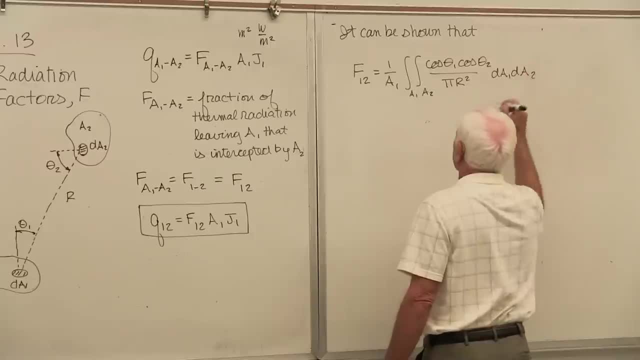 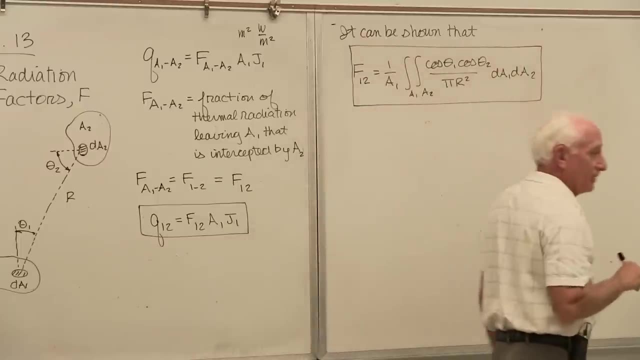 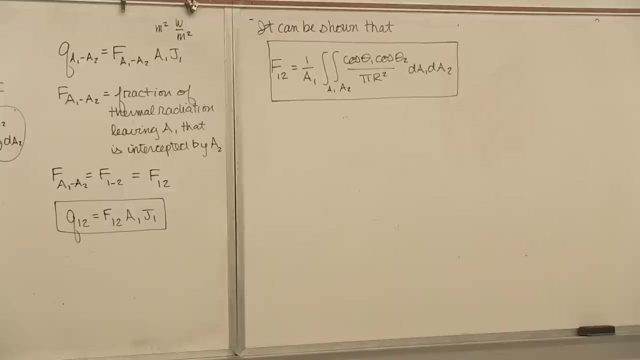 So let's see, And that is mathematically, how we define F12.. It's derived in the textbook, in a whole page of the textbook. We're not going to spend the time to derive that. That's the result of the derivation. 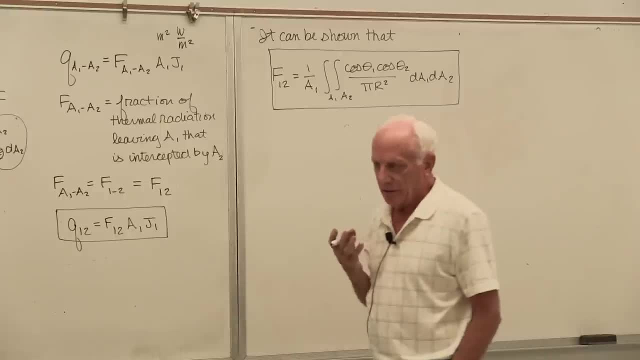 You can see that it's only a function of geometry. The distance are cosine theta 1 and cosine theta 2, dA1 and dA2.. It's only a function of geometry. The view factor F12 is sometimes called the geometric factor because of that reason. 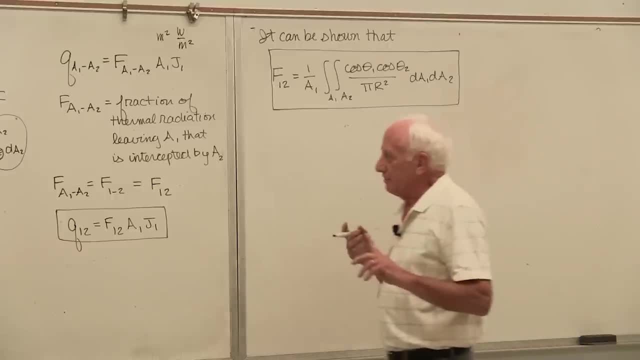 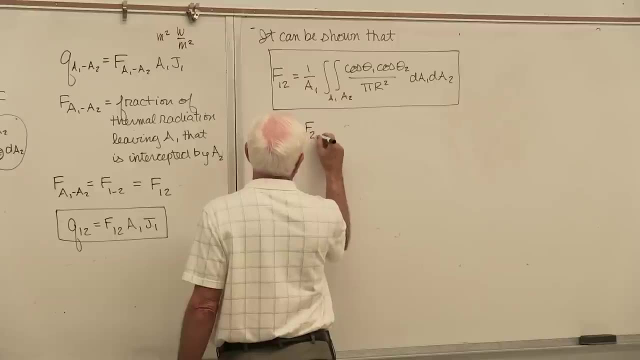 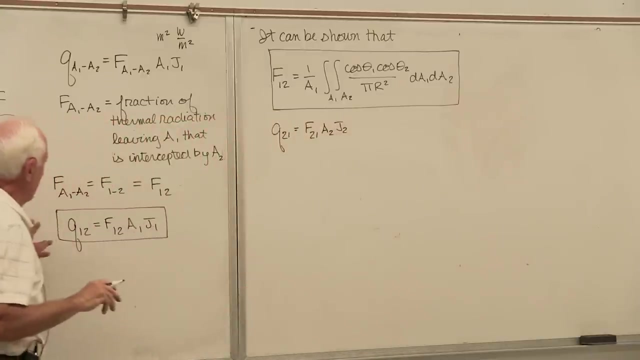 Okay, Now we can play the reverse game: Q from 2 to 1, equal F2 to 1 times A2- J2. That's the fraction of energy leaving surface A2 that is received by or intercepted by A1. That's Q2 to 1.. 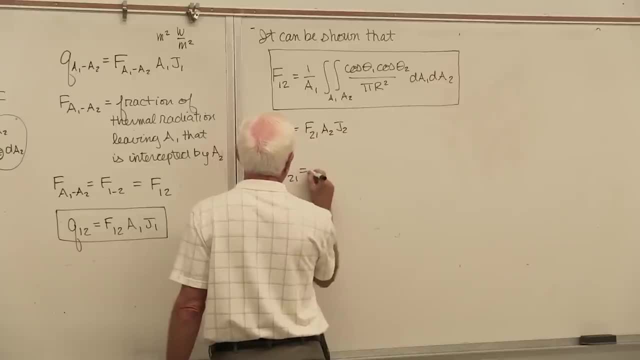 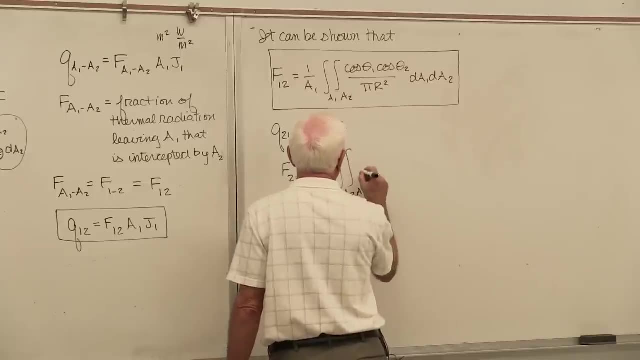 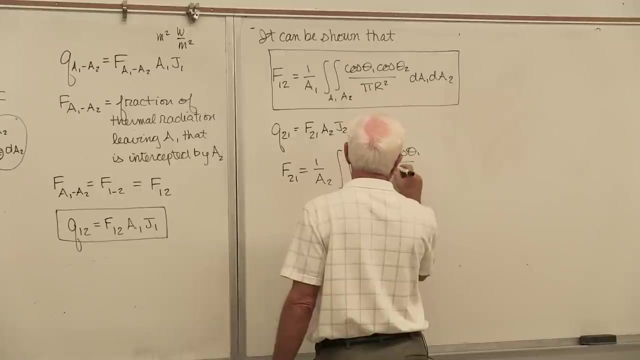 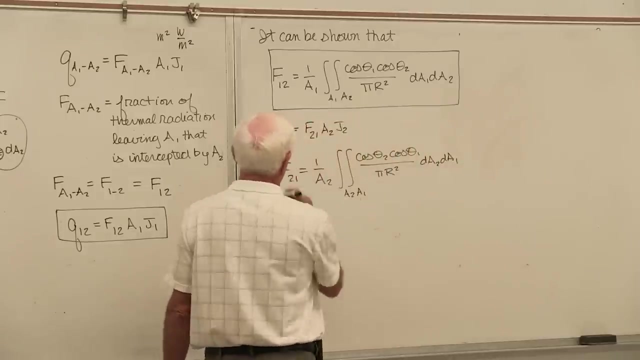 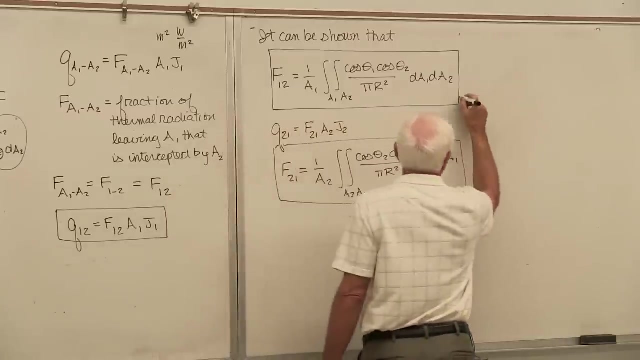 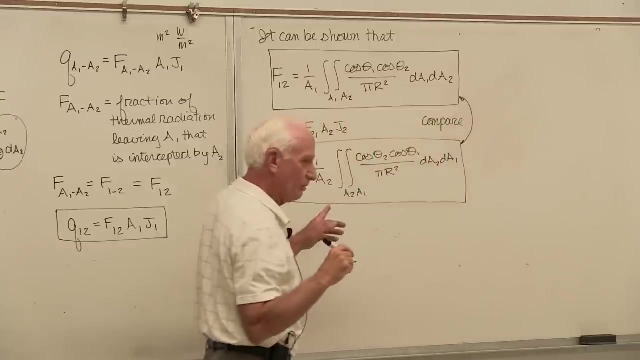 In that equation F2 to 1,, 1 over A2- integral. Okay, Okay, Okay, Okay, Okay. And then you can compare these and draw the conclusion, since the double integrals are identical, don't forget, you can change the order of integration, doesn't matter which. 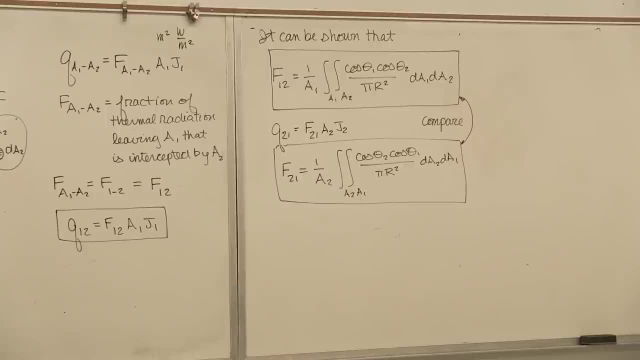 cosign's first theta one or theta two, it doesn't matter which DA's first, DA one or DA two, you can change the order of integration. And so the conclusion is: oh you know what, if I multiply A one times F, one, two, that's. 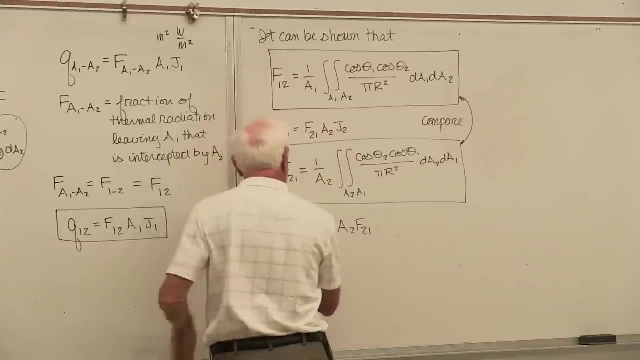 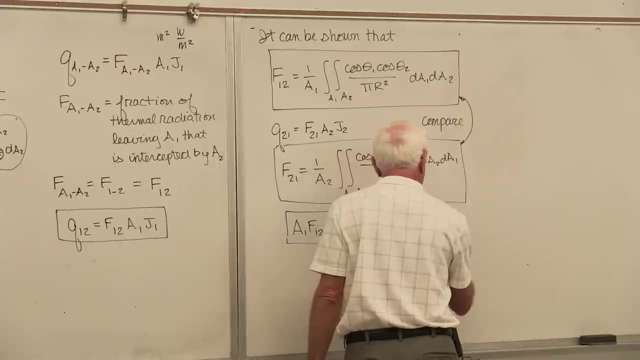 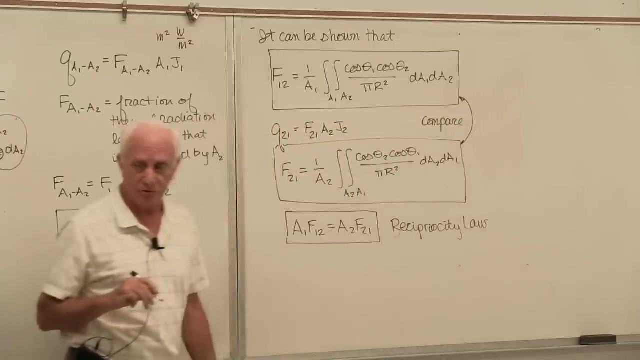 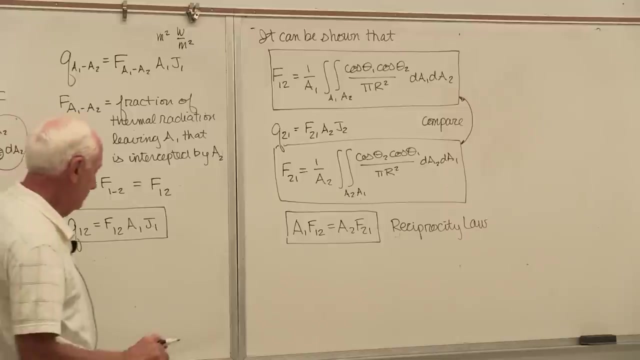 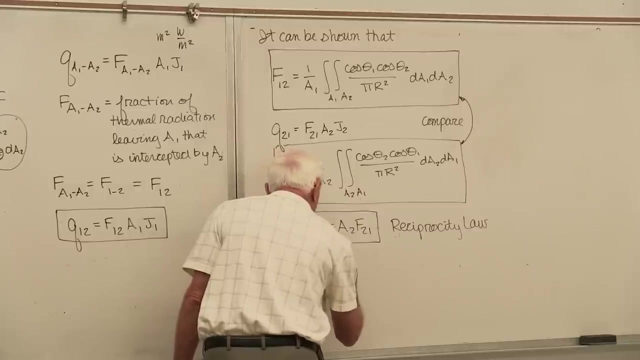 equal to A two, F two one. Okay, there is a very important conclusion called the reciprocity law, which means, if I know one view factor, F one, two, I can easily find F two one by using that equation. Now there's another law, the enclosure law. 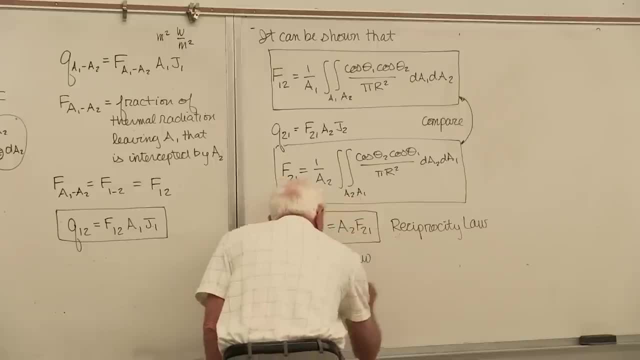 Okay. The general expression is that: Okay, Okay, Okay, Okay, Okay, Okay, Okay. Now, first of all, let's say: it's only valid in an enclosure. So enclosure, For instance. take this room. It's an enclosure. 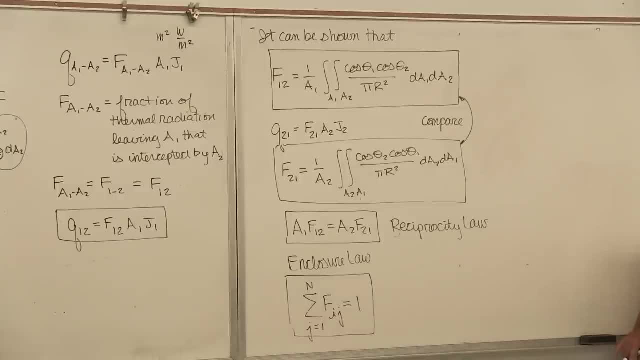 The front wall is one, back wall, two windows, three halls, four floor, five ceiling, six, 6.. This room is a 6 surface enclosure. I'm going to write that for I equal 1.. For each surface, I equal 1 to 6.. So there could be 6 equations. I'll write one of them down. 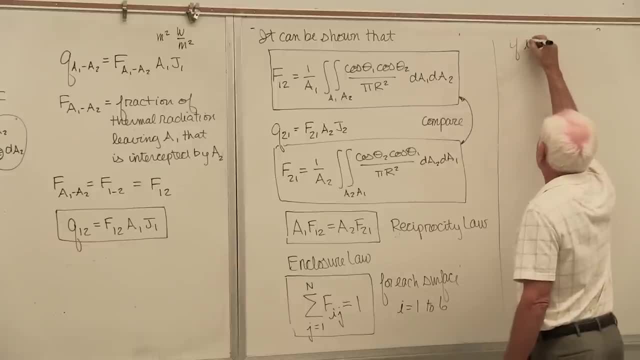 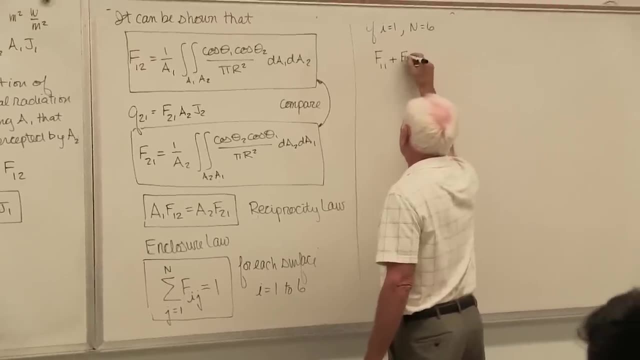 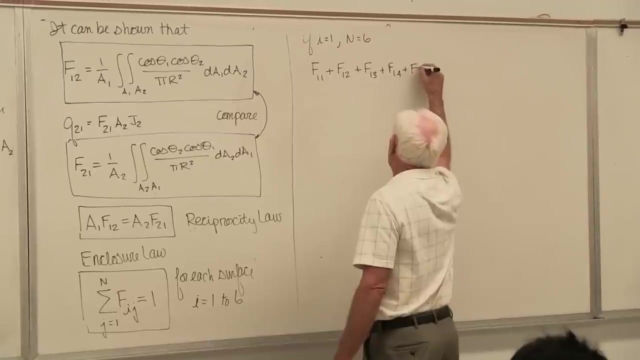 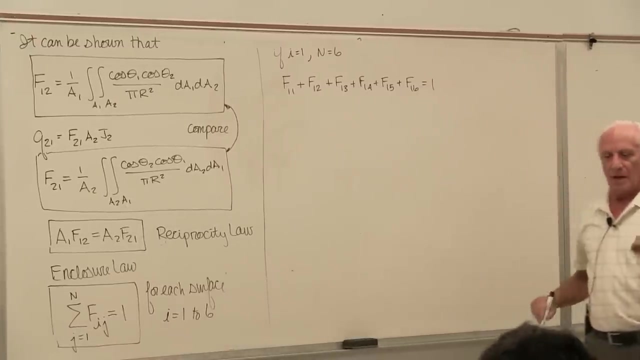 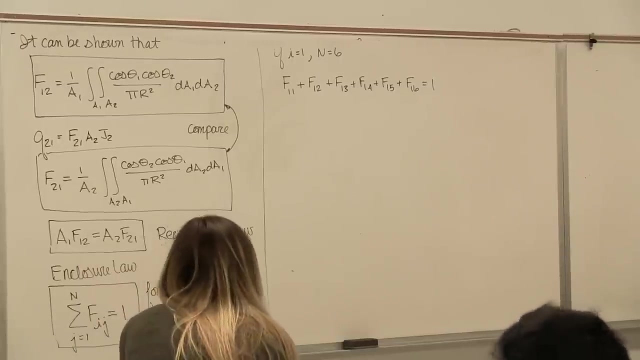 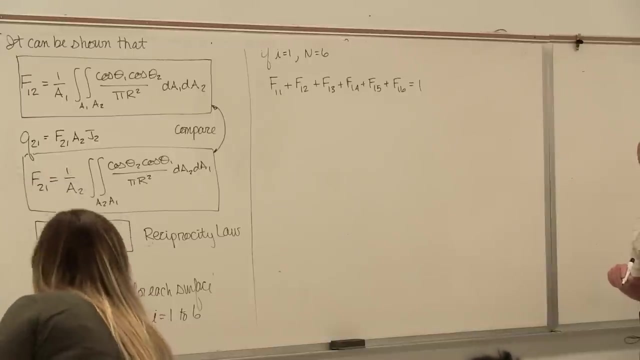 I'm going to let I equal 1.. F11 plus F12 plus F13,, F14,, F15, F16: equal 1.. I can write a similar equation for each of the 6 surfaces in this room: F21 plus F22 plus F23 plus F24 plus F25 plus F26: equal 1, and so on. I'm going to tell you. 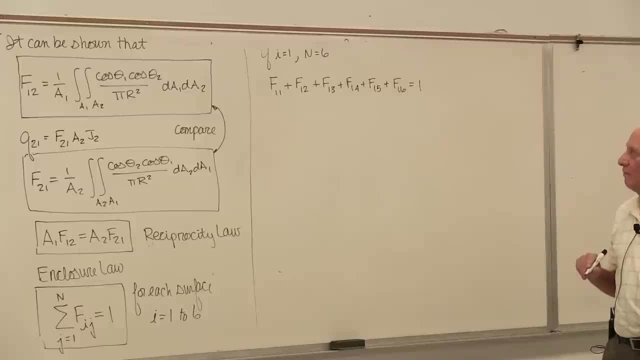 what? F11 is just a minute. okay, Let's just say what is F12.. Okay, I told you, the front wall is 1, the back wall is 2.. F12 is the fraction of thermal radiation leaving the front wall that gets to the back wall. 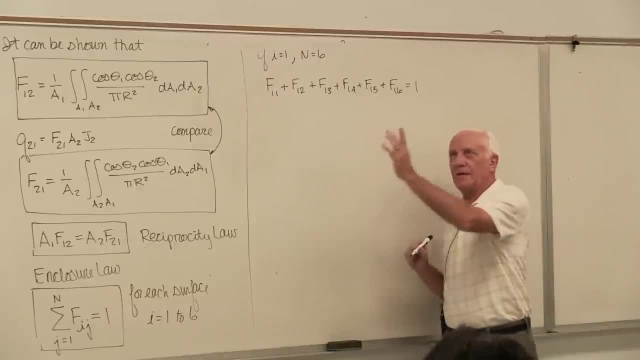 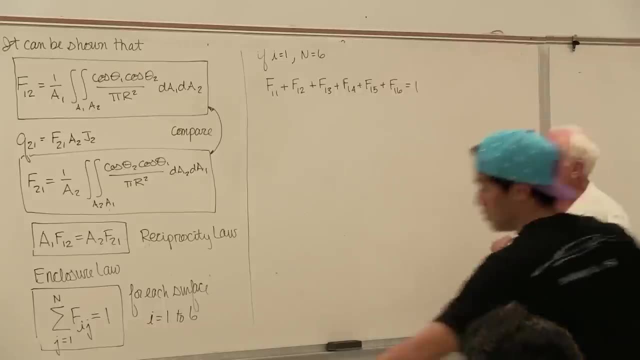 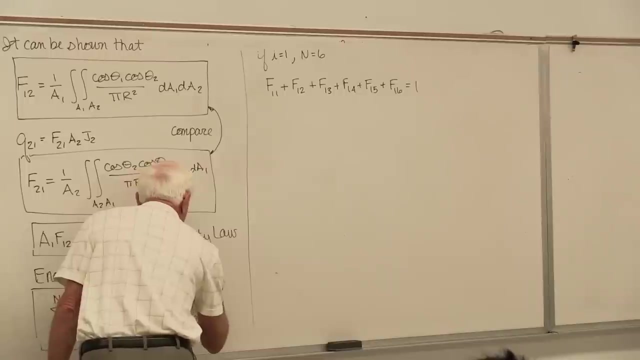 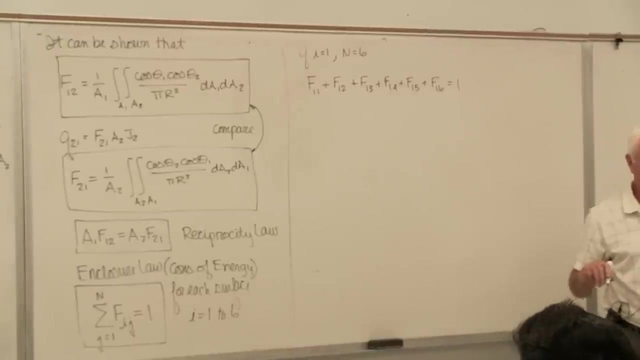 1, 6.. The fraction of energy leaving the front wall that gets to the ceiling wall. 6, A6.. Conservation of energy. okay, Enclosure law is conservation of energy. All the radiation leaving the front wall has to strike another wall in this room and the total must be 100%. 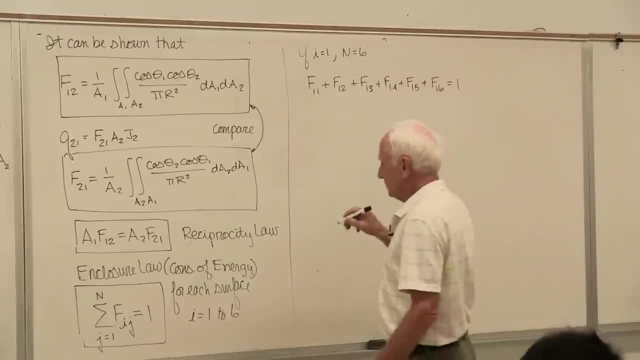 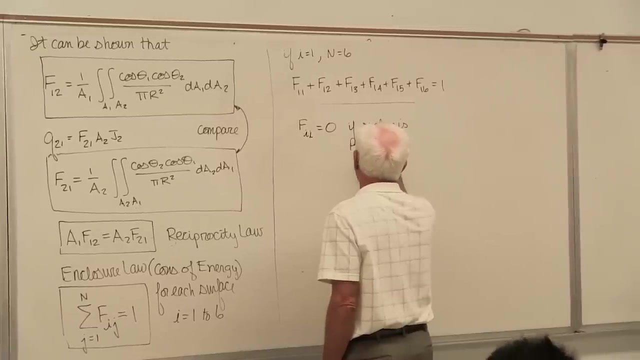 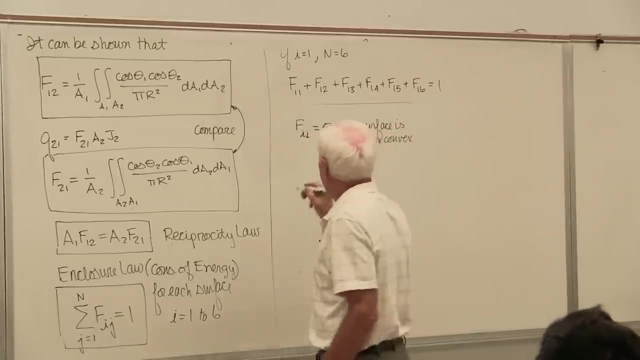 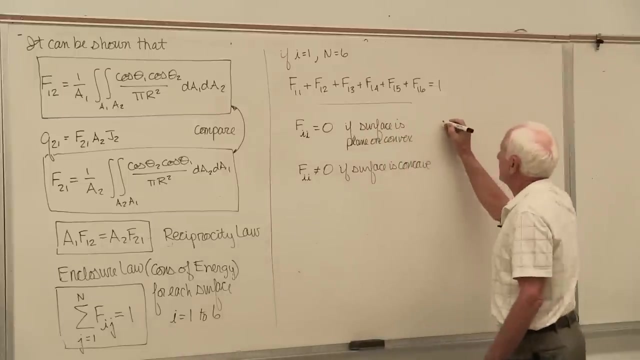 That's what the 1 stands for: 100%. So there's our enclosure law. Now let's talk about FII equals 0 if surface is plain or convex, And then FII is not 0 if surface is concave. Plain surface Radiation leaves the surface we assume. like this: Does any part of the radiation end up striking the plain wall? 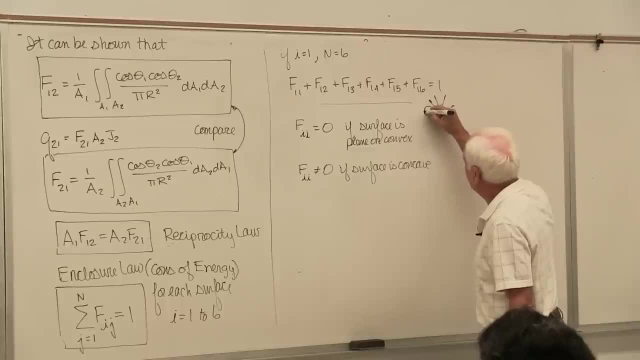 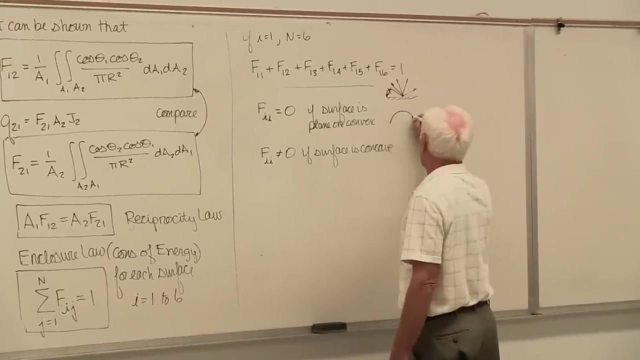 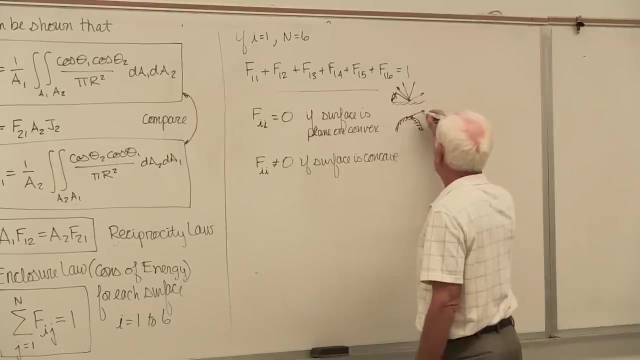 I mean, is that legal? No, that's not going to happen. So any radiation leaving that surface will not hit that surface. okay, Take convex, Take a small differential area up here. Will any of the radiation leaving that surface ever do this? 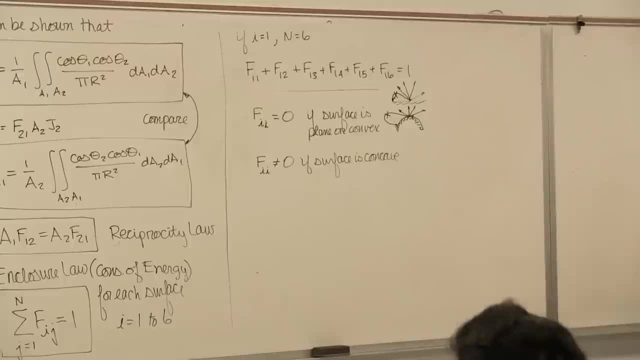 No, that's illegal. Straight lines, straight lines. Conclusion. radiation leaving that surface will never hit that surface. FII is 0.. Concave- small differential area. Radiation leaves the concave area, But Now you can do this to only one entity in our lineup. 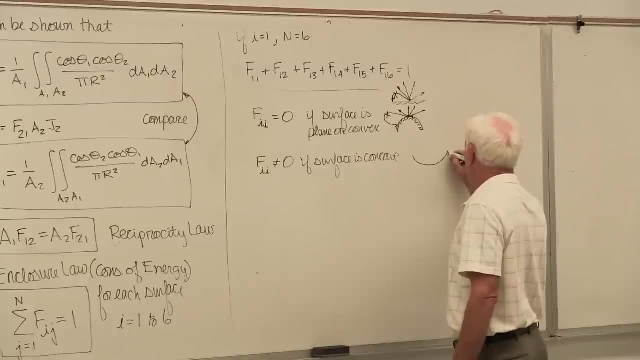 You're in Franconia, you're feasible and you're just three units away, But when I go up into the paling fourth detectors, you never, ever hit a� jewelry. mais I'mast da BRZ-E003ển a6p- grci-ha. 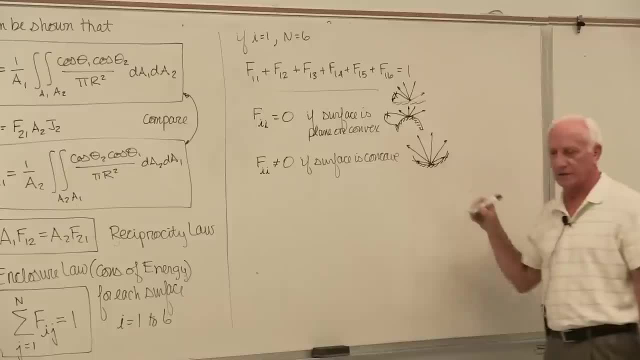 Some of the radiation leaving the small differential area strikes the area. so FII is not zero there, because radiation leaving the surface can strike the surface. In words we say: the surface up here cannot see itself, The surface right here cannot see itself. Here the surface sees itself. 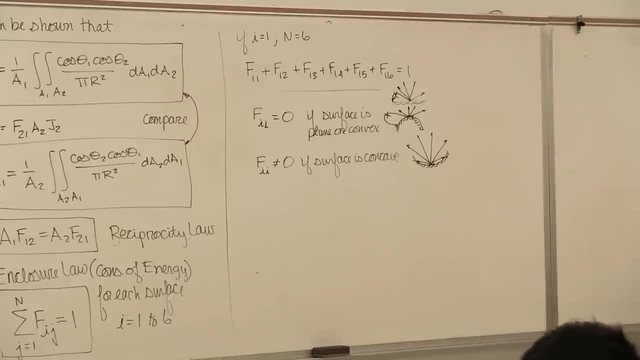 The word see. we relate to our eyes, our eyes. If I put my head on this wall and if I could get it right by the wall, do I see the front wall? Oh no, I don't see the front wall. Don't turn your eyes, your eyes, like that. I mean I could, I still wouldn't see it. 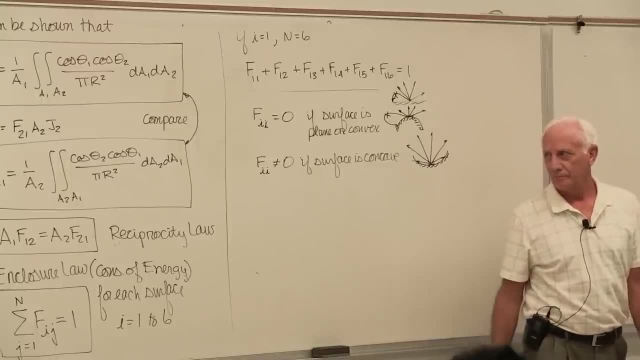 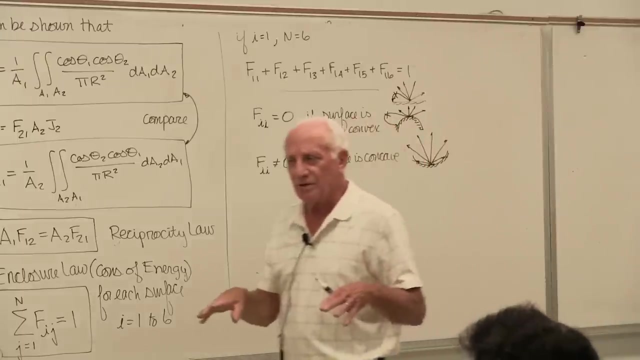 Conclusion: that surface does not see itself. I put on a surface like this- Oh yeah, I can see my hands on both sides of my head. That's concave. That's why it's called the view factor, because it relates to what we see with our eyes. the 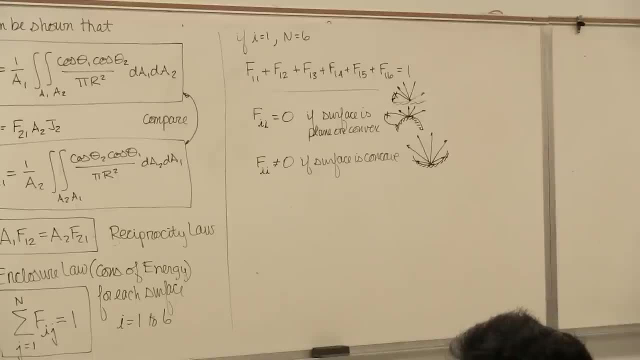 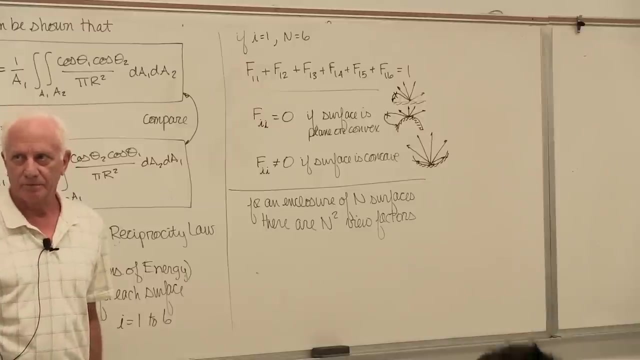 view with our eyes. It helps us to see things. It helps us to see things, Okay. so another thing for an enclosure: Okay, Okay, Okay, If you've got n surfaces. there are n squared view factors In this room. there may be six surfaces. 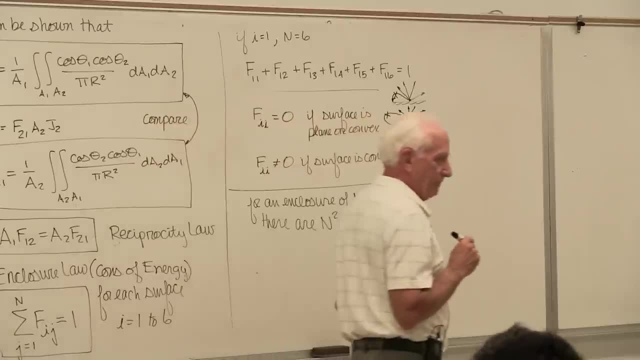 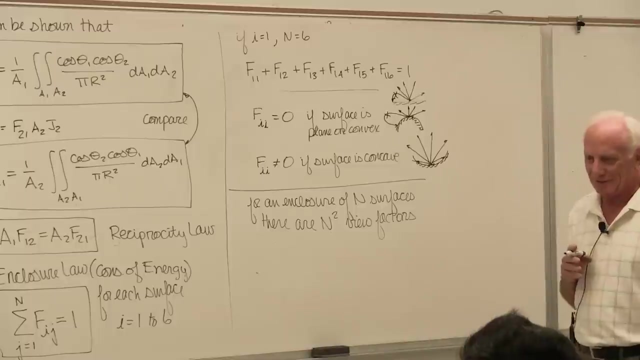 How many view factors? Six squared 36.. F51.. I mean, it goes on and on. Okay, 36 different view factors. Now, some view factors are simple to find and other ones are more complex. Let's take some simple ones. first. I'll take one that looks like this: Circular base hemisphere. 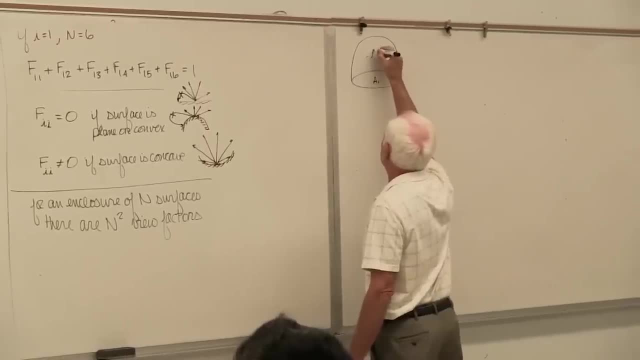 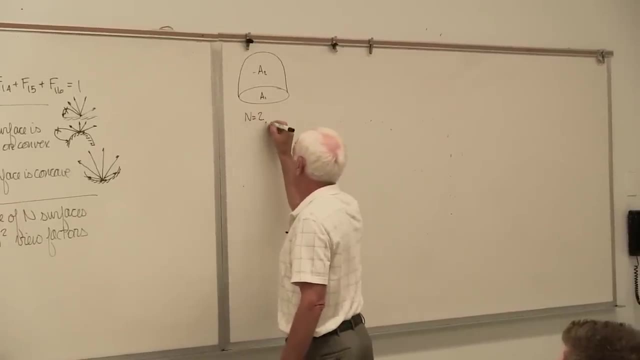 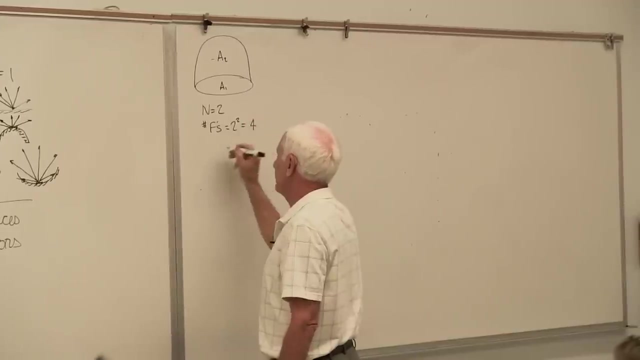 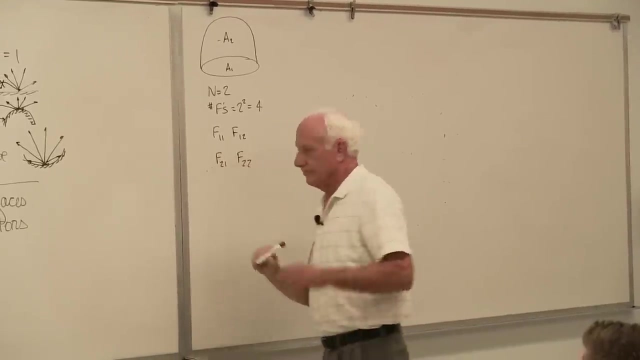 above it. Circular base A1.. Hemisphere A2.. We're looking at the inside now. N equal 2.. Number of view factors 2 squared equal 4.. Here they are, Find them all. Okay, Take a look. 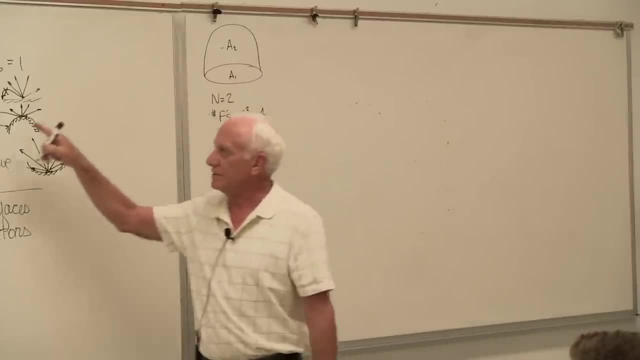 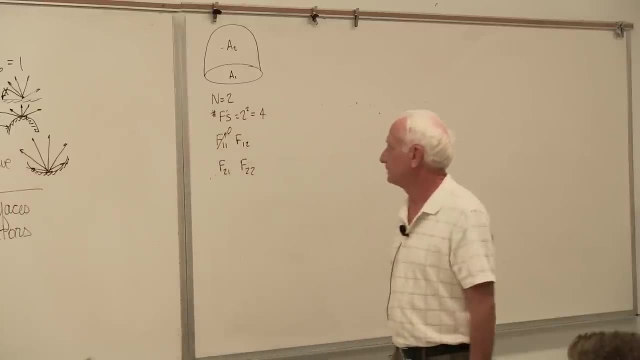 Take the easy one first. I think surface A1 is a plane surface. Yes, it is Therefore F1, 1 is 0, automatically Got it. I think all the radiation leaving surface 1 is going to hit surface 2.. Yeah, 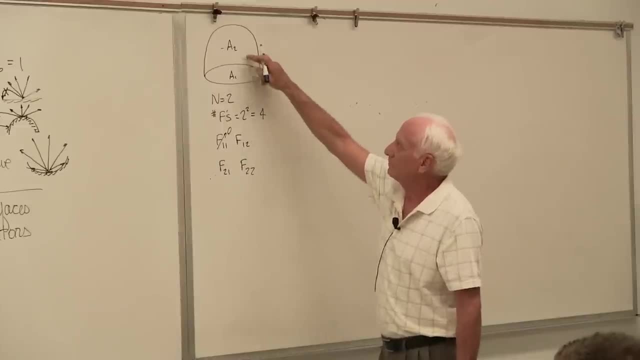 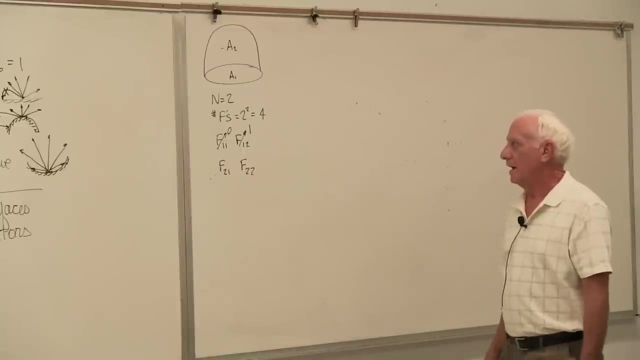 that's right. That's right. It will All radiation leaving. 1 will hit 2.. Okay, 1.. Now I'm stuck. I don't know F2, 1.. I don't know F2, 2.. I'm stuck, but now I use these. 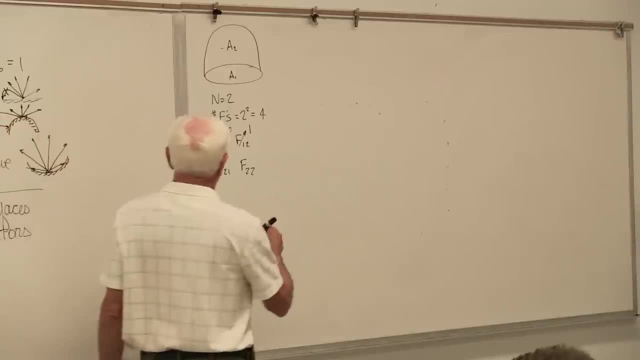 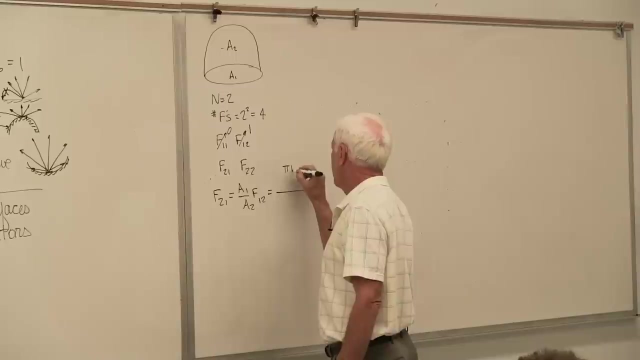 guys. Oh, reciprocity, There we are. Reciprocity: F21 equal A1 over A2.. F12.. F12 is 1. A1, pi D squared divided by 4.. Hemisphere, Hemisphere, Hemisphere, Hemisphere, Hemisphere. 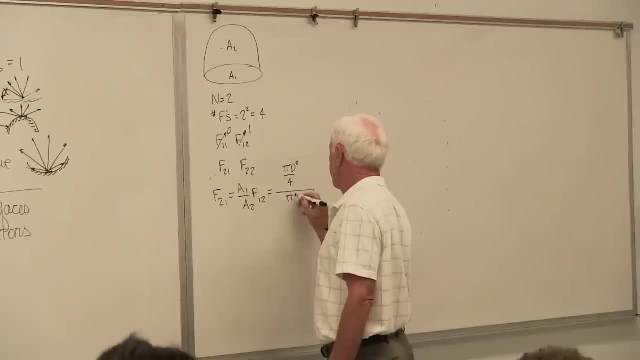 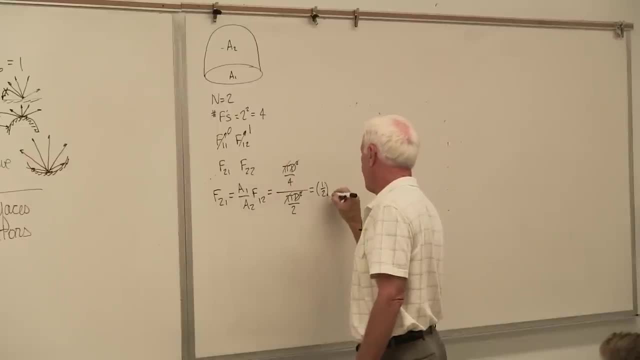 times F12 of 1.. 1 half times F12 of 1. Got it. F22. Enclosure law: 2 surfaces N equal to F21 plus F22 equal 1.. So F22, 1 minus 1 half equal to 1 half. Got it. 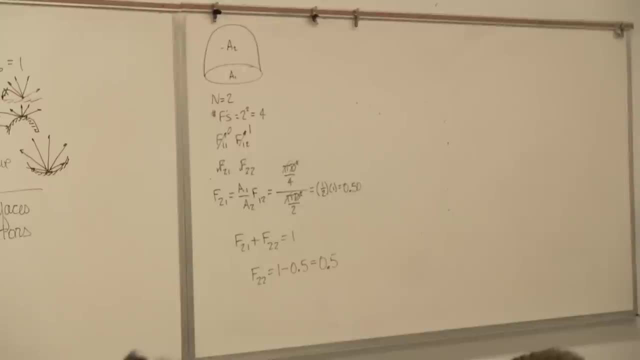 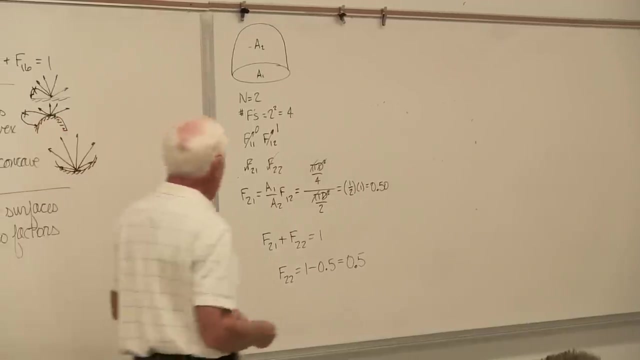 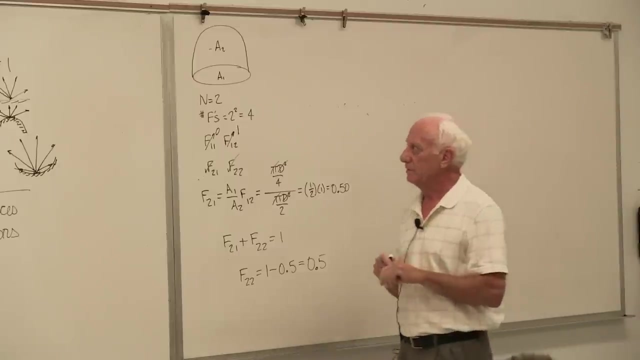 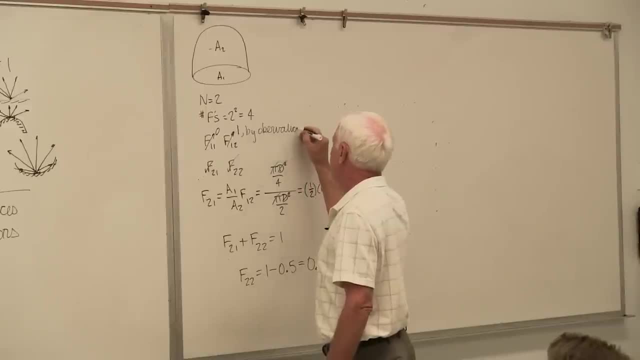 So that's called view factor algebra in a wayiß. I said F12 is along. By what rule? By observation else can the radiation go? that leaves surface A1? There's no place else to go but A2. 100%. 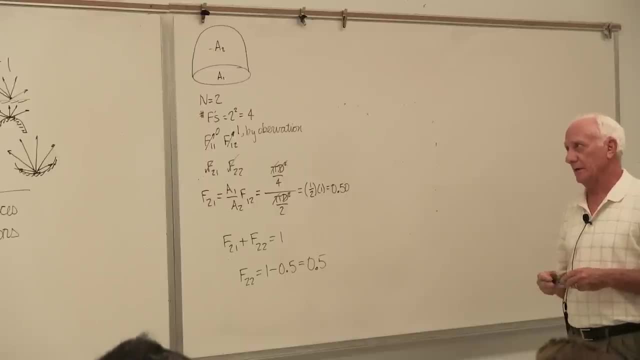 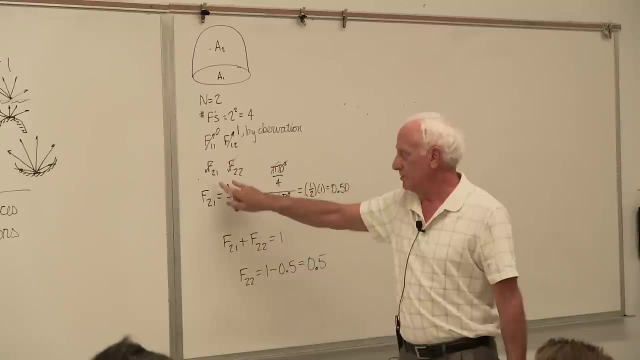 of what leaves surface A1 ends up hitting A2 directly. okay, by observation. Then we use reciprocity: relate those two guys. Then we use enclosure law to relate those two guys. Then we use this definition of a plane: surface F11 is zero. That's called view factor algebra. 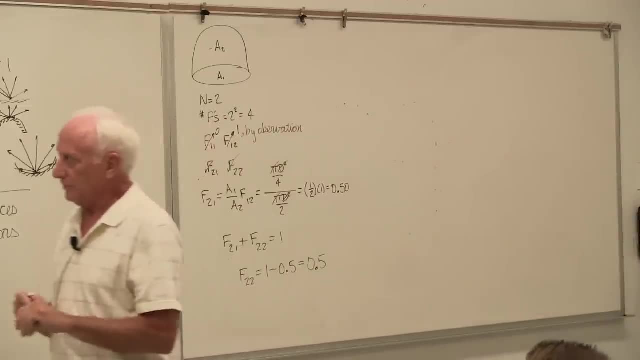 Now, a lot of times it's not that simple. A lot of times you have to go back to the basics and find these guys from that equation. So I'm going to show you how you do that. First of all, we can go to table 13-1.. Yeah, table 13-1.. Let's see here. 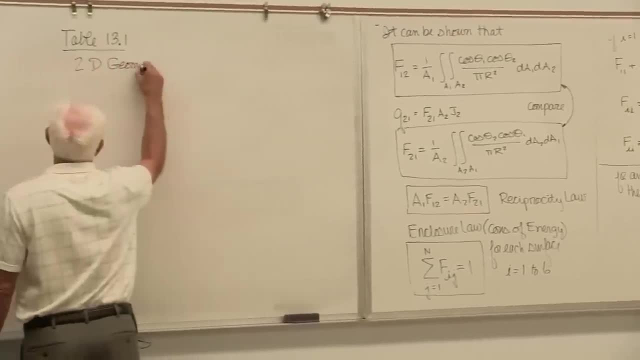 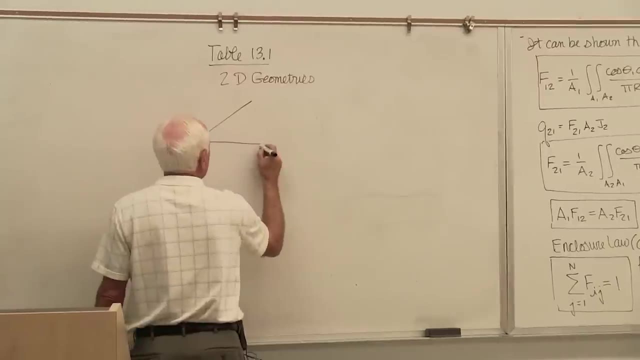 These are two, three, four, five, six, seven, eight, nine, ten, eleven, twelve, thirteen, twenty-two D geometries. One, for instance, looks like this: There are seven given in the table, seven in the table. This is distance. I'm not going to do it that way, I'll do it. 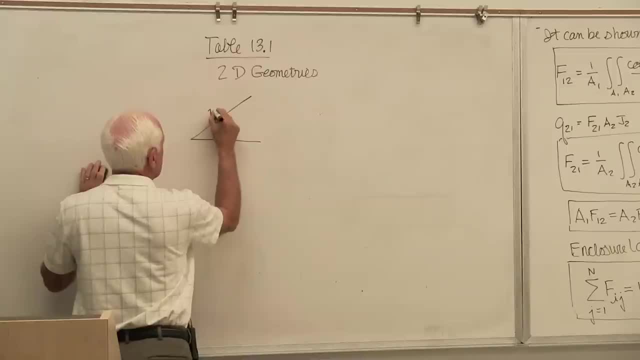 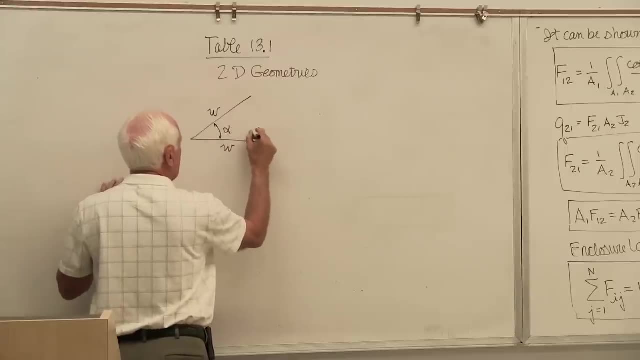 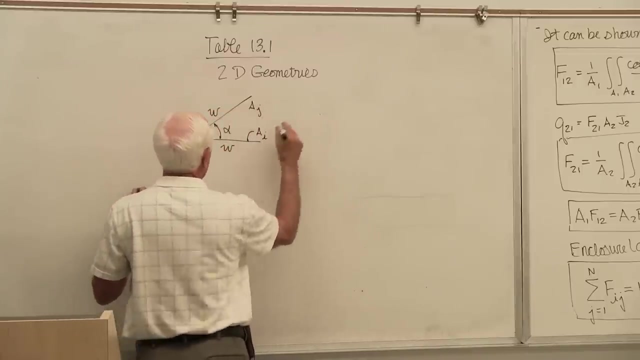 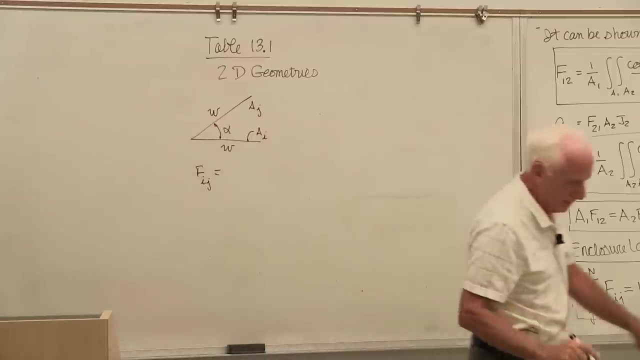 this way: This is distance W. This is distance W, This is angle alpha, This is A1.. And this is, I think he calls it I1.. This is FIJ AIAJ, And then in the table he says that FIJ one minus sine alpha over. 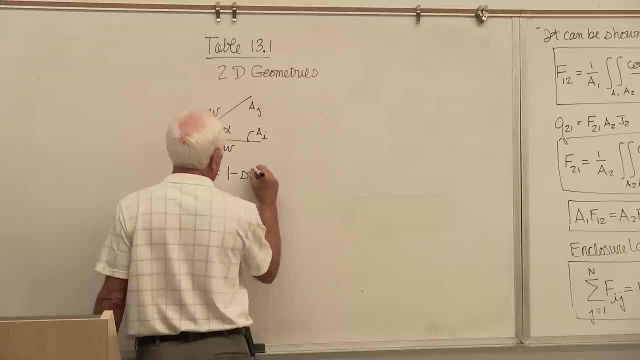 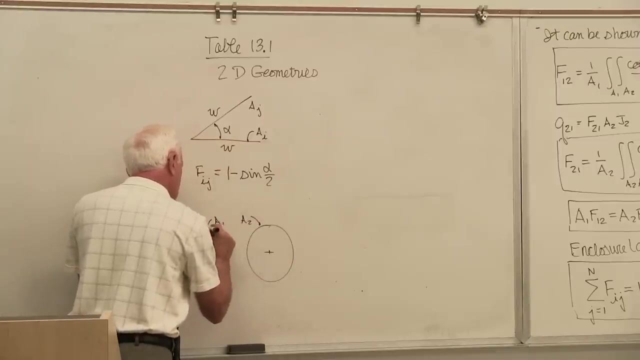 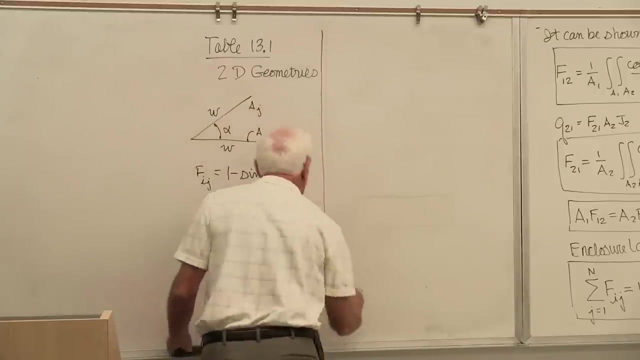 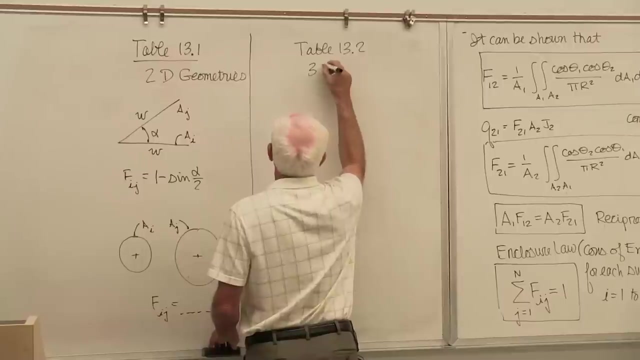 two. He has other geometries. Another one is two different diameter pipes And then like: this is surface a2 and this is surface a1, and then he gives the equation for F. IJ should be IJ. table 13 to 3d geometries. 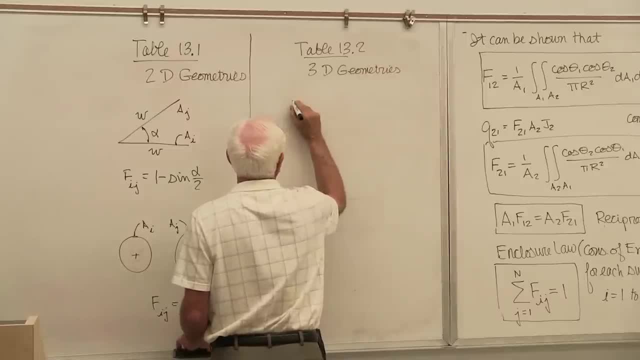 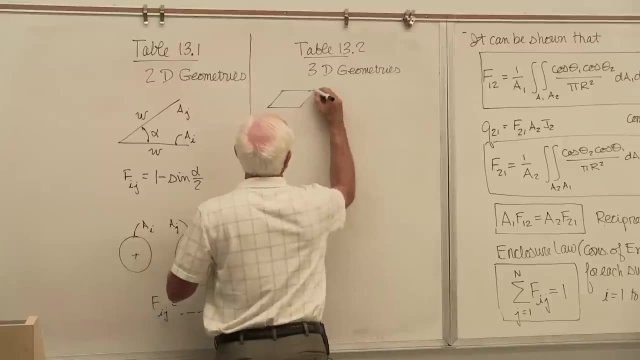 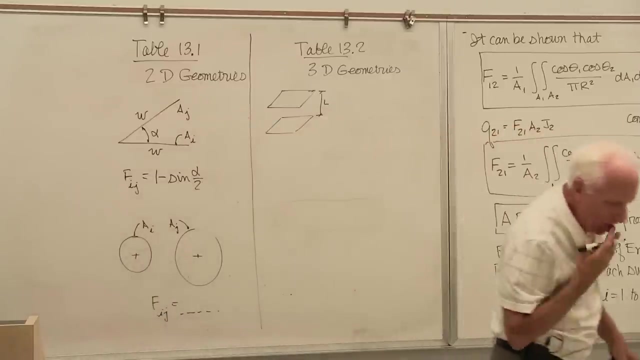 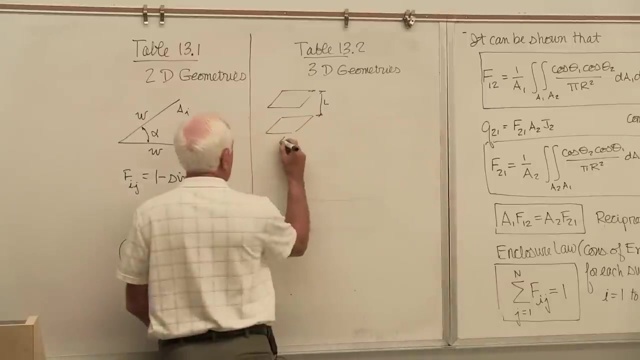 first one: rectangles, one above the other, separated by a distance, L, and he gives us dimensions on those rectangles, XY and L. So X here, X here and Y here, which makes that over 0.. X and Y, This is I, this is J, And he gives us F, I, J. Oh, it's a big long expression. 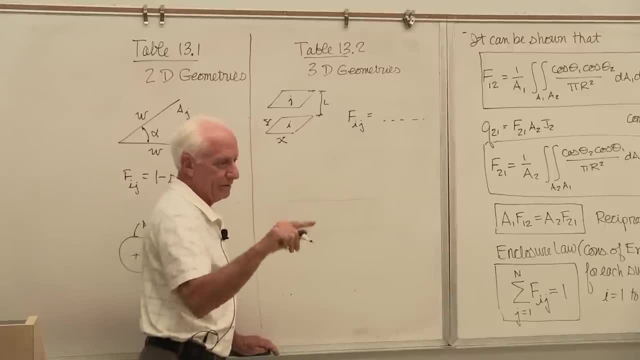 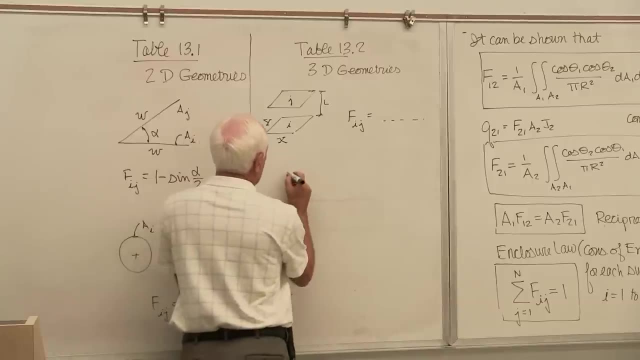 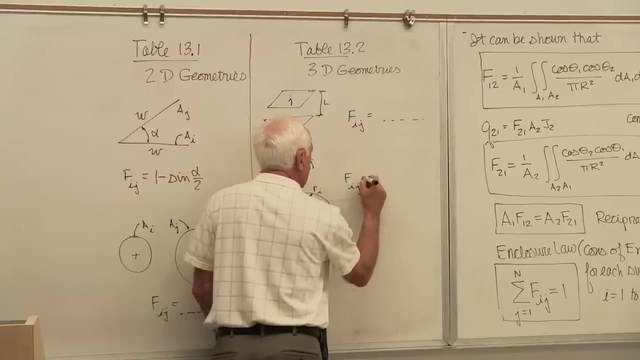 It takes three lines in the table, three lines Natural log, inverse functions, trig functions, things like that. It's pretty messy. The second one is two concentric circular disks separated by L. This one is R I, This one is R J, And he gives in the table F, I, J the equation. 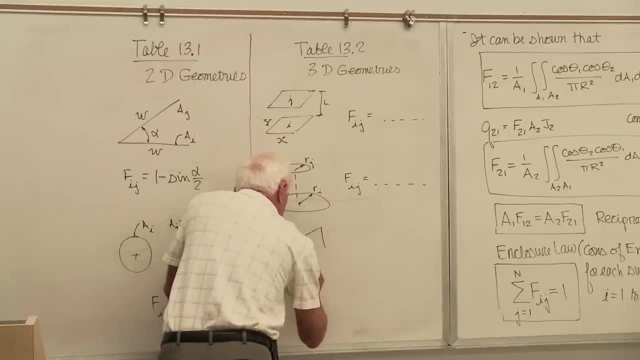 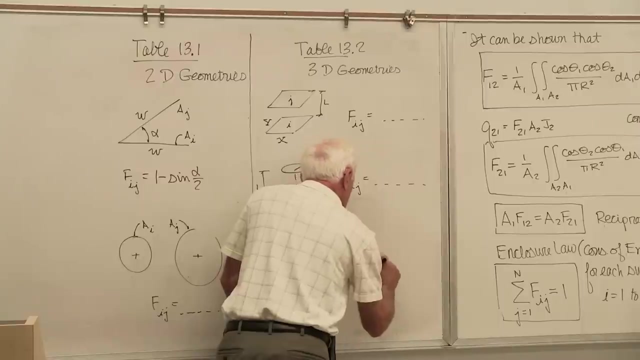 And then he has two rectangles with a common edge. They're normal rectangles, So a right angle there. This is surface I, This is surface J, This is X, Y and Z. And there's an equation given in that table: F, I, J, equal, It's the longest equation of all. Four lines, four lines. 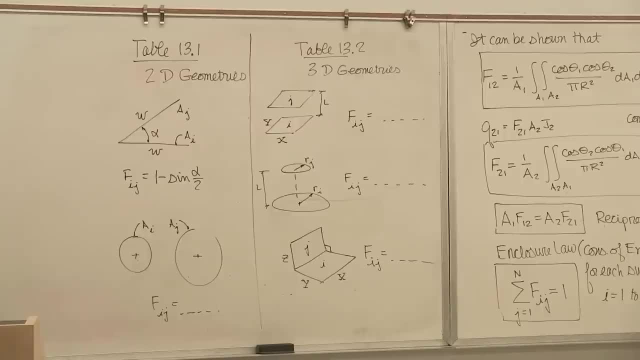 That's the length of the equation. Okay, Those results came from solving this double area integral. Double area integral. It's, it's really messy, It's really messy, It's really messy, Uh, Uh, Uh, Uh Uh. 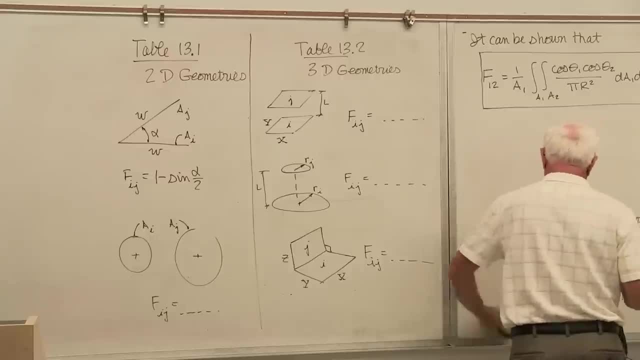 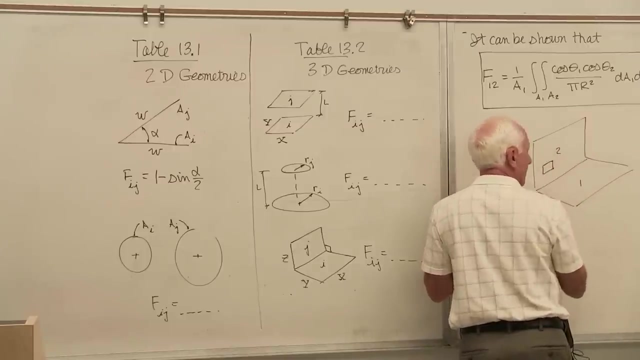 Uh, And because it's a double area, integral, so if you Here's a one and two, So here's a little differential area. Uh meal, This is uh x two, And we call that Z. This is uh d x two, d z two. 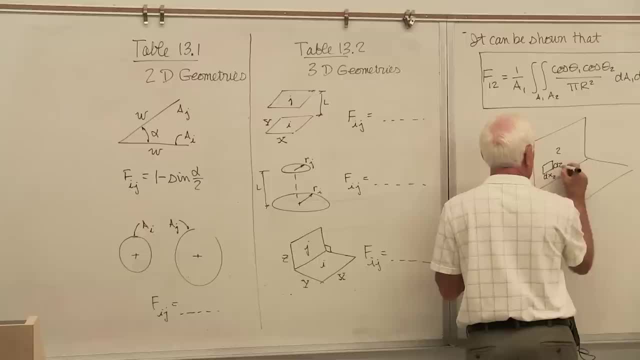 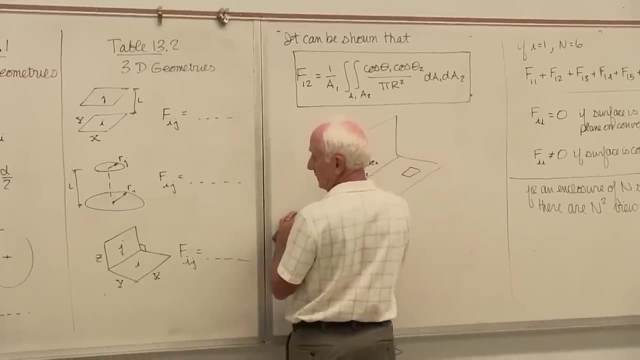 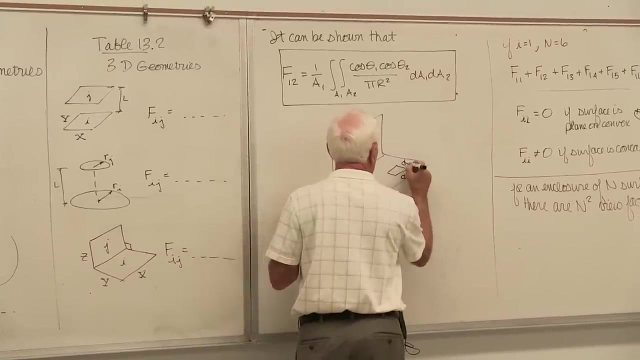 Uh, Uh, Uh, Uh, Uh. And over here here's a small differential area, and this one is dx1, surface 1, and this dimension is ydy1, and here is r and there is the angle theta2,. 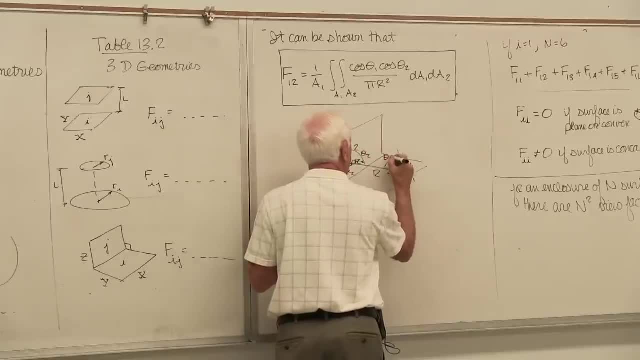 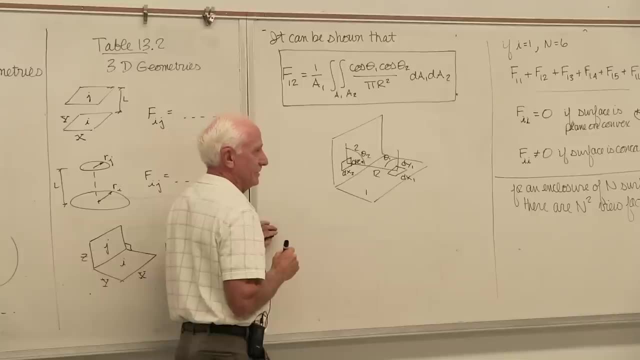 and there is the angle theta1.. Okay, now go ahead and find r in terms of those x1, y1, x2, z2.. Go ahead and find cosine theta1 in terms of the y's and the x's and the z's. 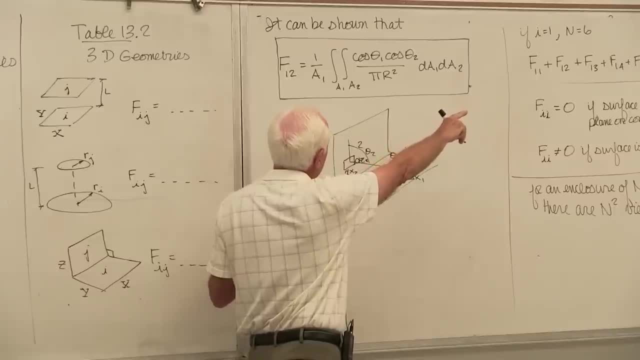 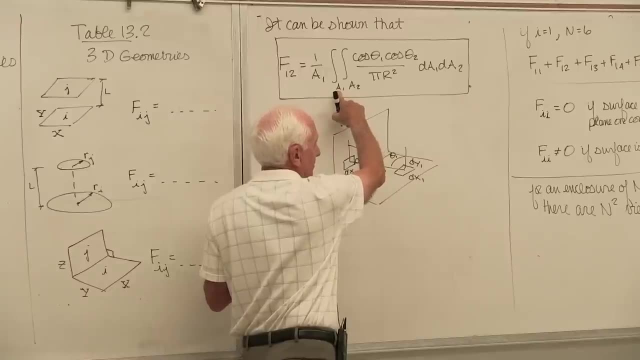 This thing becomes humongous, humongous. You've got four integrals: integral with respect to x1, y1, x2, z2.. Oh yeah, for one of the simplest possible geometries, the front wall and the floor. 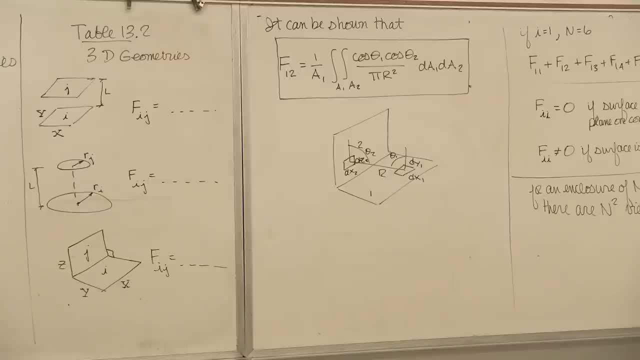 two rectangles, a common edge at right angles. It's simple. It's a real tough job, a real tough job. Obviously, we don't do this in ME415.. We save that for the graduate students. They're the ones we love, you know. make them work hard. 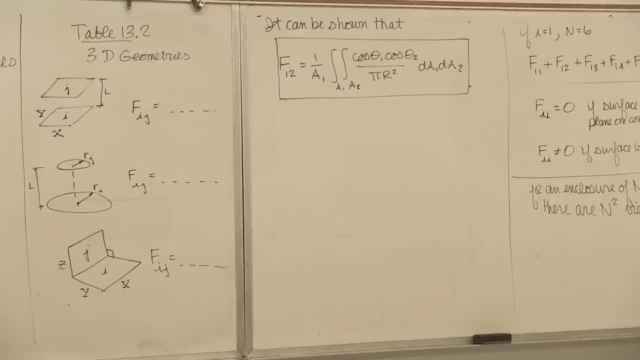 So if you take the graduate course here in radiation, you'll probably do one of these in your life. I mean at least one in the course. They'll make you do one because they want to make you see how tough it really is for simple geometries. 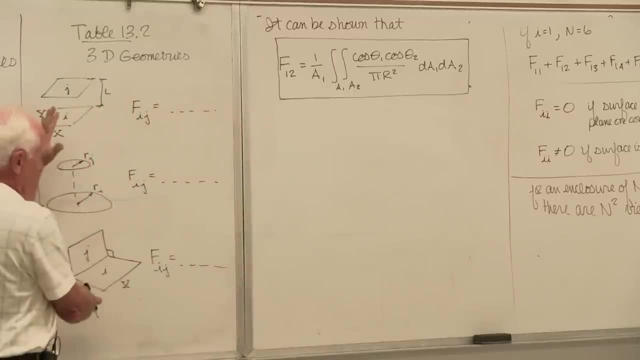 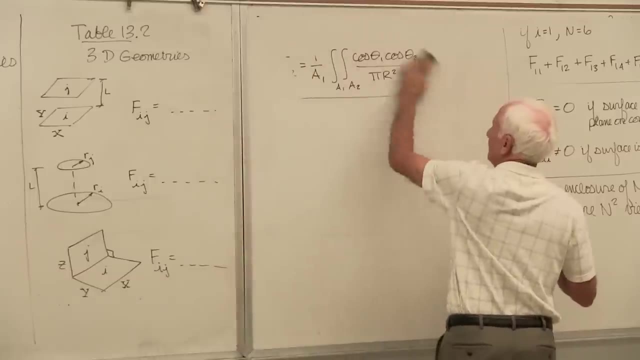 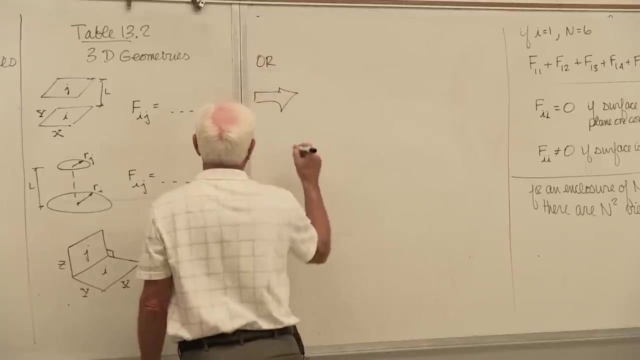 So, yeah, we're not going to do that, though Here are the results done for you. The results are real long equations, Real long, Real long equations. But the good news is he's also given us graphical solutions. So, if you want, you can do the graphical solution. 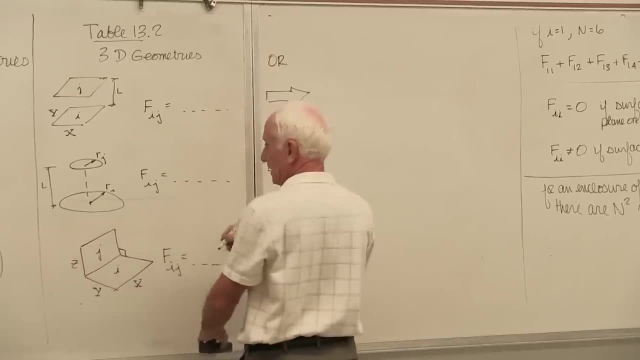 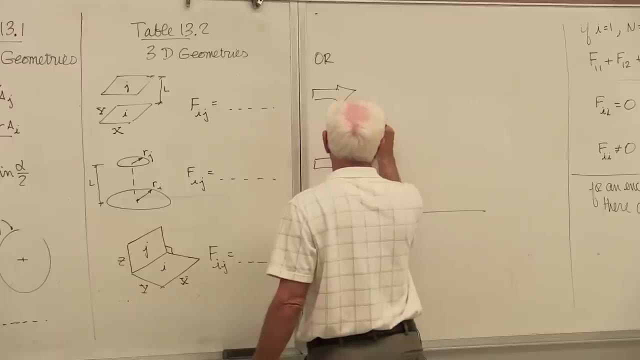 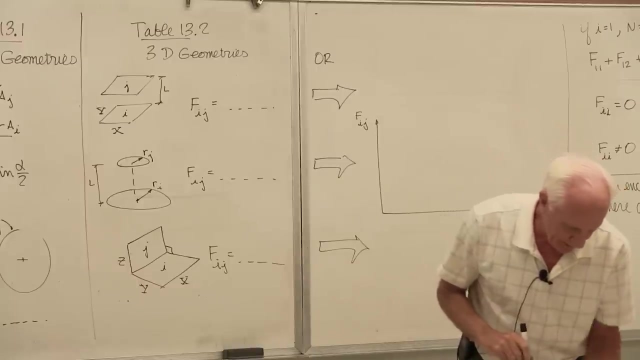 I'll just put a couple on here. I'll put this one on here for you. This is FIJ FIJ. Okay, and this goes from: Let's see that's figure. I'll put the figure down, Figure 13.5.. 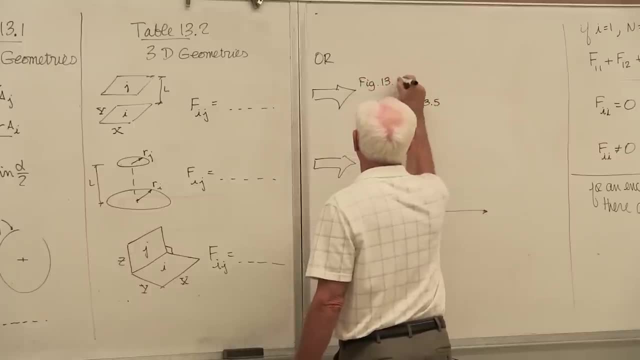 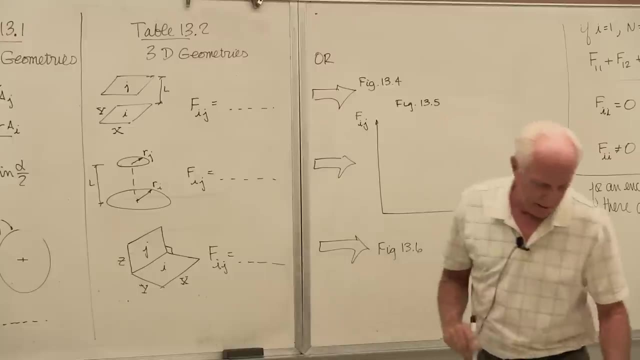 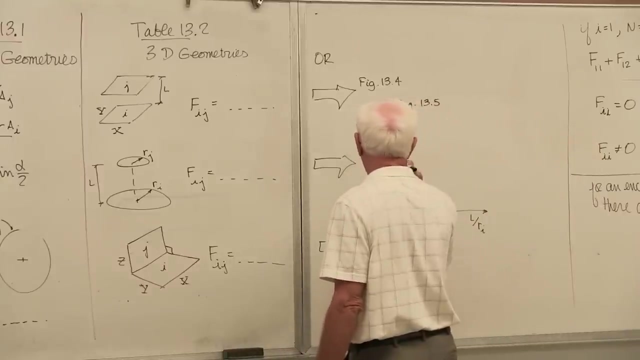 This one is figure 13.4.. This one is figure 13.6.. Okay, the x-axis L over RI. Y-axis FIJ Parametric curves. They go up to 1, 0.. X-axis, logarithmic 1, tenth, 1 and 10.. 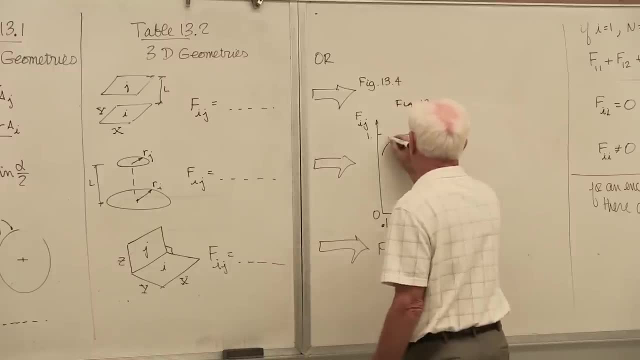 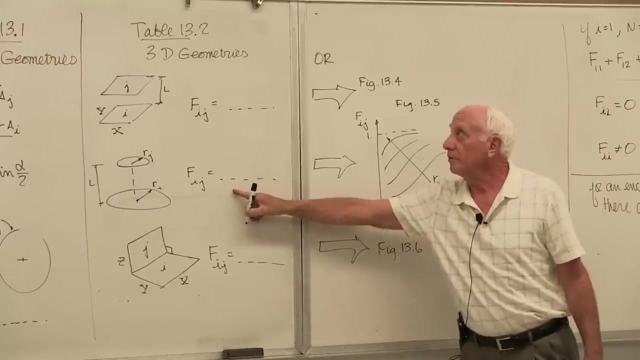 Curves look something like this: If you go in that direction, this parameter increases. That parameter is RJ over L. So this is a very good example of the linear regression of the equation. So the equation in table 13.2,. 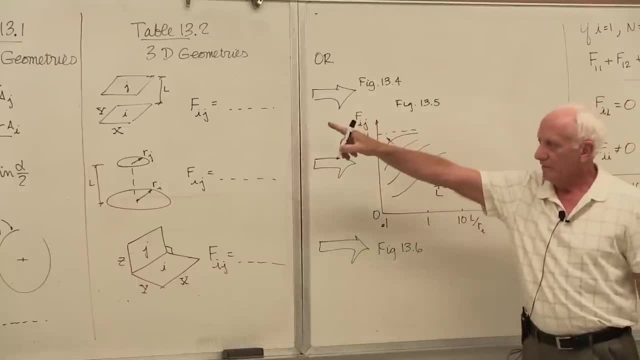 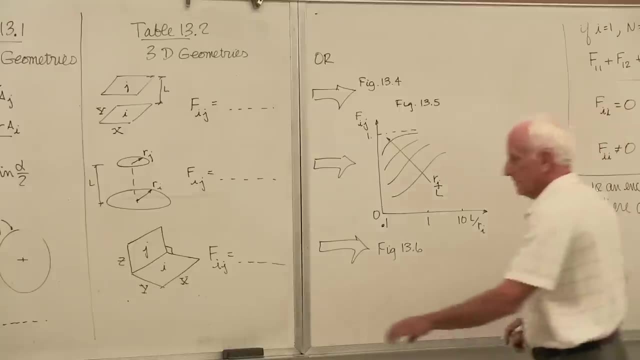 or the graph, figure 13.5.. Same thing for the parallel rectangles or the rectangles common edge at right angles. Okay, so you've got those in your library. That's what you use to solve this stuff if you can't see it. 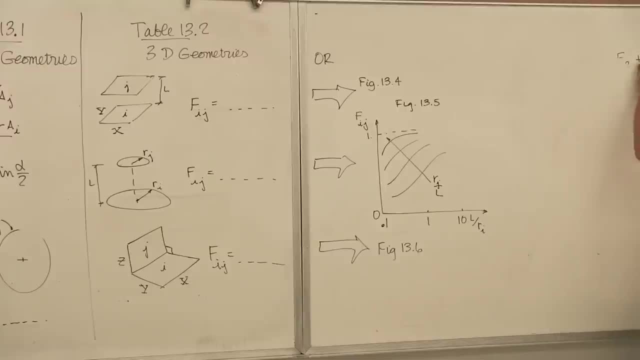 Over here this problem might work. I didn't need to go over there because I said- and here's the magic word- I said I know F1-2 by observation. Without that I'd be stuck. Okay, All right, now we take another one. 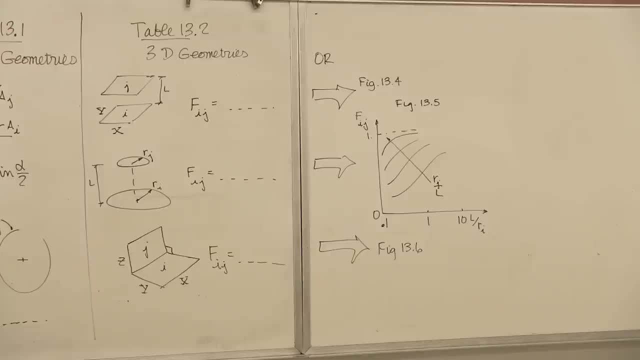 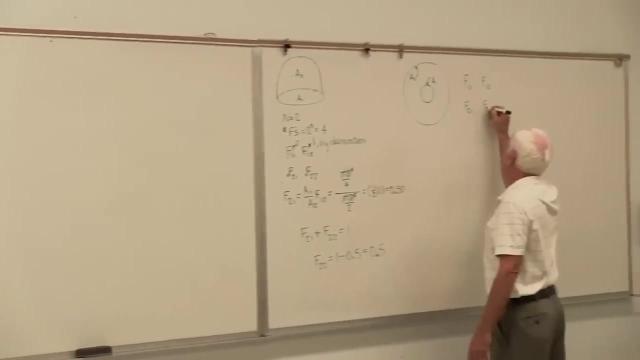 We take and put a tennis ball inside of a basketball. Two spheres: Tennis ball inside a basketball. This surface A1.. This surface A2.. And now we say find all Fs Okay, F11,, F12,, F21,, F22.. 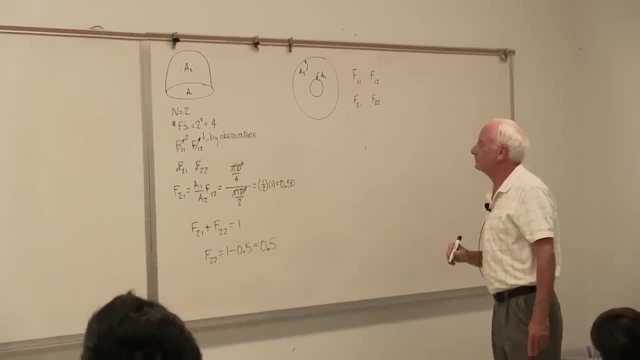 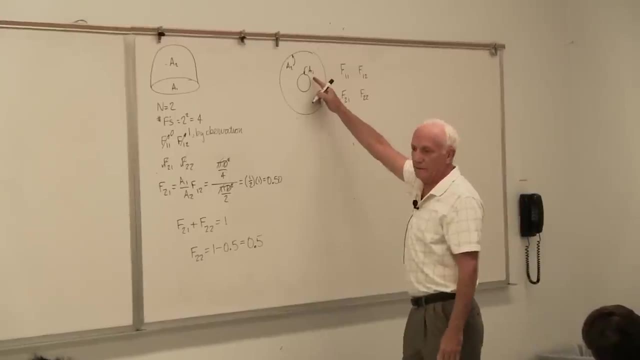 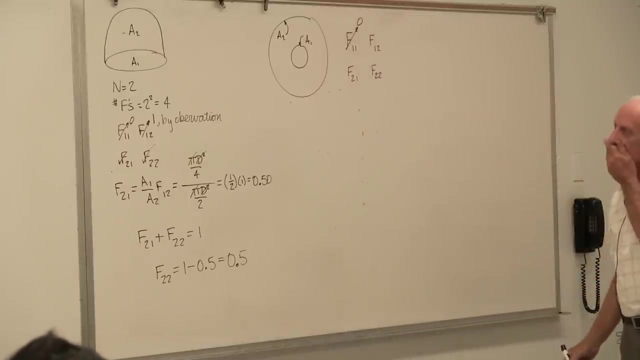 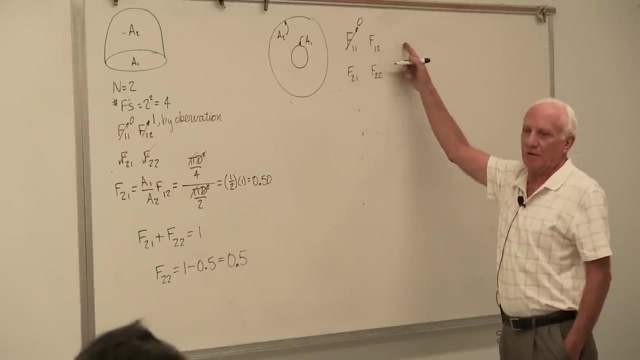 There are no plane surfaces. Nope, There's a convex surface. A1 is convex F11.. A1 is zero. Got it. Now comes the by observation. You don't have to, You can do the enclosure law: F11 plus F12 equal 1.. 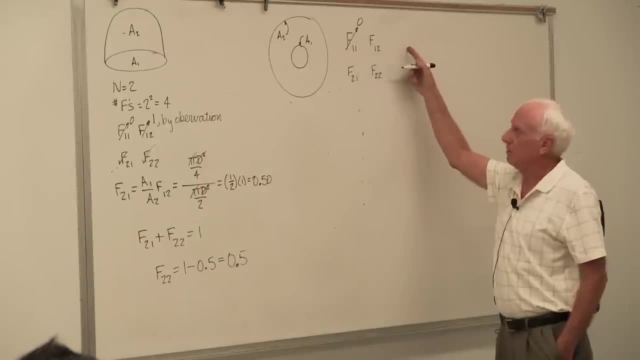 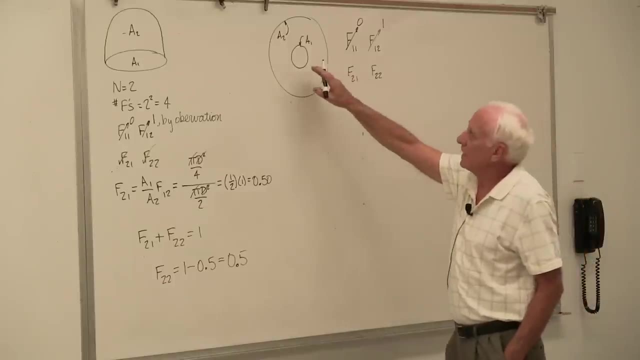 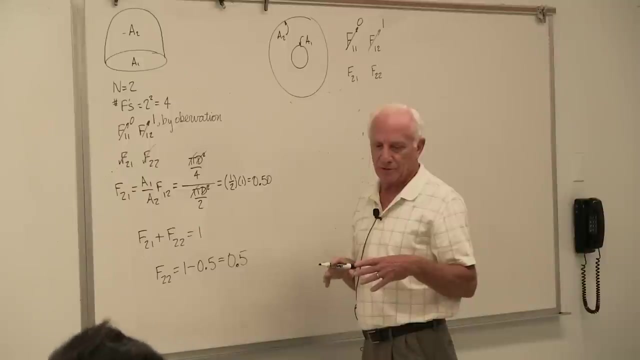 Conclusion: F12 equal 1.. Okay, got it. Or you can say, if you want, by observation, all the thermal radiation leaving surface A1 ends up striking surface A2.. Yeah, that makes sense. Now we're stuck until we use. okay, this is called view factor algebra. 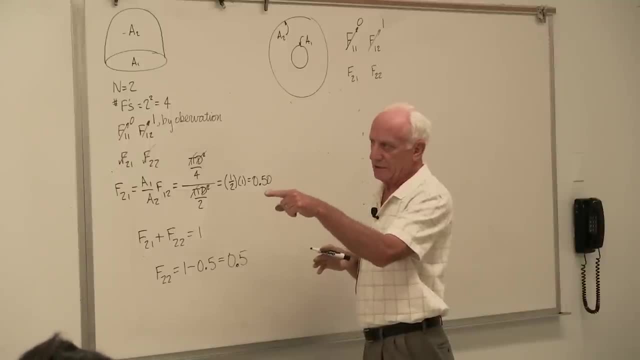 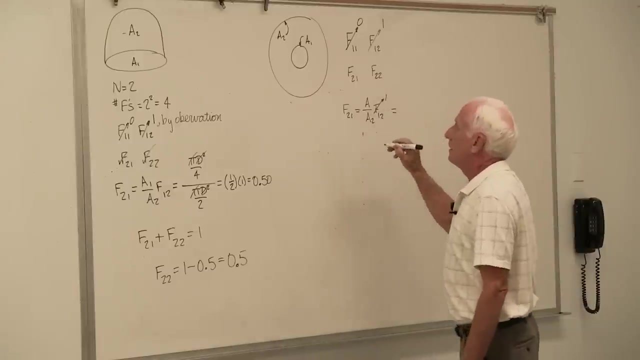 You use those algebraic equations, reciprocity enclosure law, I say okay, F21 equal A1 over A2, F12,. F12 is 1, A1, surface area of a sphere: pi d squared, E1 over d squared. 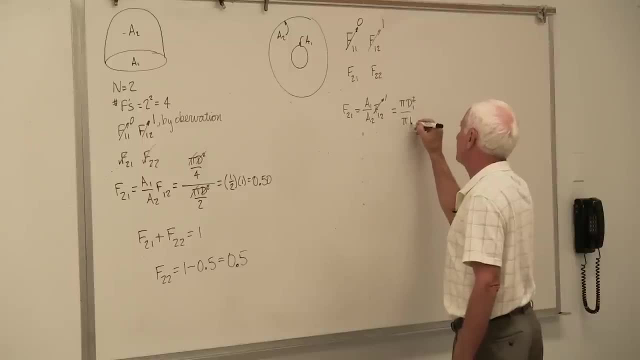 Pi d 1 squared. Pi d 2 squared times 1.. D1 over d 2 squared. So there's F21.. Now I use the enclosure law. Got it: Enclosure law. F21 plus F22 equal 1.. 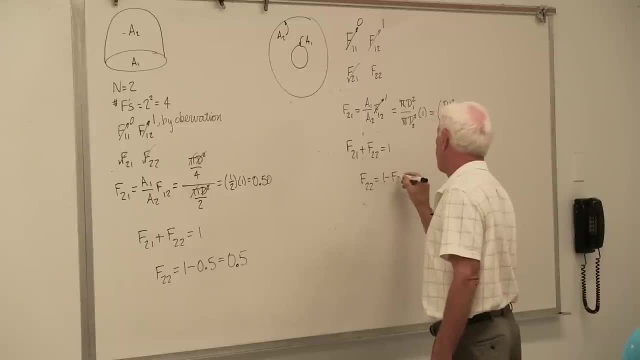 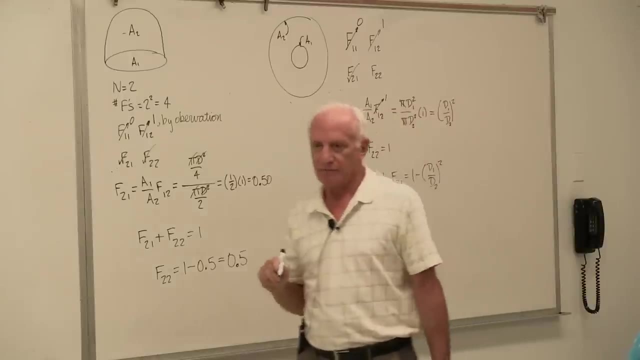 So F22. There it is Found all four view factors. Of course you find the view factors you need to solve the problem. Sometimes you don't need to find all of them, but sometimes you have to find several. Okay, let's do another simple one. 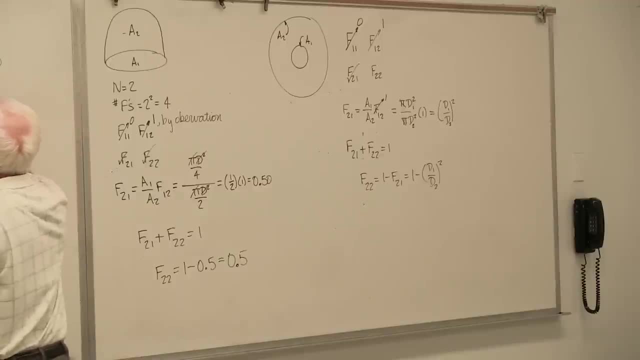 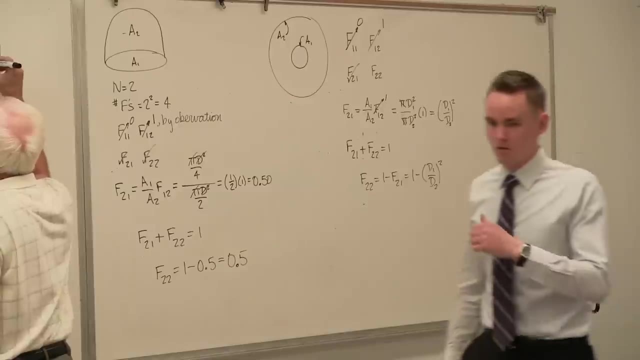 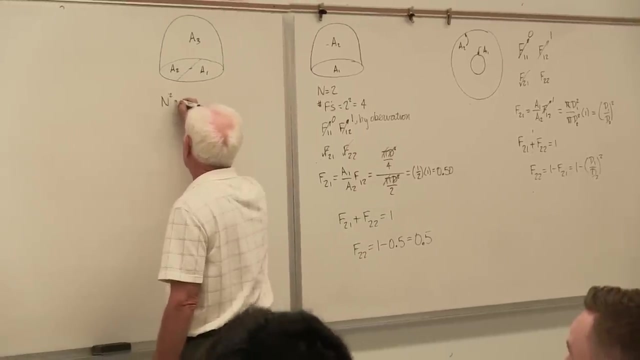 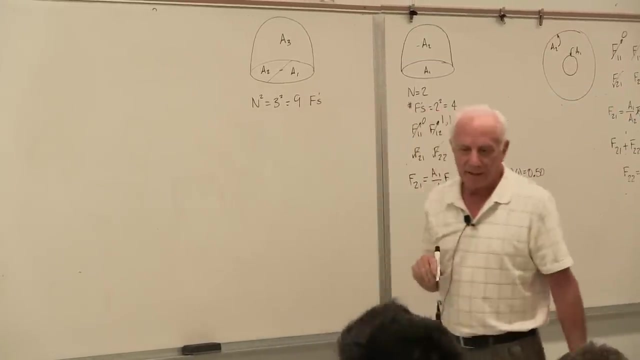 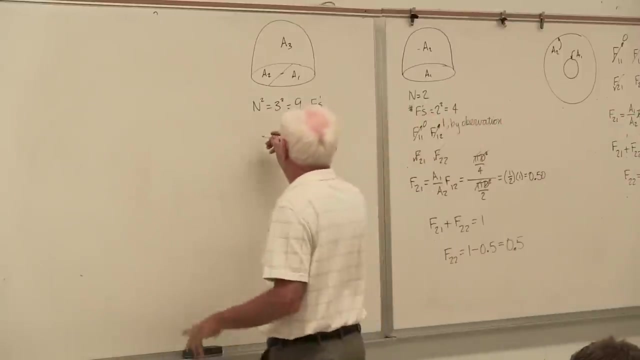 This guy right here again one more time. But now we divide it up into two: a1, a2, a3, n squared equal 3, squared equal 9. f's. Sometimes it pays off if you list them like in a matrix type format or determinant. 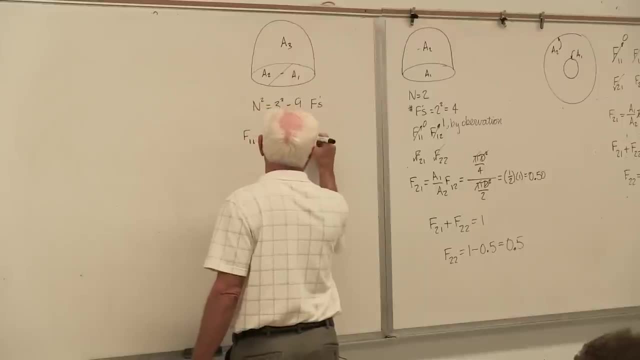 For instance, f11, f12, f13.. Okay, That way you don't forget anything and it helps you too. it guides you. F21, f22, f23.. F31, f32, f33. The name of the game. find all the view factors. 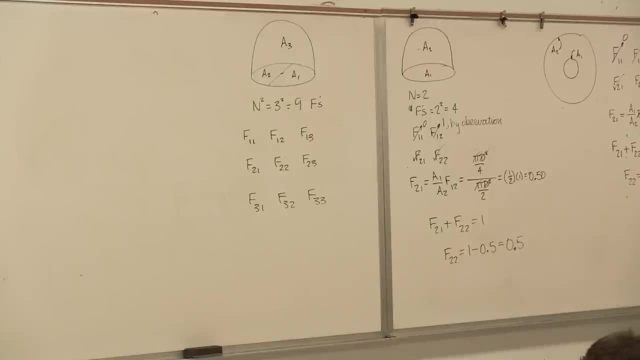 Find all the view factors, nine of them. Take the easy guys first. Are there any plane or convex surfaces? Plane or convex Yep a1, a2, a3.. A1, a2.. Conclusion: F11 is one. 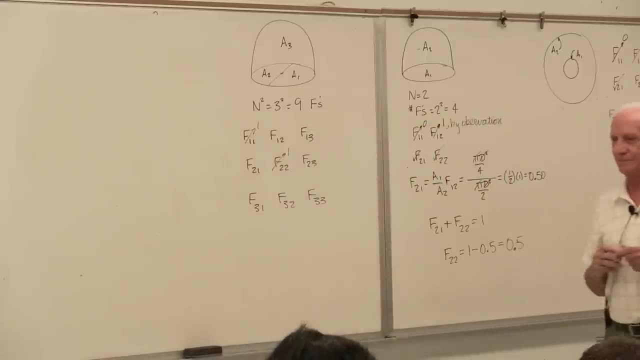 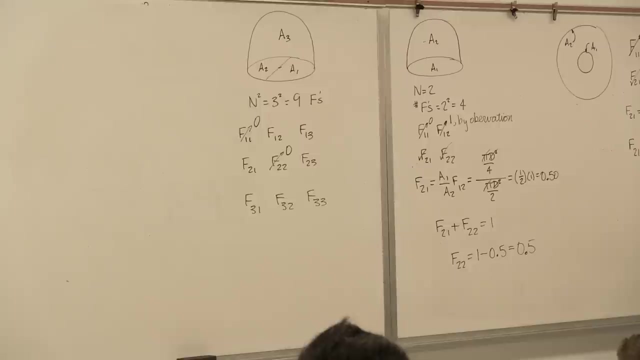 F22 is one, Not f33.. That's a concave surface. Take the easy ones again. I'm sorry. Oh yeah, How about zero? Thank you so much. How about? Can any radiation leaving a1, can any of it get directly to a2?? 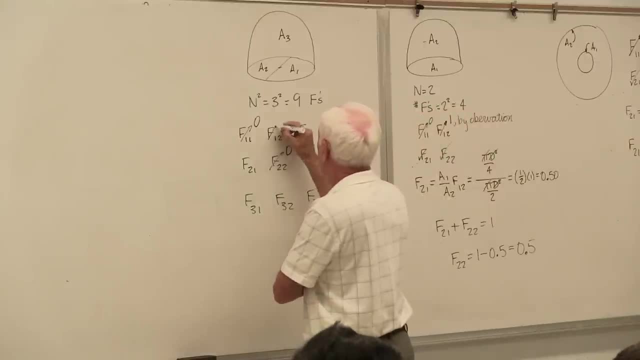 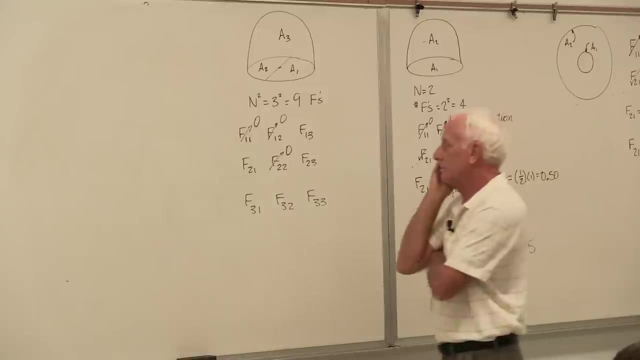 No, No, Uh-uh. F12? Zero. Can any radiation leaving surface 2 get directly to a1? No, A21 is zero. This is going pretty good. The enclosure law: F11 plus F12 plus F13 equal 1.. 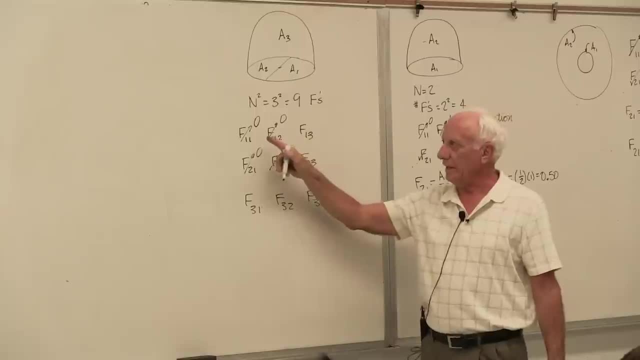 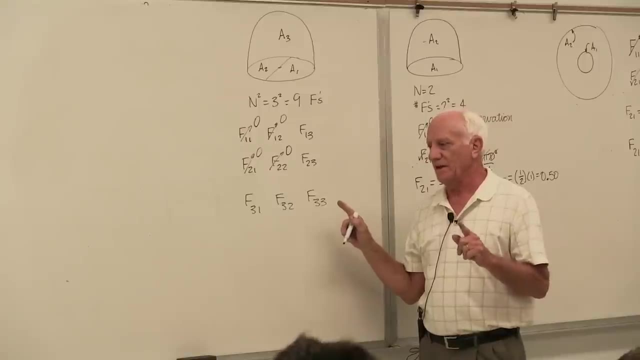 Here's a rule: If I know any of these rows here, if I know everything except 1f, I can solve for that 1f by saying F21 plus F22 plus F23 equal 1.. So what's F13?? 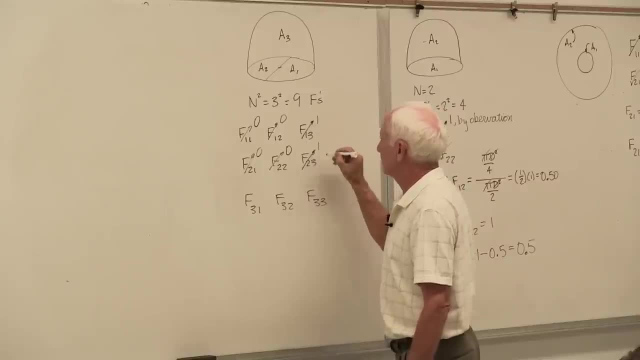 That's easy. It's 1.. What's F23?? That's 1.. You want to talk about energy? Okay, Look up here All the thermal radiation leaving surface 1, can any of it strike a2? No. 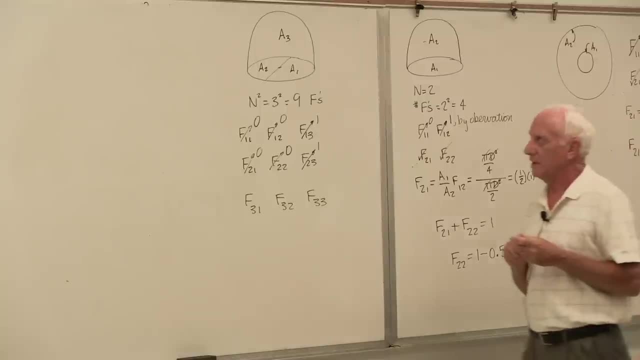 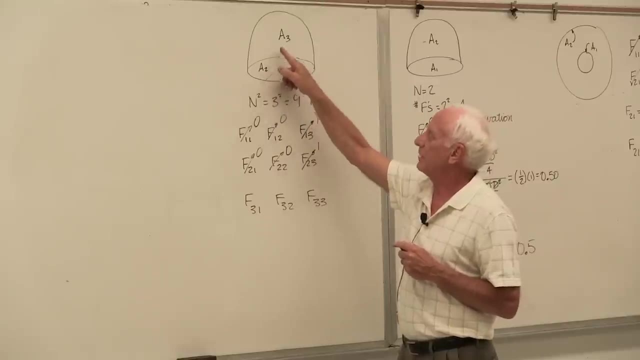 Therefore, where does it all go To a3.? Any radiation leaving a2, can any of it strike a1 directly? No, So where does all of it go To a3.? Now don't play this game. Of all the radiation leaving a3, does half go to a2 and half go to a1?. 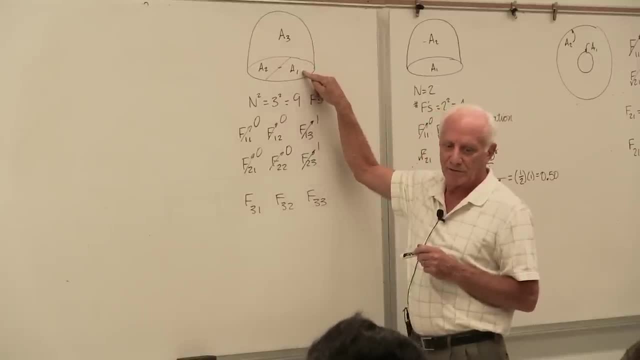 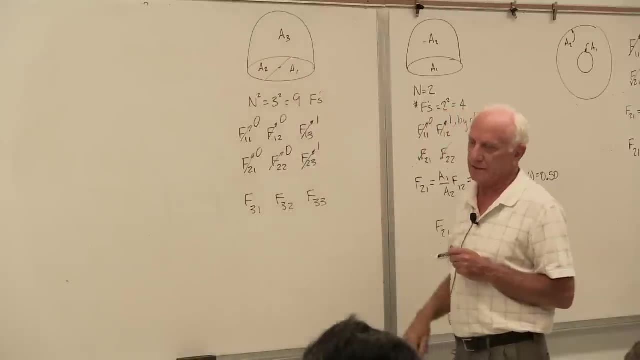 Oh no, Uh-uh, Not there, Because some radiation leaving my fingertip here is going to hit over here. So F33.. F33 is not going to be 0.. Okay, So stop. Now we're done. That was the simple stuff. 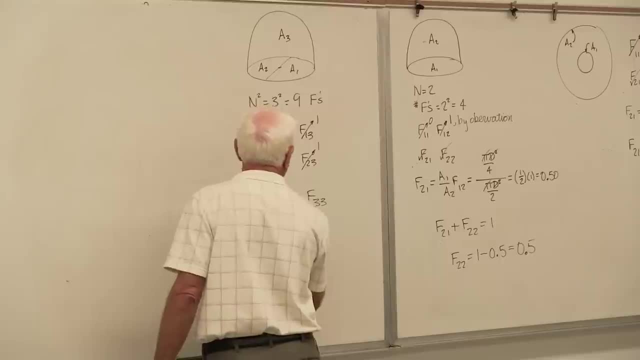 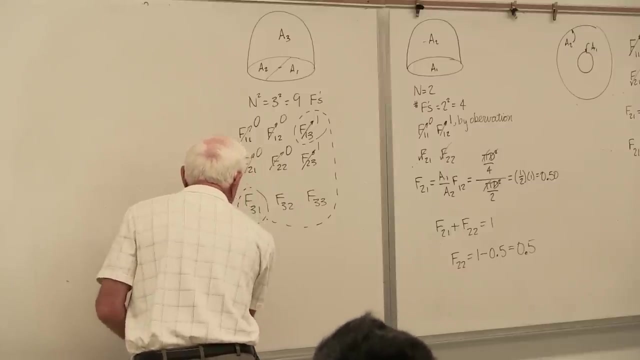 Let's look at F31.. F31. F13.. Reciprocity: A3.. Let's do it this way: F13.. F31.. Pardon me, F31.. Okay, A3.. A1.. F13.. 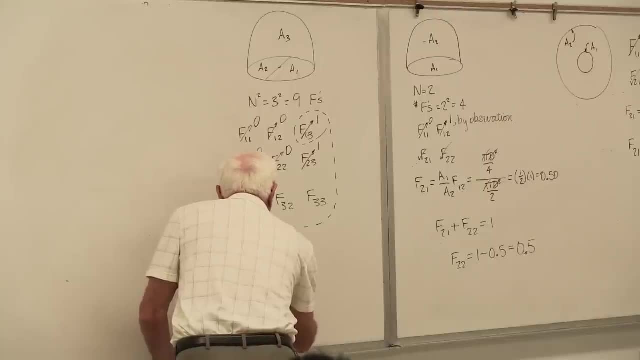 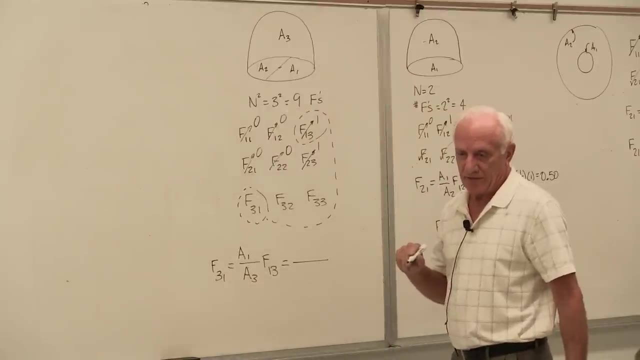 A1. Half of a circle: Pi Pi d squared divided by 4.. So pi d squared divided by 8.. A3. Hemisphere Area of a sphere: Pi d squared. Hemisphere Pi d squared divided by 2.. 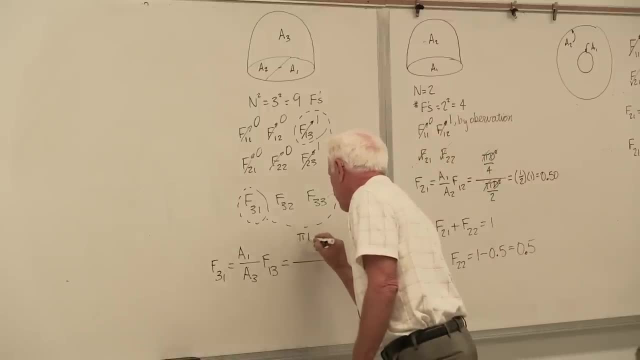 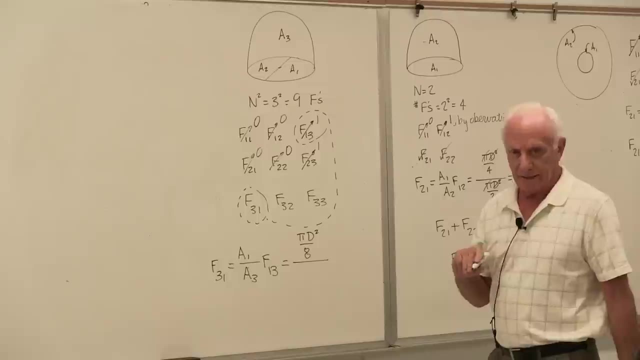 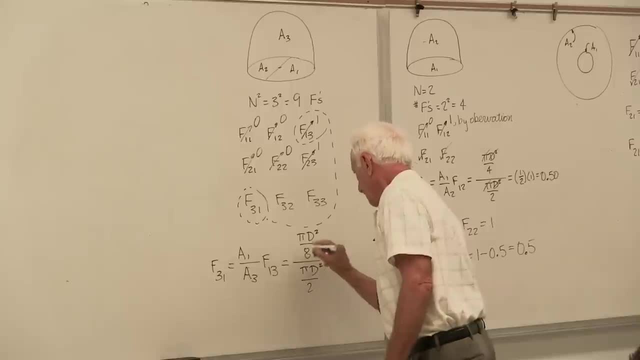 F13.. I found it One: Pi Cancel D squared, Cancel 2 divided by 8.. 0.25.. Yeah, Then I say you know what, By symmetry, F31 has to be equal to F32.. 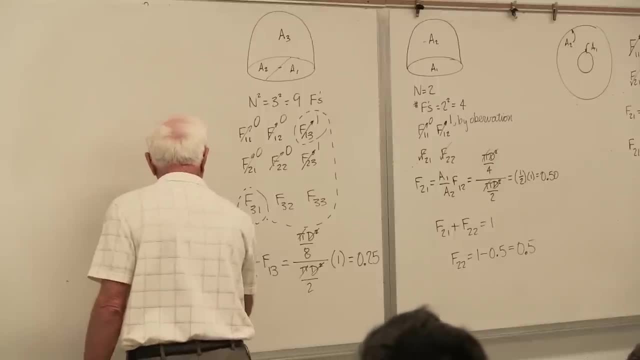 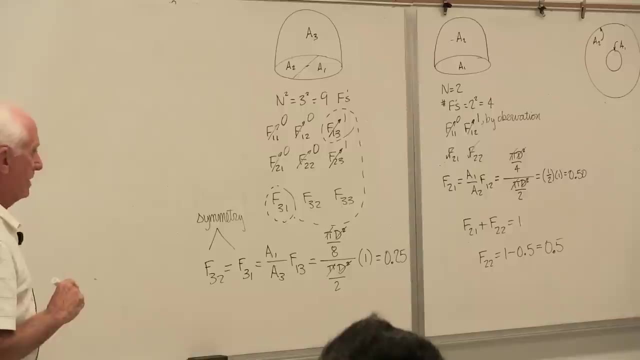 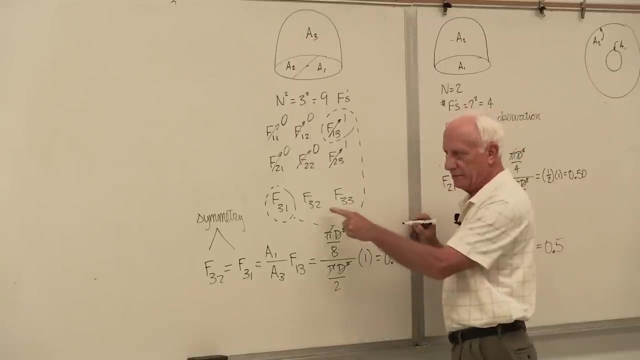 So F32.. How Symmetry? Now I say, okay, now I know everything in the third row except one view factor. I don't know F3,3, but I do know F3,2 and F3,1, so I say F3,1 plus F3,2 plus F3,3 equal. 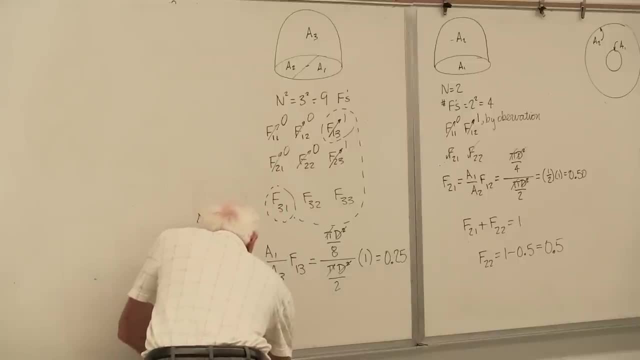 1. So, got it, got it, got it done, found all nine. Did I need to go to the figures or the tables? Nope, nope, nope, nope. Why not? Because I said right here, oops, right up here. okay, F1,3 was 1.. 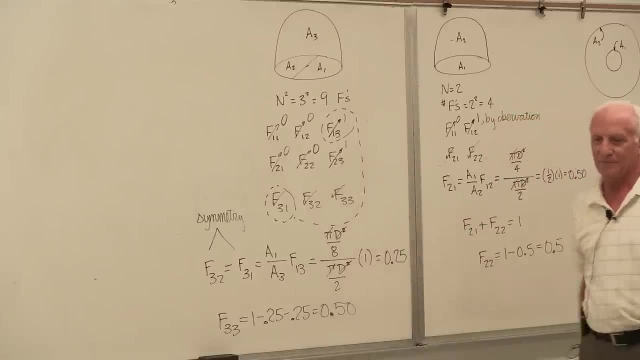 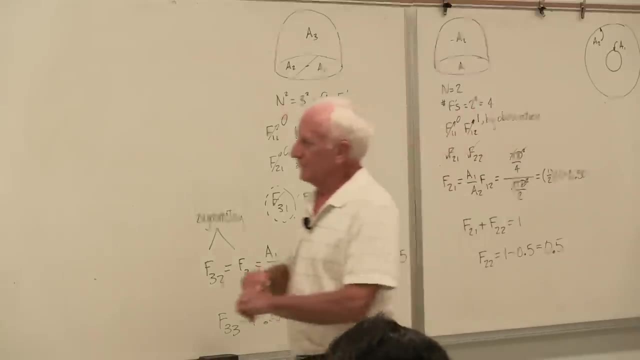 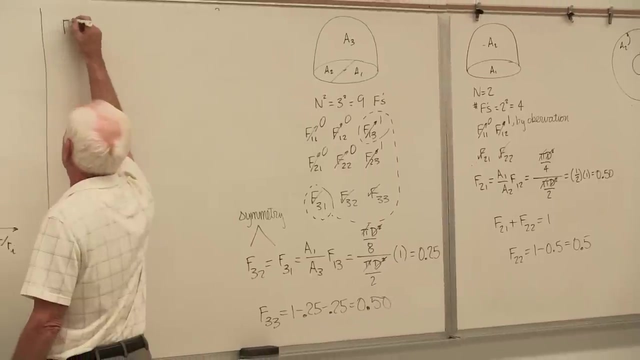 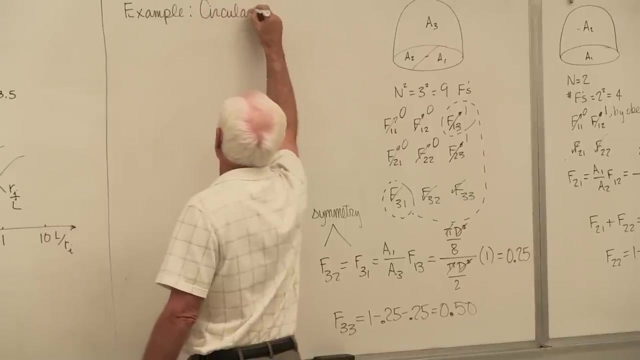 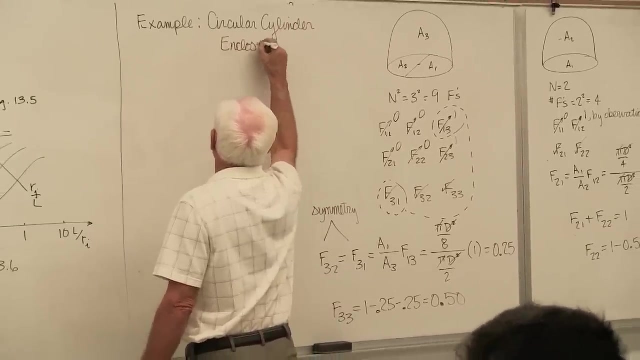 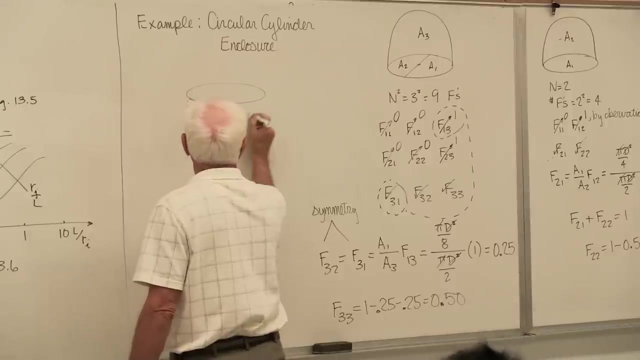 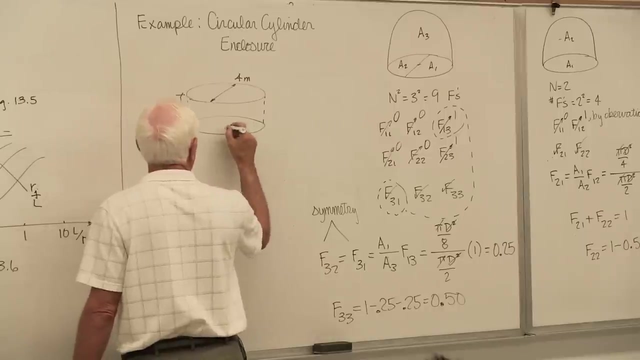 F2,3 is 1.. That was what I had to say to make this thing work. Okay, now we'll try this one Circular cylinder. Okay, okay, okay, okay, Okay, looks like this: This dimension diameter is 4 meters, separated by a distance of 1 meter. 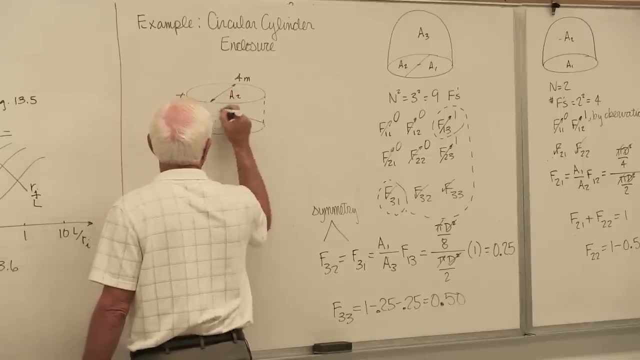 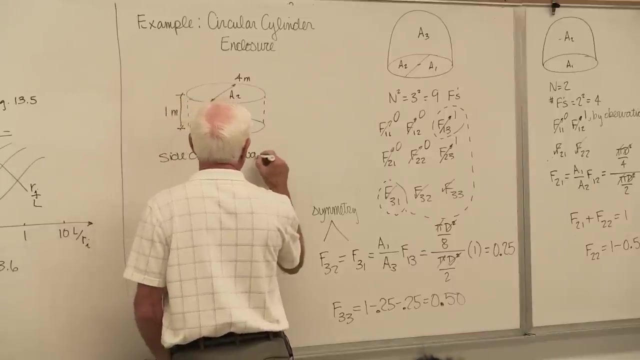 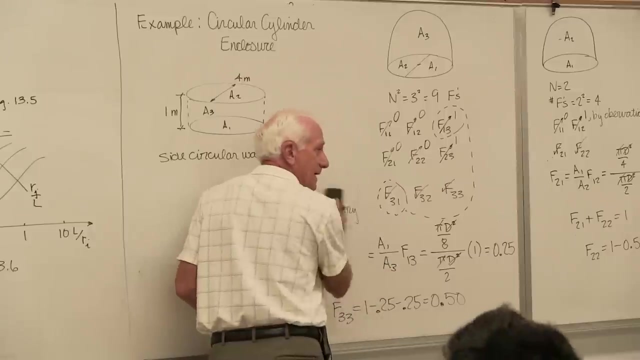 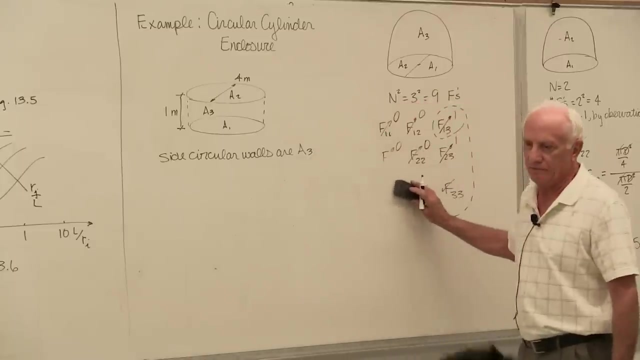 I call this surface A1, this surface A2, and the side walls are A3.. Why do I call them different areas? Probably they have different temperatures. So maybe the temperature of A1 is 1,000, the temperature of A2, 500, the temperature of 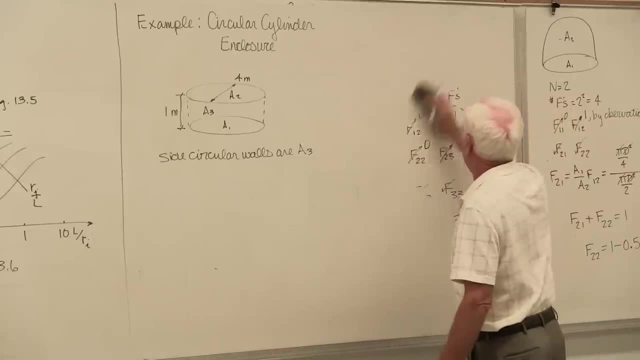 A3, 300.. That's how you number surfaces. They have some differences. One might be adiabatic, One might be a known temperature, So you give it a different area designation: A1, A2, A3.. 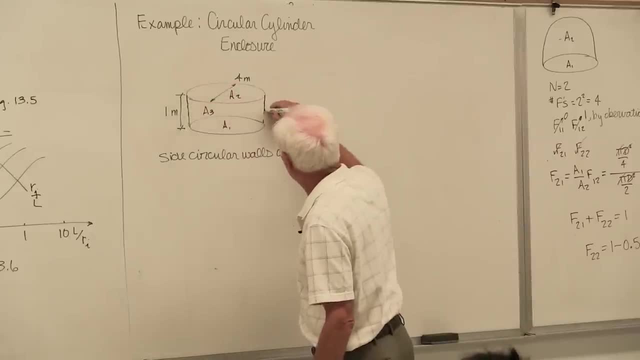 I'm not going to this guy's connected. It's not a dash line, It's a coffee can. The top is A2, the bottom is A1, the side walls are A3.. You see, we're not calculating heat transfer. 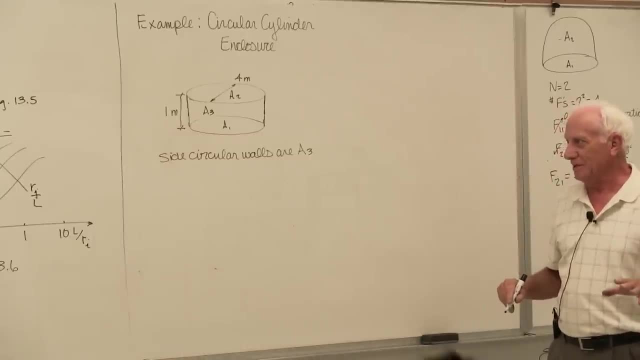 Okay, We're not calculating heat transfer yet. The first step in these problems is you calculate the view factors. Once you get the view factors, then you can find the heat transfer. But you can't find the heat transfer until you find the view factors. 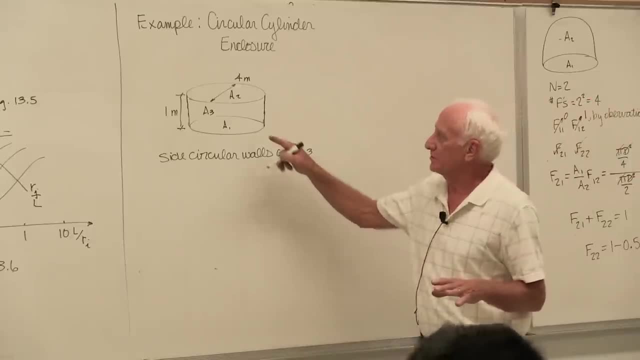 I might say: what is the net heat transfer between surfaces 1 and 3, the bottom and the side walls? The first thing I need is F13 to do that. F13, all right, So here we go again. How many surfaces? 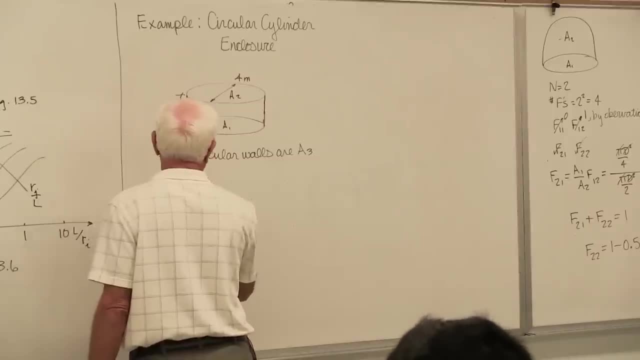 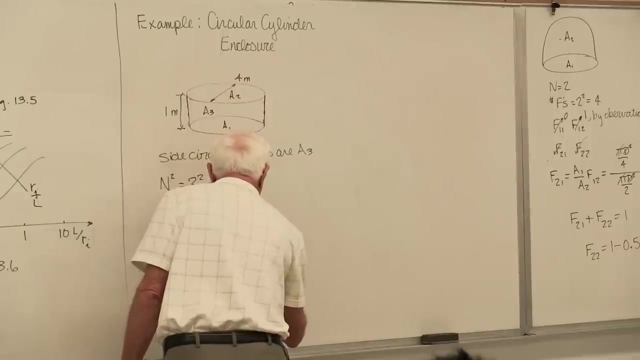 Three, How many view factors? All right, N squared, 3 squared, nine F values, So nine Fs. Write them down, Okay, Now Okay, Look at that and say, okay, are there any gimmies? Oh yeah, there's two of them there. 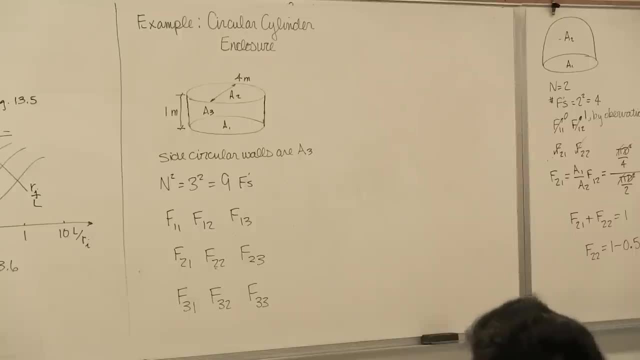 I see two plane surfaces, two plane surfaces: A1 and A2.. Okay, So A1, F11 doesn't see itself zero, F22 doesn't see itself zero, Not A3. It's concave, Okay. 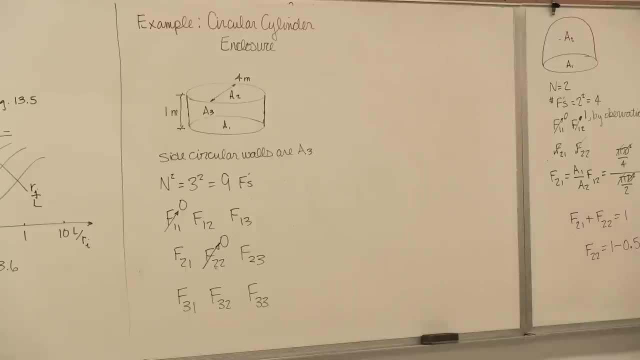 What? concave? a3 concave. okay, do I see anything by observation? a number? give me a number. no, I don't know, I go over here observation. the number is one over here here. f1 to observation is one. I see it over here. no, I had no idea, but luckily 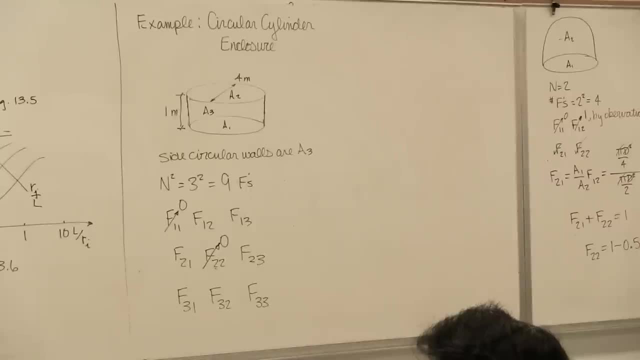 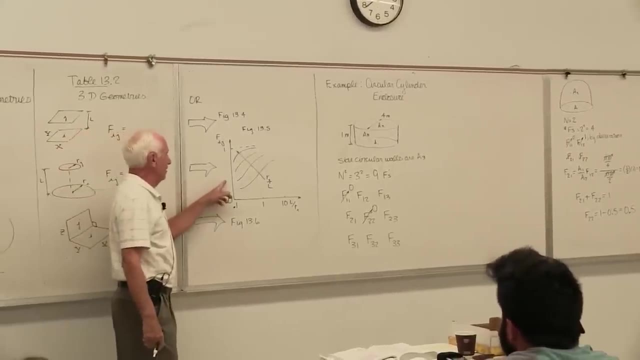 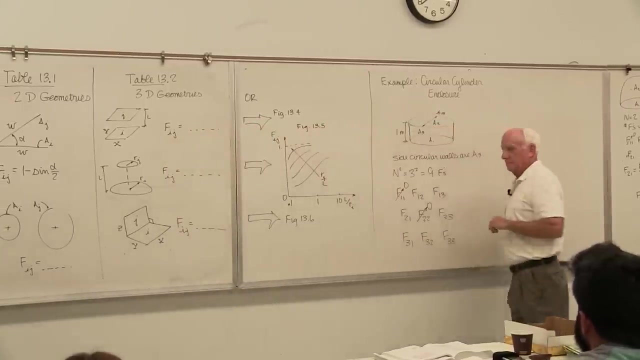 if I go to these tables, table three, two, oh there it is two parallel disks right there, same radius. or if I want, there it is right there on a graph, figure thirteen five. okay, so I'm going to find f1 to two, bottom to top. so I'm going to use, I'm 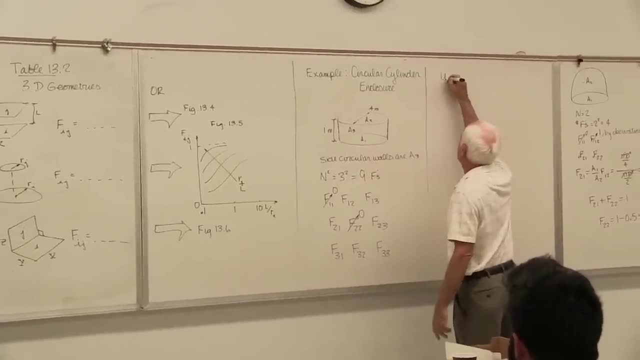 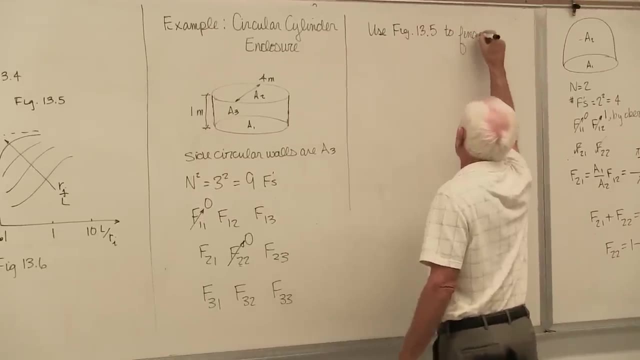 not going to do that long equation, I'm going to use figure thirteen five. first thing you do, would you say: okay, that means I equal one, J equal to. so R, I are J and L. L is 1 meter, the radius is 10 meter and this is I. people said very. 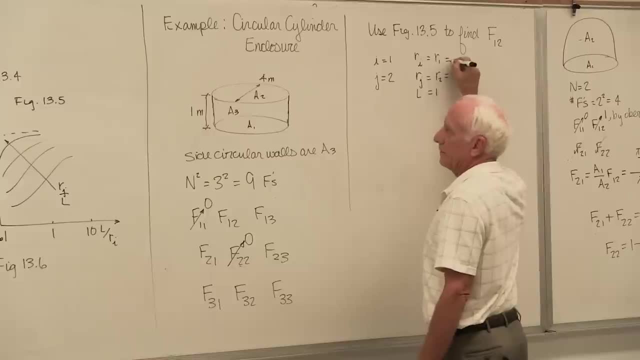 far. this is very far the liter like percent, with a lot of factor, and that's why it was so important. I've spent too much time classifying and they're danny click and that's why I was typing. I do 15 hundred centimeters and that's the. 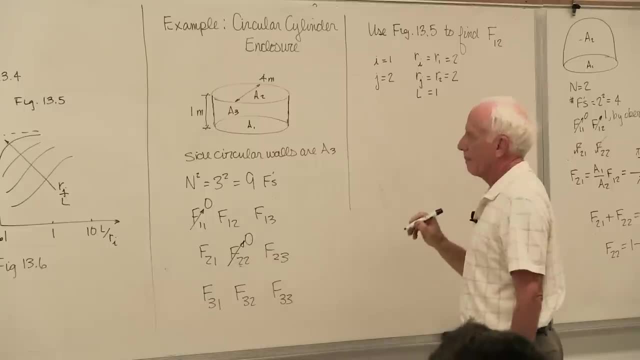 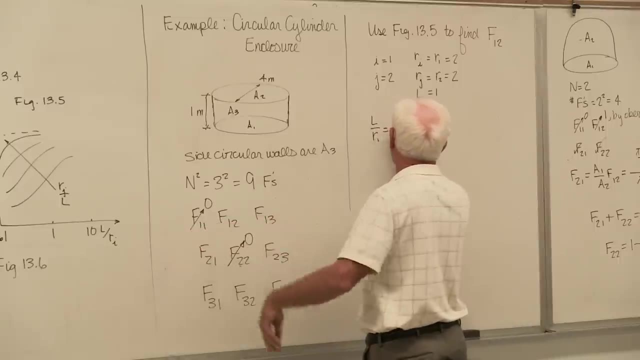 2 for each one. Okay, find the x-axis: L over R1.. Find the parametric variable Rj over L, R2 over L. Go to the graph x-axis. Well, first of all, get rid of a lot of these lines. 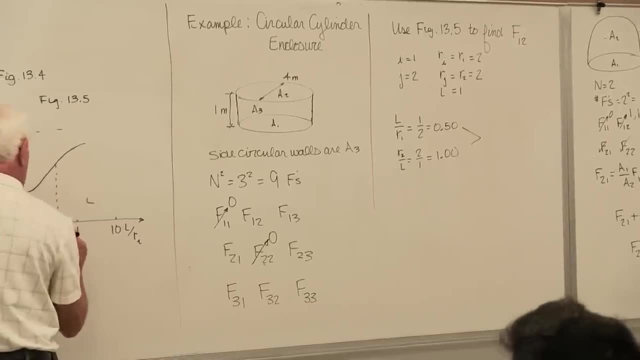 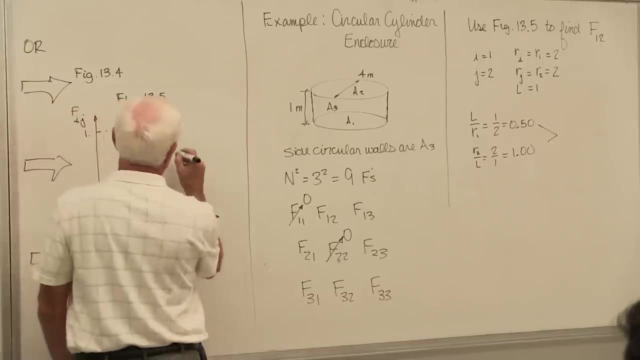 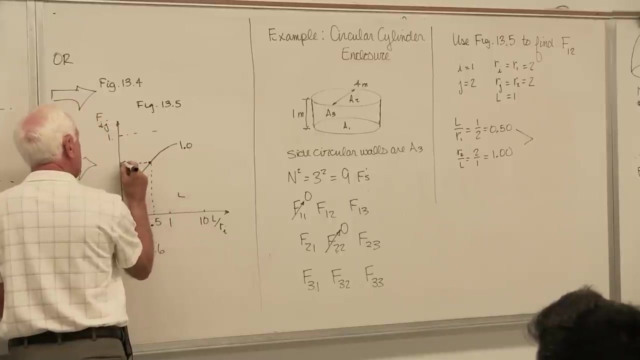 Go to 0.5 on the x-axis. Go to the line or interpolate, if you have to- You might have to- To find the line labeled 1.. Go across horizontally and get the estimate of the view factor 0.62.. 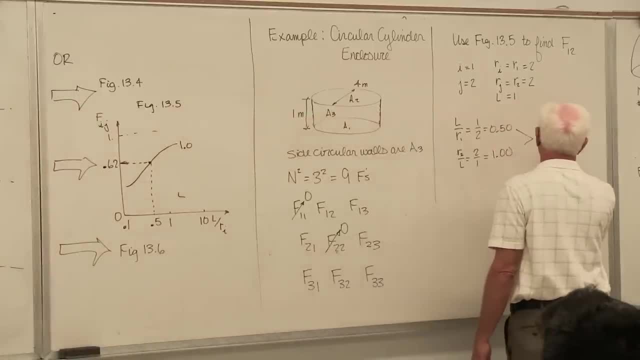 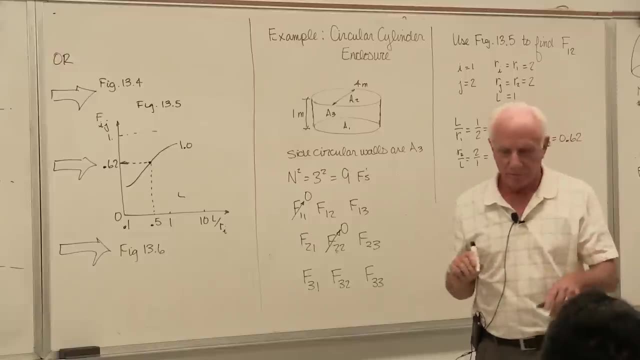 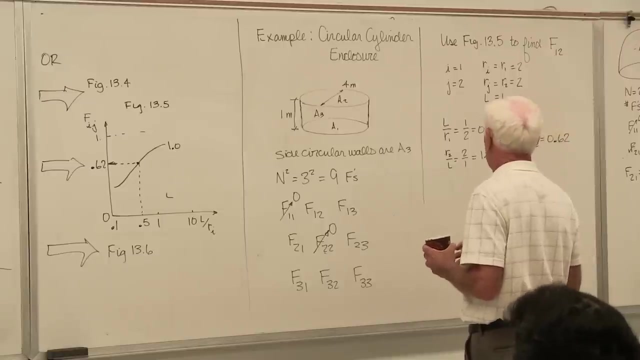 So F12: 0.62.. Oh, R2,. what is R2?? 2, and what's L1?? Yeah, R2.. R2, dimers: 4.. R4, raises 2.. Did I miss? 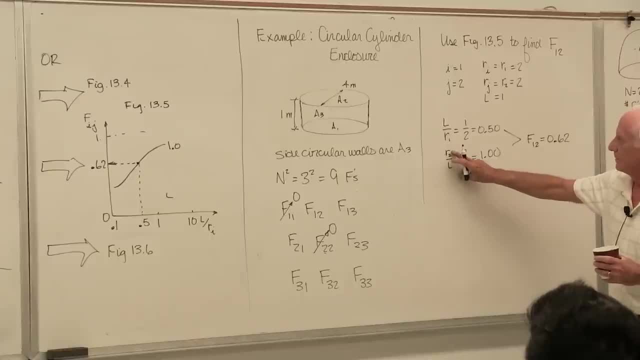 Oh no, R2.. L is 1, L is 1, R1, R2.. Oh no, Yeah, thanks, That's the new math, okay, Thanks, yeah, Okay, it's easy to do on the board. 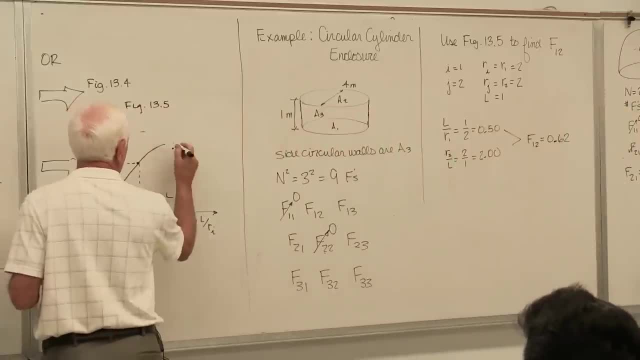 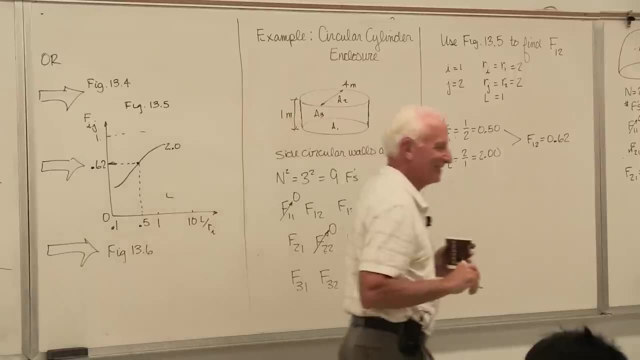 I got this magic finger that just does that. If you used ink on your notes, you're in trouble, I guess, but that's okay. The answer is still 0.62.. Thanks, though, I appreciate that. Okay, so what's the difference now? 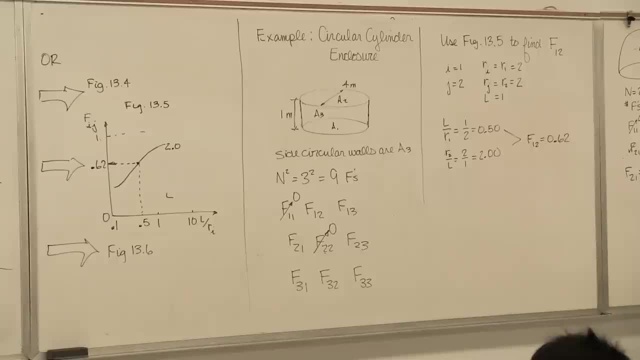 We couldn't use by observation. We had to use the tables 13.1 or 13.2, or the figures. Don't forget now two-dimensional. Two-dimensional means we've had a piece of paper, we've had it before for conduction. 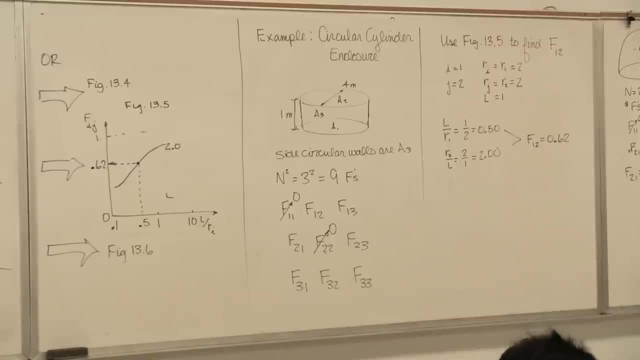 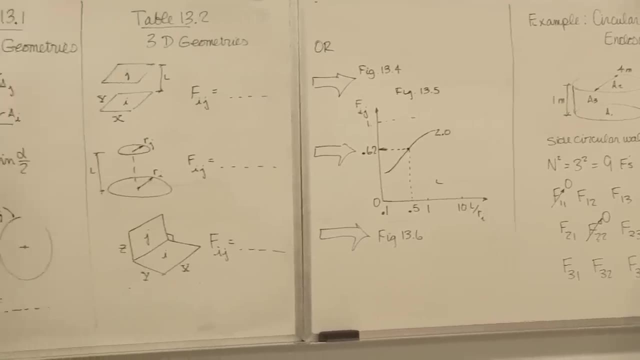 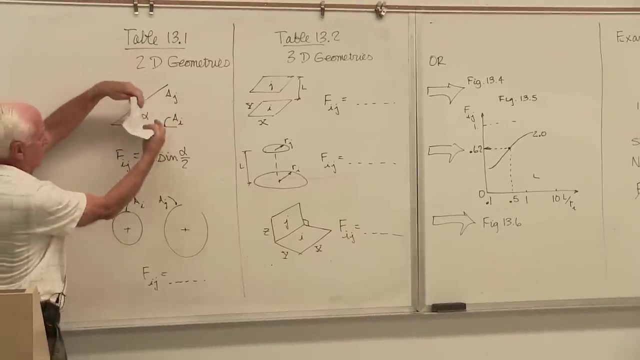 but just to remind you, Here it is, The bottom surface here is A1,, the top surface here is A2, and the angle between them is alpha. The sides are W, W here, W here. How long is it? The answer is: I don't know. 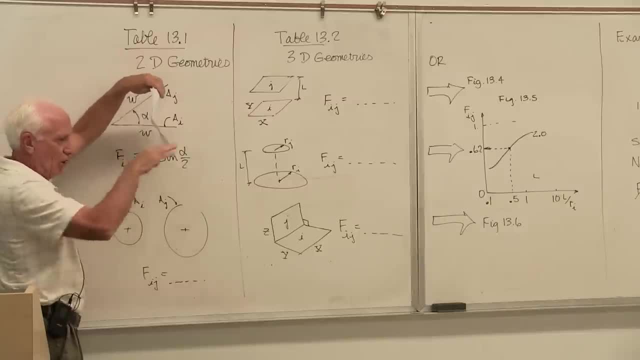 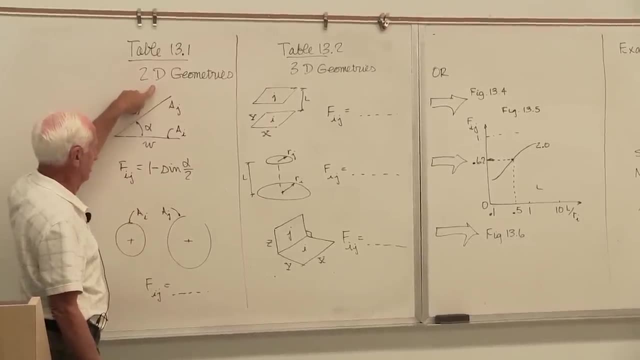 It's long, though It's long compared to W, It's long. If it's long, you can say, oh, it's a 2-D geometry, but you've got to say the word long. okay, Here's two pipes carrying a hot fluid to cold fluid. 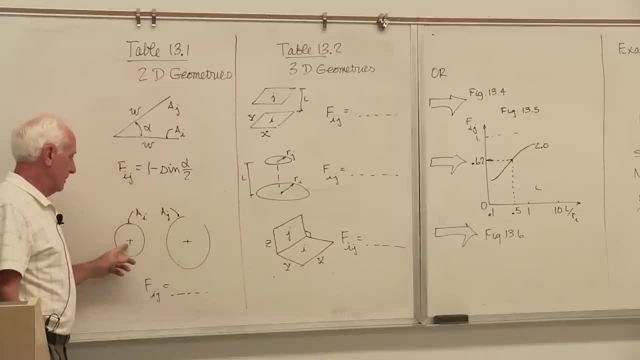 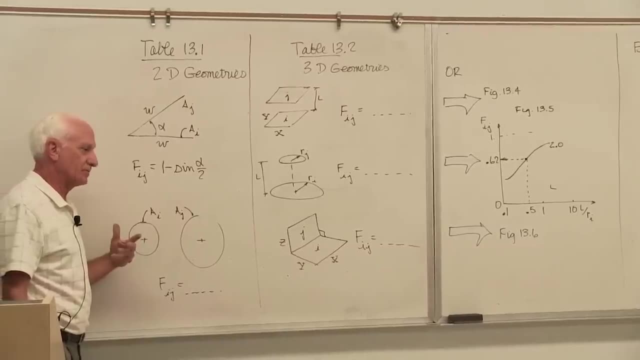 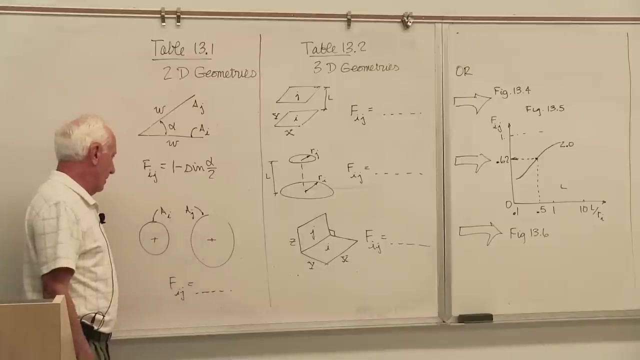 in a plant hung from the ceiling and I want to find radiation from one to the other or maybe outside the space station Pipes carrying fluids, maybe for a solar thermal plant. It's a vacuum out there. I want the radiation exchange hot to cold. 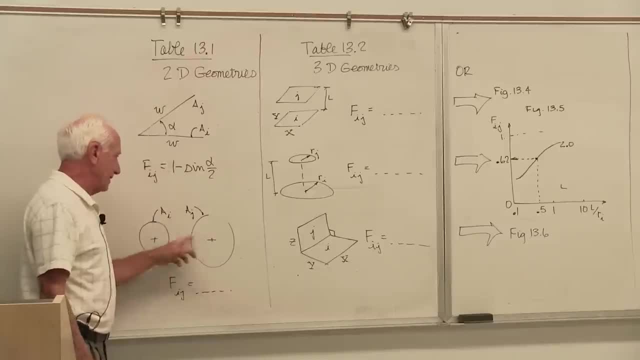 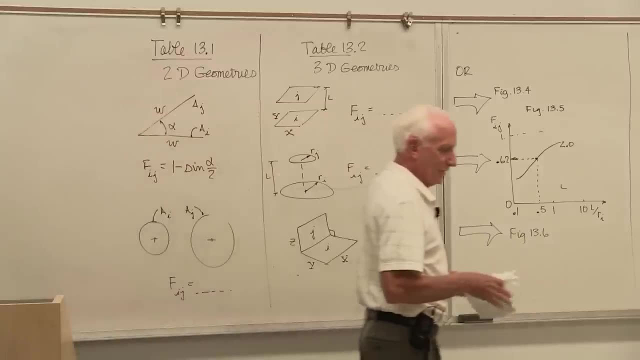 Here's a 2-D that works fine, as long as these these cylinders' diameters are small compared to the length of them. So that's what 2-D means, as we know from the conduction chapters. Okay, back to here. 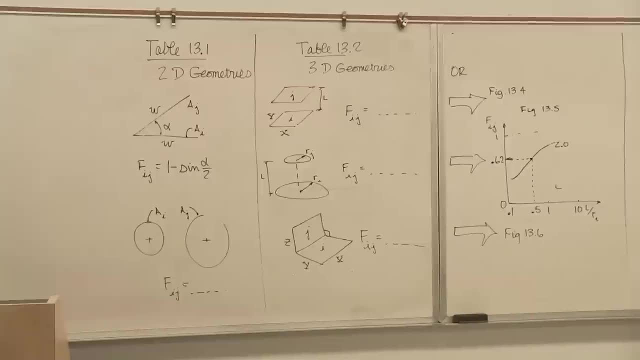 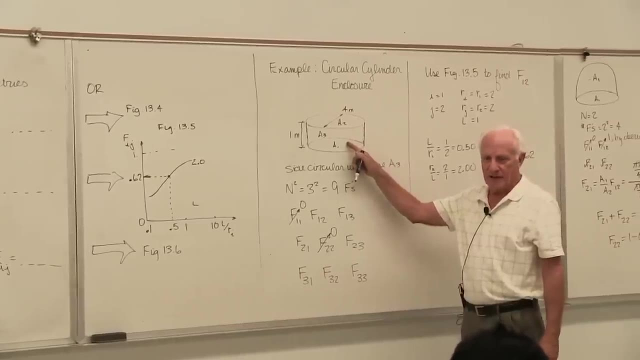 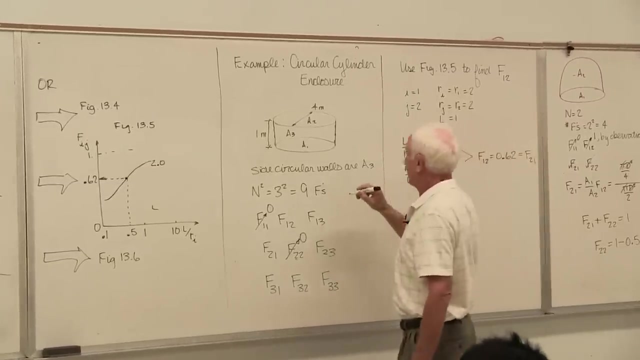 You know what I think? F12 is the same as F21.. Turn the coffee can upside down, Does it matter? No, Oh, okay, That's also F21.. Put a checkmark by them. I've got F12,, I've got F21. 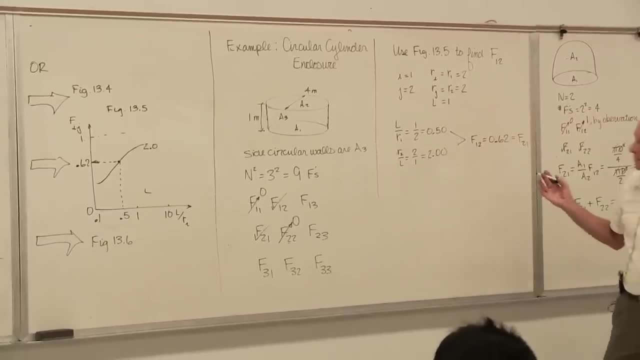 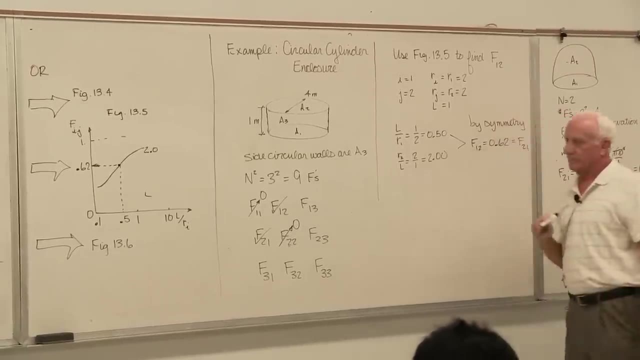 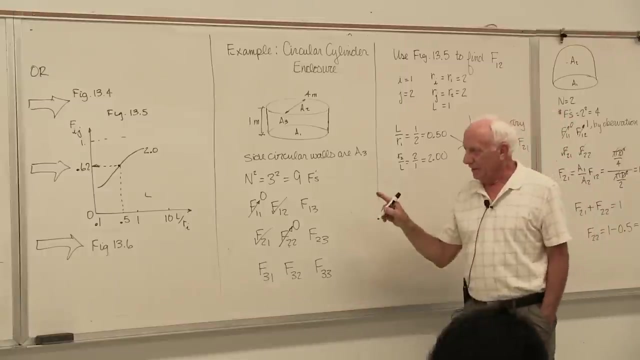 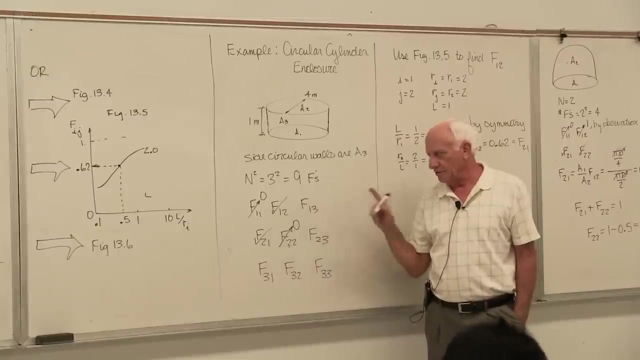 Good. Why is that? I don't know. call it symmetry. I told you kind of the rule: If you see any row, every row is the, you know, in the in the bottom left corner, the Earth enclosure law. If you see any row where there's only one unknown, you can solve directly for. 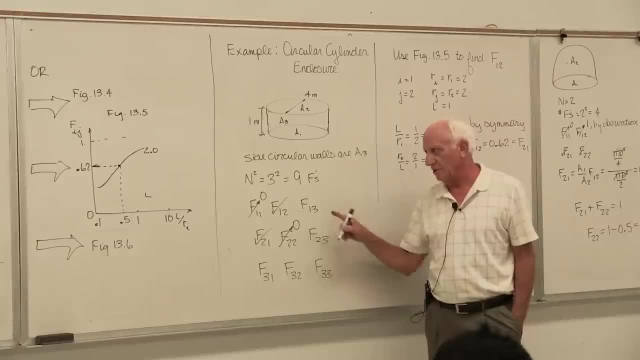 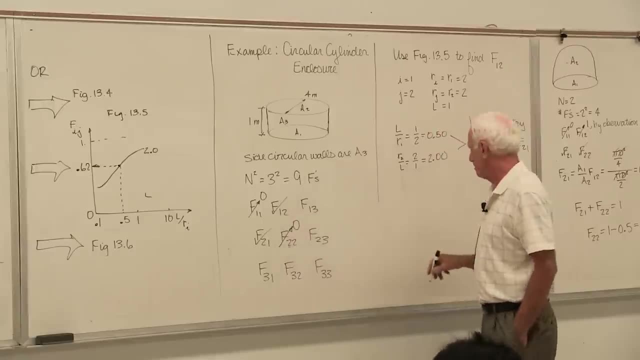 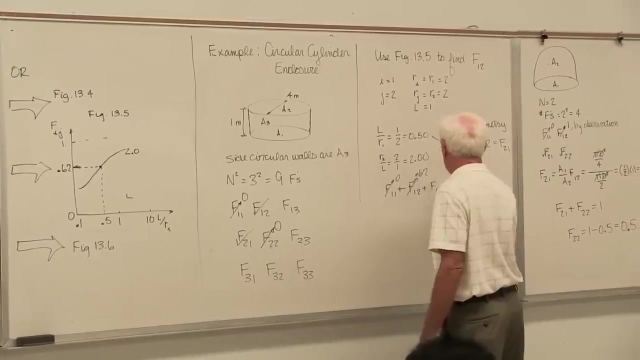 that unknown. That's why it's good to put it in this format, like this: Oh yeah, F1, 1, 0.. F1, 2.62 plus F1, 3 equal 1.. So F1, 3.. This guy 0.. This guy .62.. So F1, 3 must. 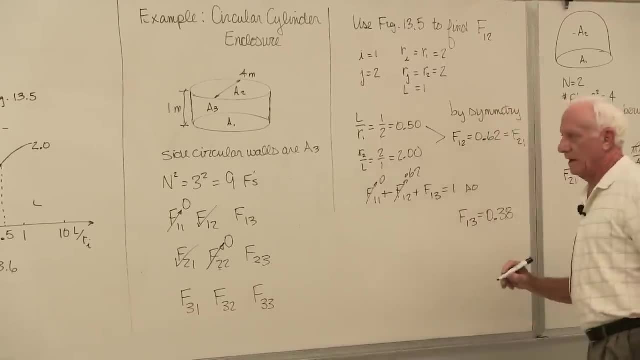 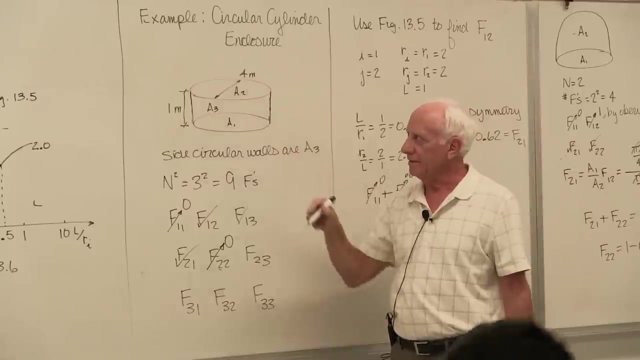 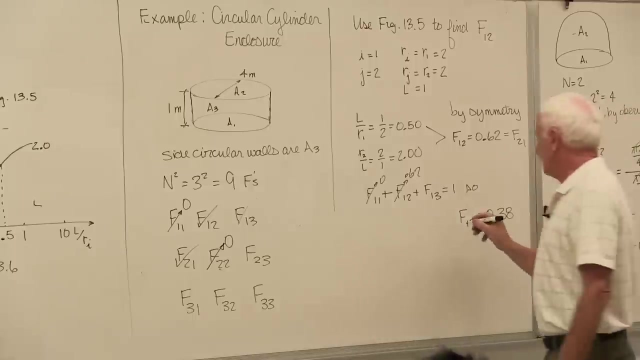 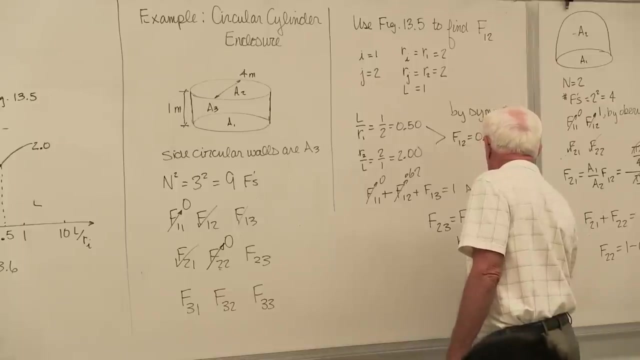 equal 0.38.. Got it F1, 3.. You know, if that's F1, 3, I think that's the same thing as F2, 3.. Why shouldn't it be? Why That's symmetrical. Got it: F1, 3 equal F2, 3.. 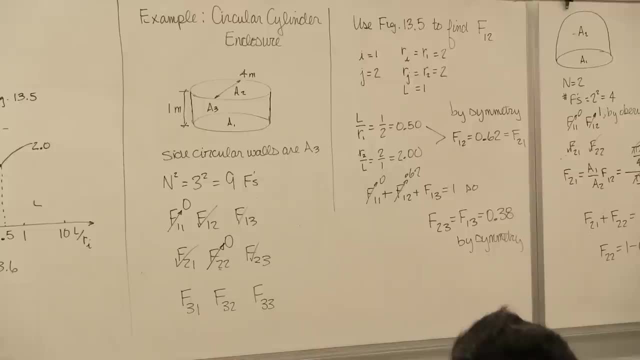 Got it. I've got six of the nine. now I've got six of the nine Over here. Gee, I don't know any of these guys here, But oh yes, I do. F31,, F13, reciprocity. 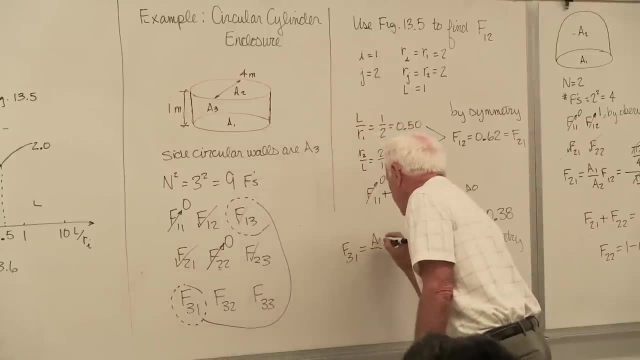 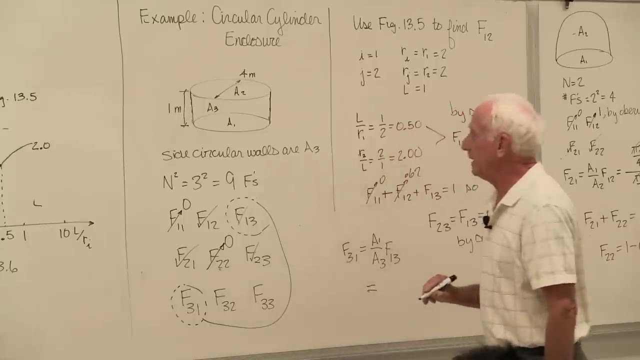 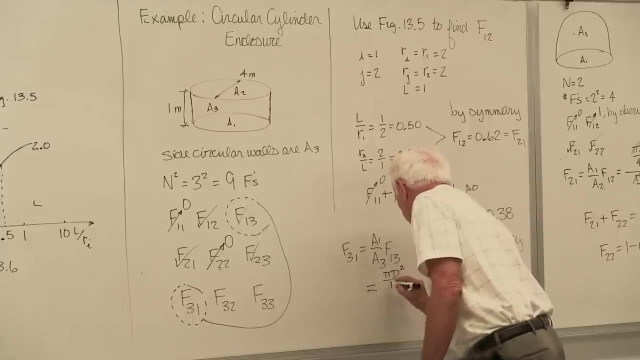 F31 equal A1 over A3, F13.. Okay, A1, pi D squared over 4.. Pi D squared over 4.. Divided by A3, pi D times L, L is the spacing. L equal one meter. 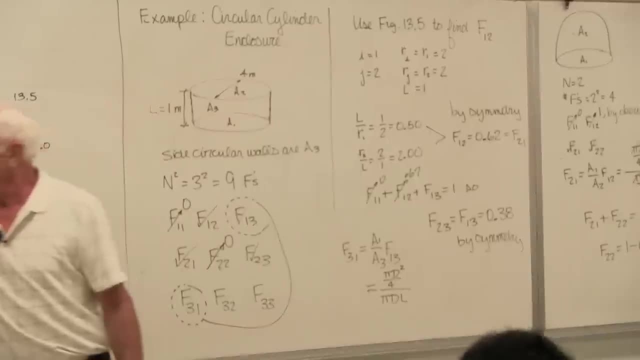 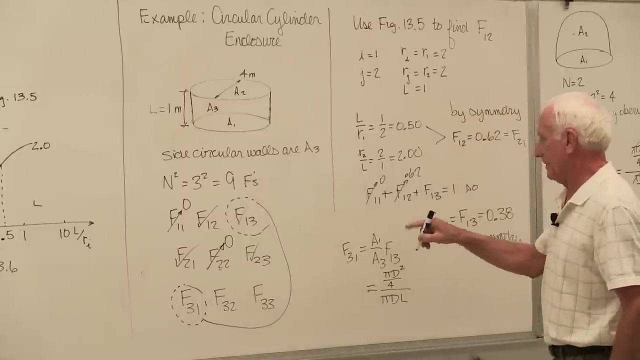 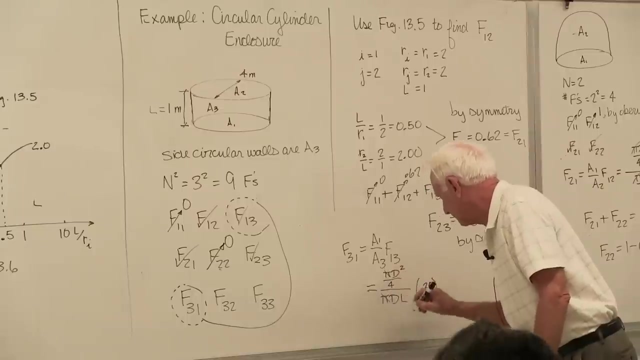 Like the picture in the textbook shows. L is the spacing from the two parallel disks Times F13.. I just found F13. It's .38.. Pi cancels, Pi cancels. We have 4DD. We have D over 4L. 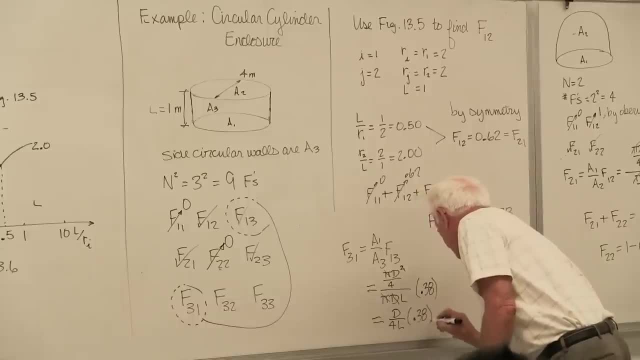 What's D: 4. What's L: 1. 4 divided by 4 times 1.. 4 divided by 4 times 1 is 1.. .38.. I got F31.. Then I say to myself: gosh, you know what? 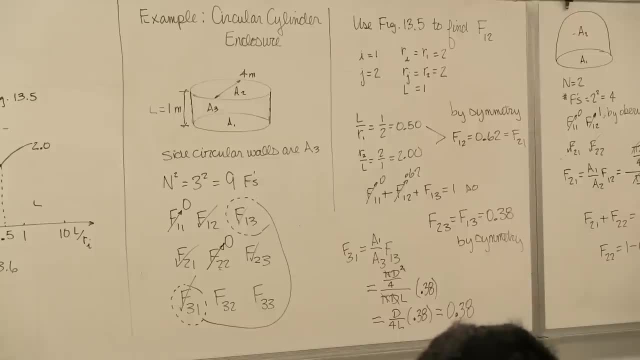 I really think F31 is a stupid thing. It's the same as F32.. Say: how do you know that? Say it's symmetrical. You got it. This is F32.. All right, I got F31, F32.. 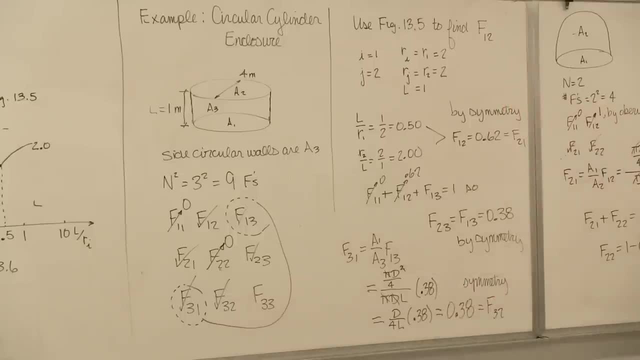 Here's the rule on any row: when you put them in that format, If you don't know one F in a row, you say F is enclosure law. F31 plus F32 plus F33 is 1.. F31 plus F32 plus F33 is 1.. 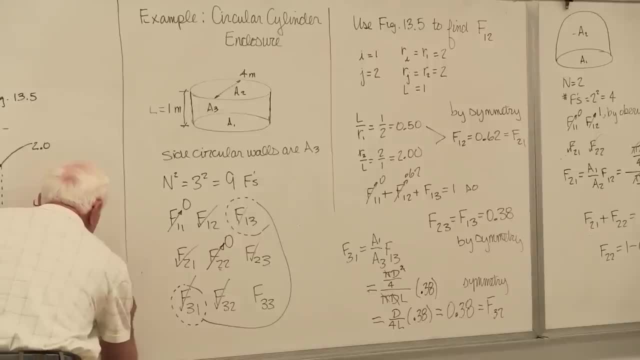 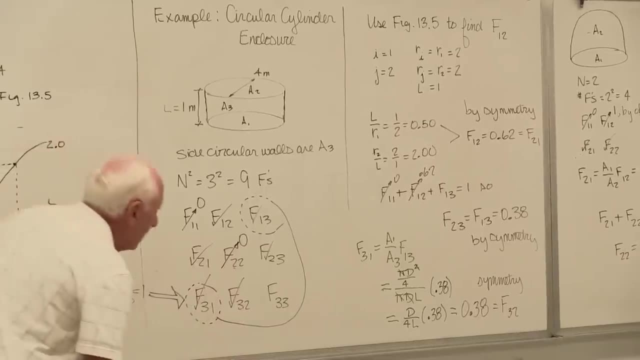 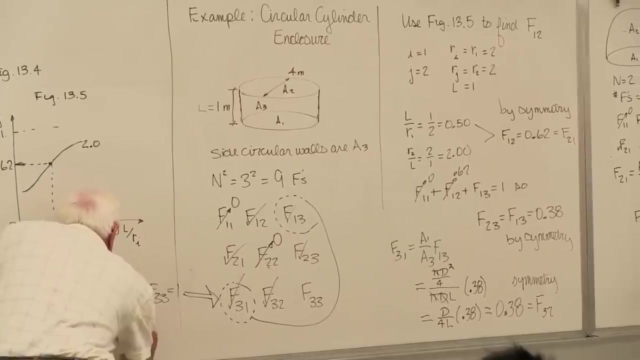 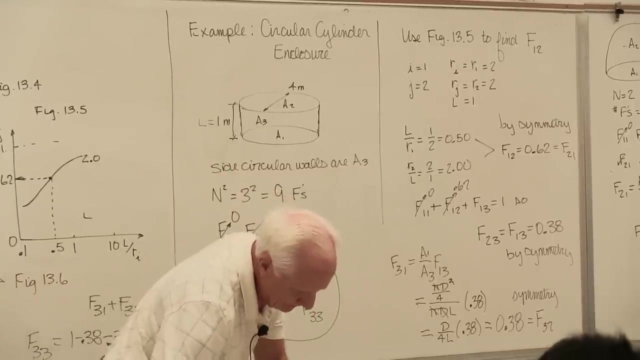 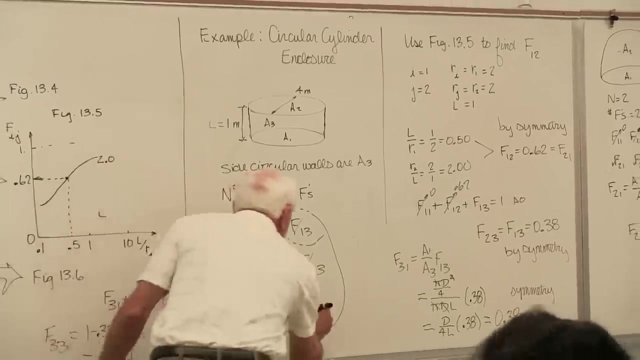 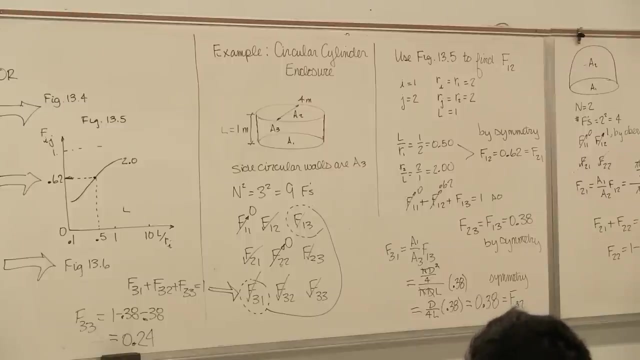 F31 plus F32 plus F33 equal 1, from there F31.38 minus .38, F33. F33.24. .34. .34. .34. .34. .34. .34.. Got it? I found all nine. Okay, that's how you play the game. You try to see if you can. 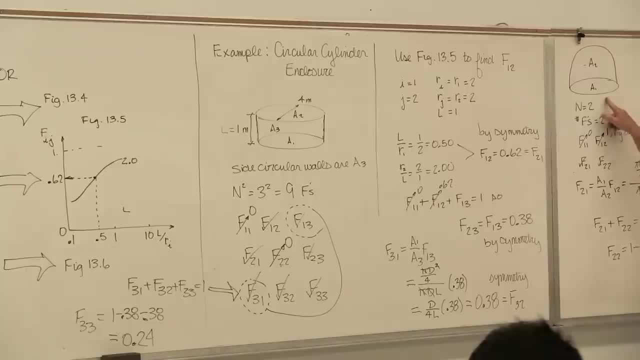 see things directly by observation. If you can't, you try and find either a table or a figure to find that first one that you need, And once you find that one, generally things start to fall out. Once I find F12, bam, bam, bam, bam and I got everything right from. 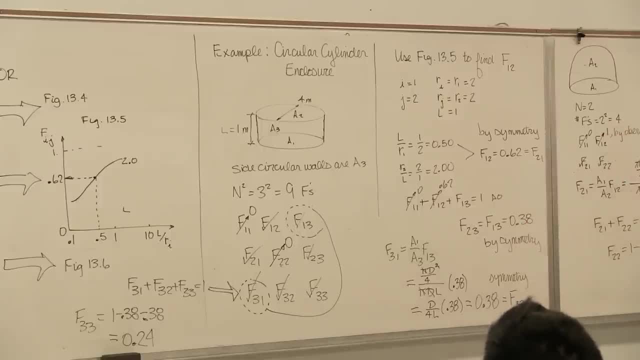 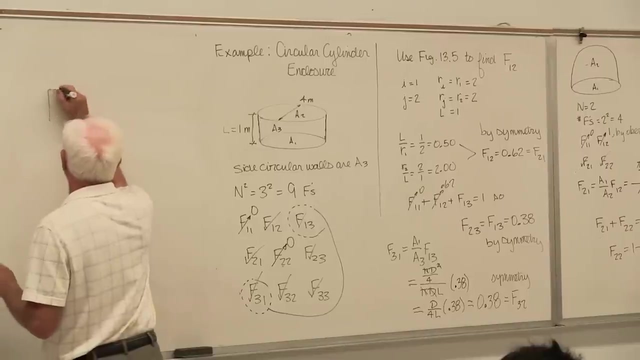 there. It's all I needed. Okay, that's called view factor algebra. View factor, algebra. I'll do one more, because this is the one that confuses people. I'm going to take this bottom one down here and I'm going to take an enclosure which is a rectangular wall room, and I'm 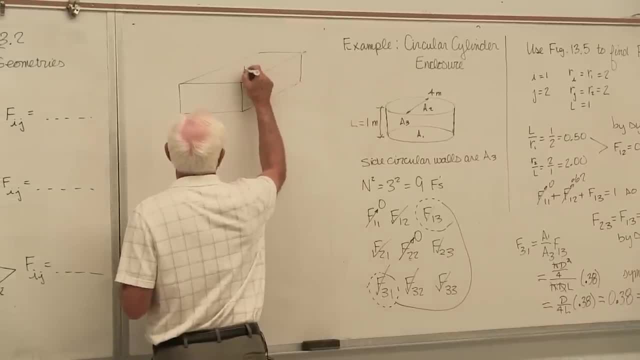 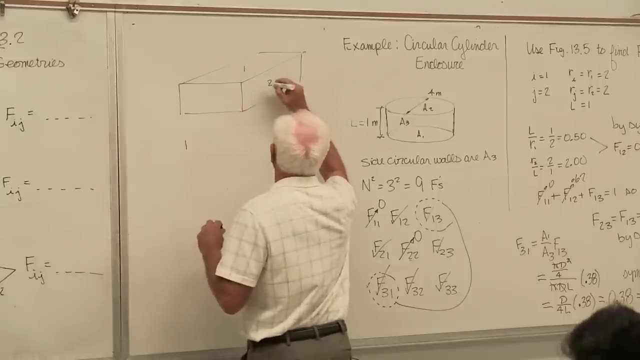 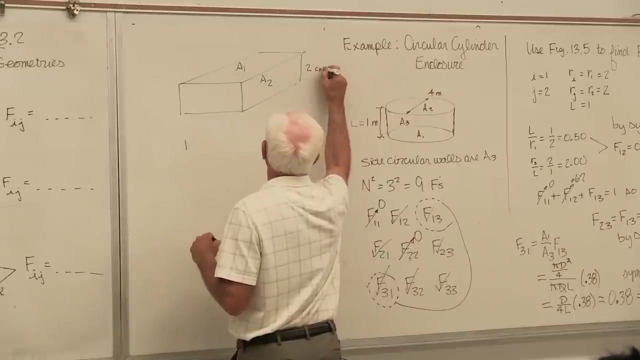 going to call this area one and this area two And I want to- okay, I'll put some dimensions in here- I'll call that two centimeters, three centimeters and five centimeters And I want to find F12.. 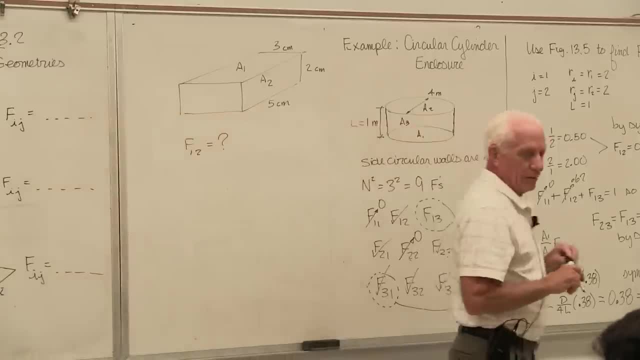 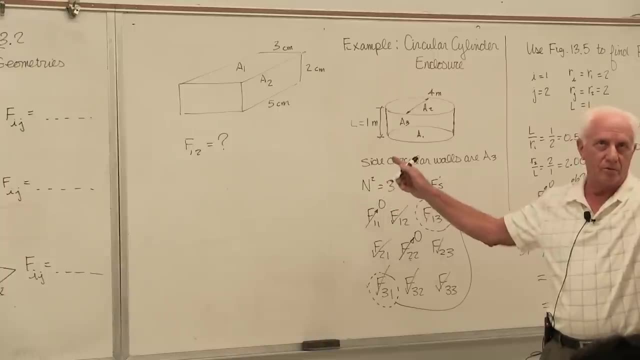 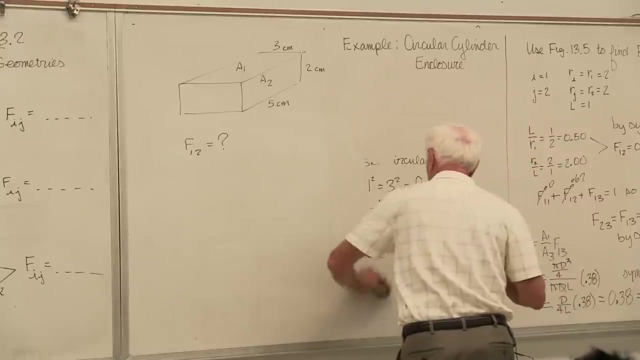 Okay, it's like the ceiling would be A1 and the front wall is A2, just so you kind of know what it looks like. This is a rectangular shoebox. this room is. Ceiling is A1, front wall is A2.. To do this right, and here let's draw the graph, Okay, so here's the graph. 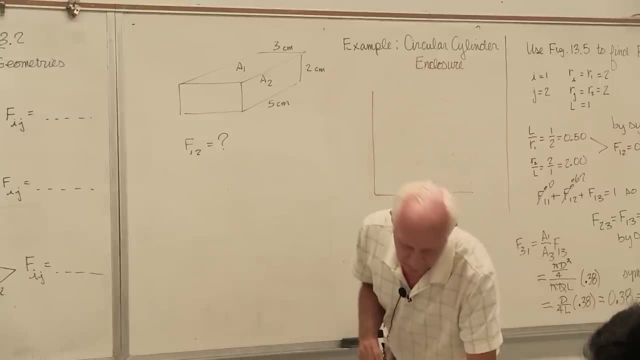 And we've got. okay. I'm going to draw the picture first. on the graph It looks like this: Right angle, I and J, X, Y, Z, And here's FiJ Okeex. I'm going to draw, I'm going to. 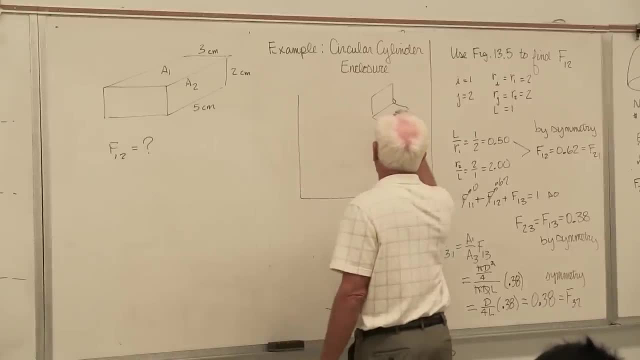 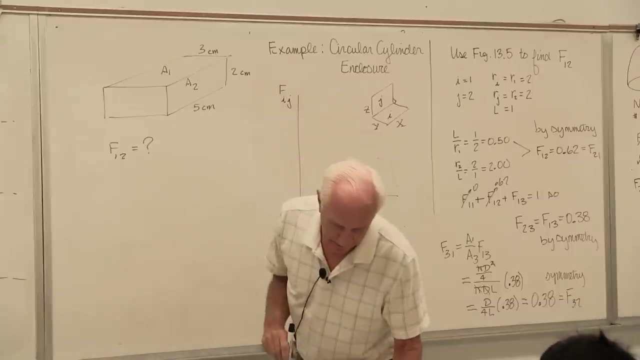 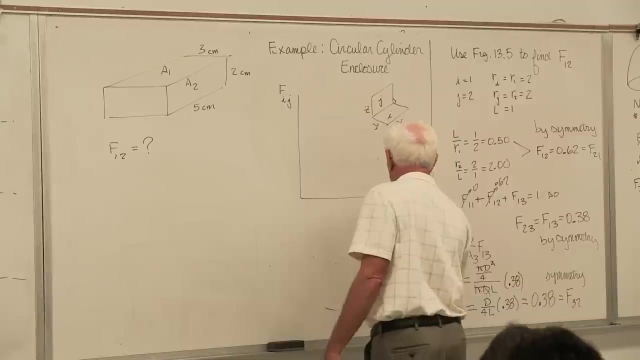 draw the picture first. on the graph It looks like this: Right angle, I and J, X, Y, Z, And here's FiJ, And the x-axis is z over capital X And the parametric curves are y over x. 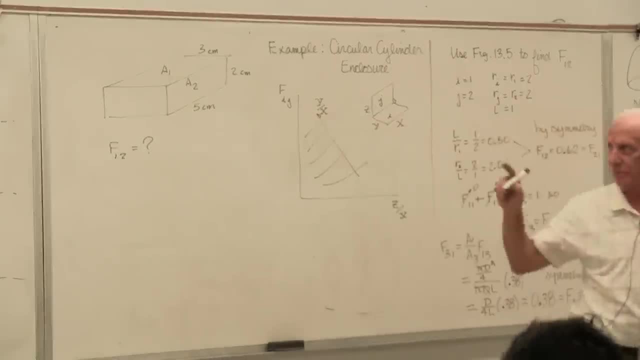 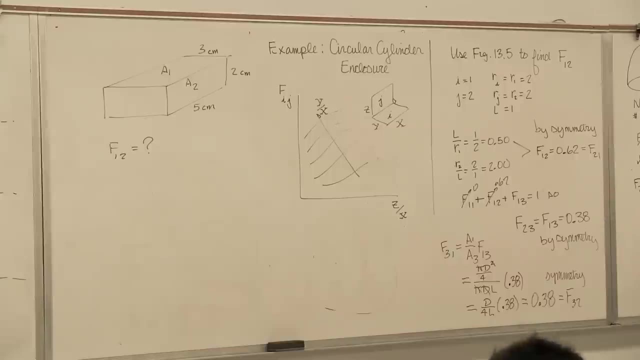 And, of course, in your data package for the course you have table 13-1,, table 13-2, all three of those figures- 4,, 5, and 6,, 13,, 4,, 5, and 6.. 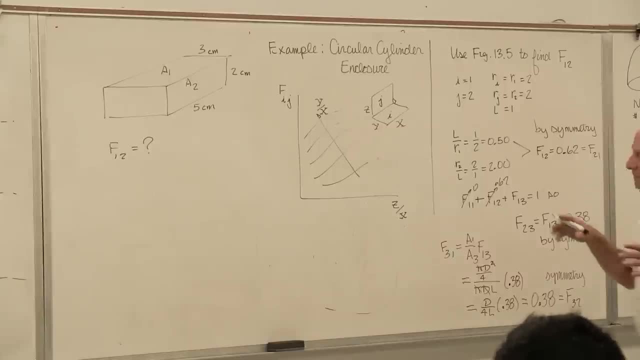 You have all that on your data package, Okay, so here it is, F1-2.. Sometimes this kind of gets people all messed up because 1 and 2 don't look like I and J over here. So you don't want to make a silly mistake on exam or homework. 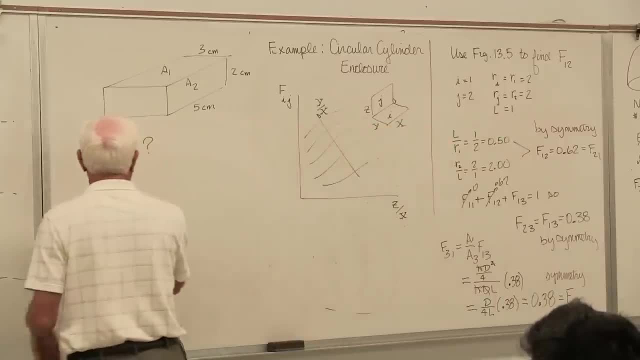 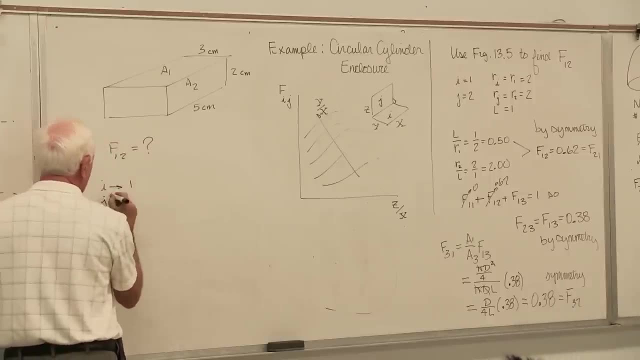 So the first thing you do, you say okay, what do I want to call I? Okay, obviously I is the first subscript 1.. What is J? Okay. next thing: J, second subscript 2.. Here comes the tough part. 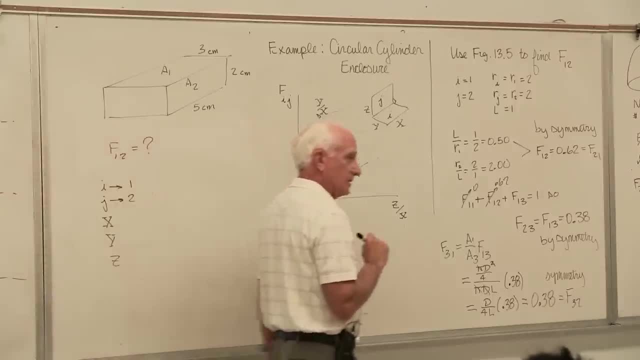 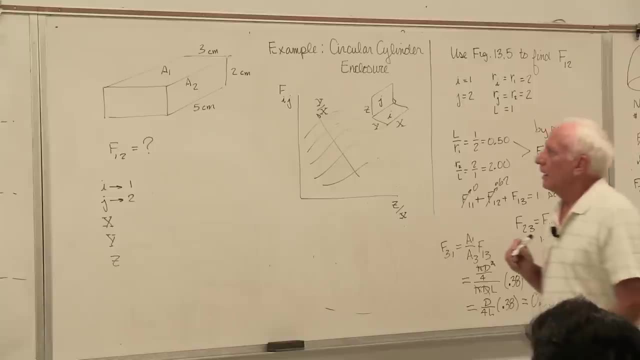 This is the one where people generally make their mistakes with X, Y and Z, And of course, it's going to give you an error in F, in F1-2 when you do that. Okay, identify A I Here, that's A I. 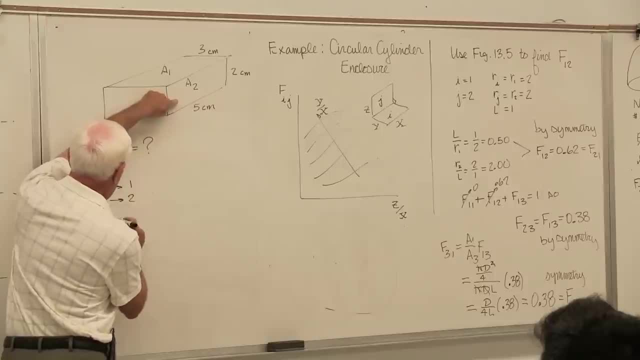 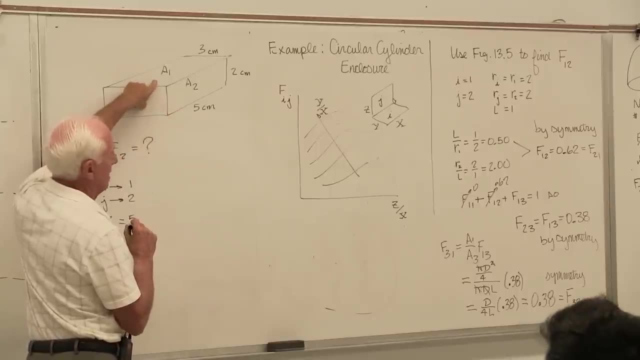 There's A. There's A J. What's the common edge? X, Common edge. 5. For A I: what's the direction from the common edge? away from there? 3. For J: what's the distance away from the common edge? 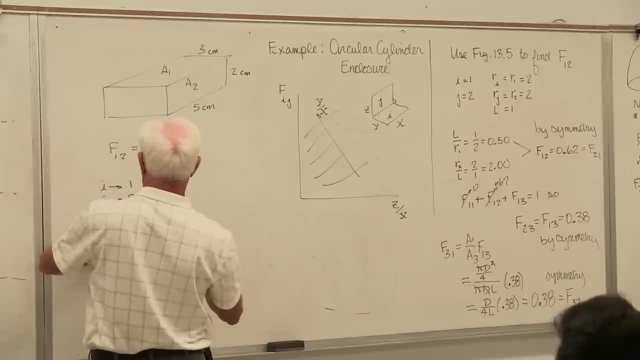 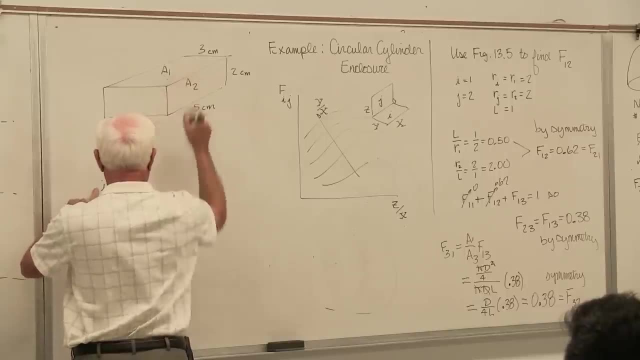 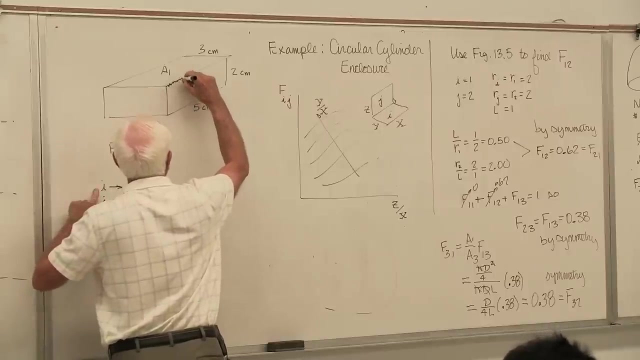 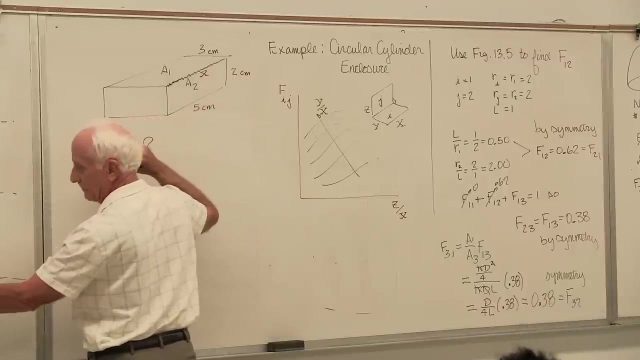 Right, that is the Y is our yeah Y goes with I, And I is this, that's 3.. And J is 2.. Yeah, There's the common edge right there, That's X. The distance away from the common edge for surface. I is Y.